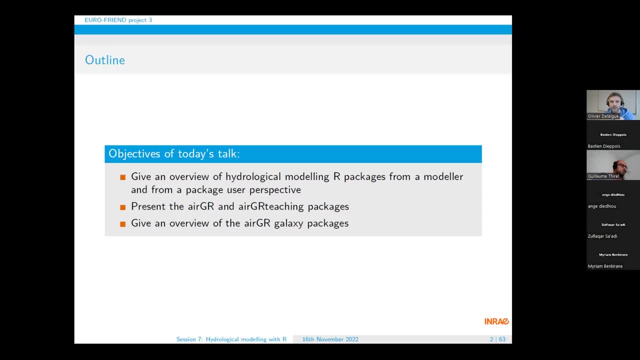 Then we will present two packages, RGR and RGR-Teaching, which we developed And which propose the geohydrological models. And finally we'll give an overview of other packages that are around this RGR package to open new possibilities of modeling. 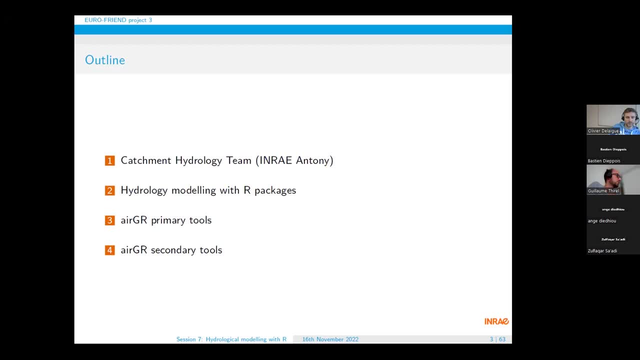 So the outline of the talk is this one. So first I will present our team in a few words, Then I will present a work on the R packages that are available in R And we will present the data of our hydrological modeling based on the paper. 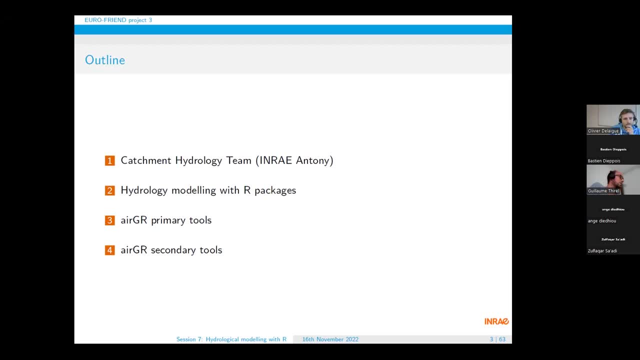 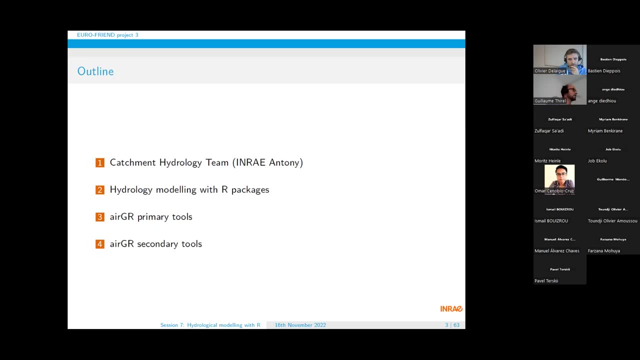 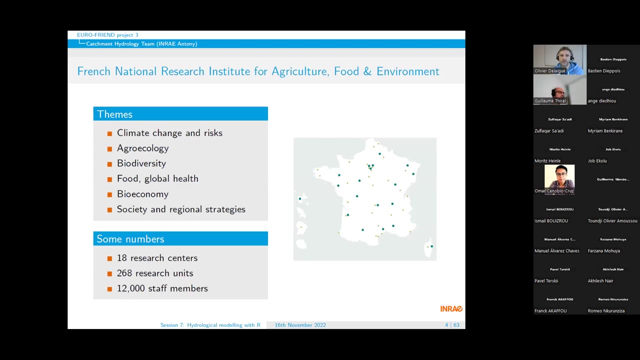 And Olivier will present the RGR main tools And finally, I will finish with the RGR galaxy. So our team, So we are a research center called INRAE, which stands for French National Research Institute for Agriculture, Food and Environment. 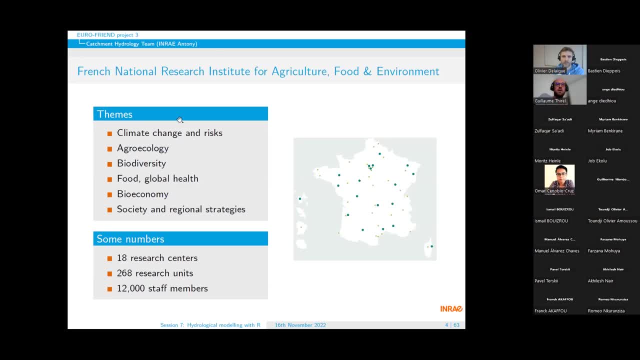 And we are based in Antony, So Antony is very close to Paris And INRAE is very large, So it's 12,000 people, many research units, and we are all around France And so the topics of this institute are very large. 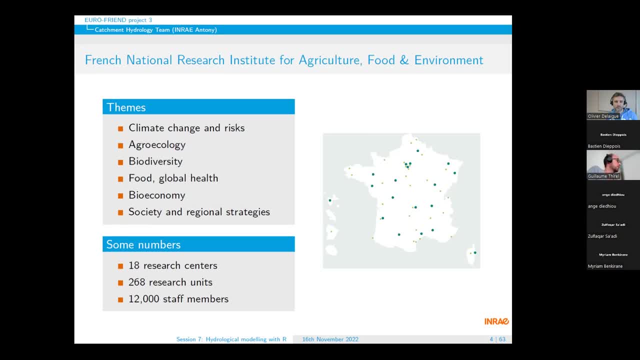 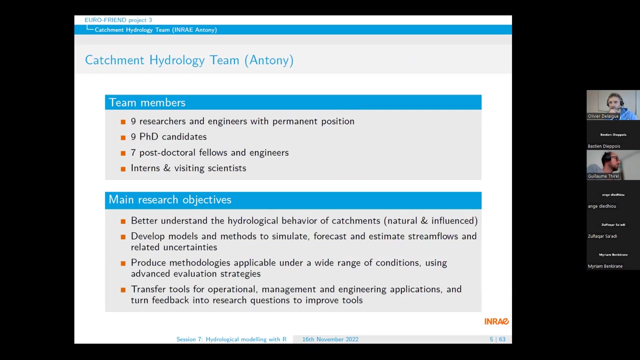 Climate change and risks, which are the ones we are focused on: Agroecology, biodiversity, food, health, Bioeconomy and everything around society and regional strategies. Regarding our team, the next slide: Yeah, thank you. So we are nine, researchers or engineers, functionaries. 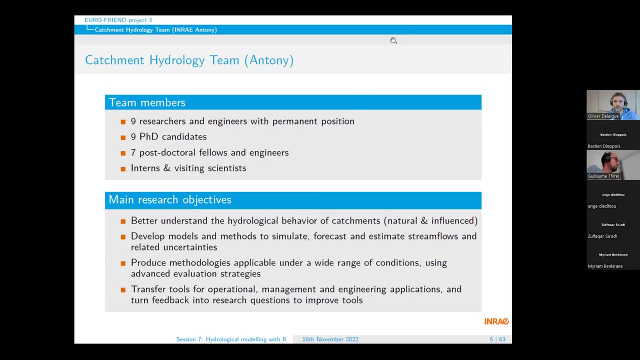 We have a lot of PhD candidates, postdocs, fellows, engineers and interns or visiting scientists And our research objectives. Research objectives are around hydrological modeling. So first to understand the behavior catchments, both for natural conditions, which is what we have done on a historical point of view in our team. 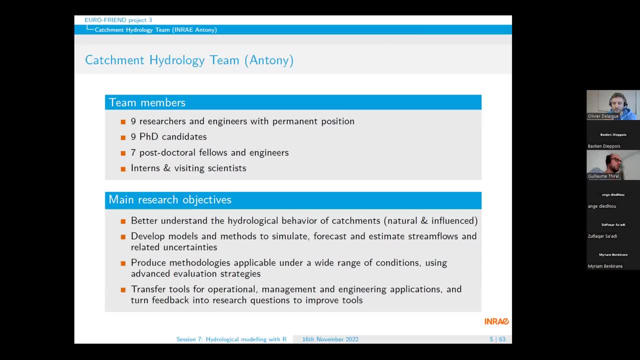 But also we are looking more on influenced hydrology. We try to develop models and methods for forecasting, for simulating stream flows, And we have a lot of works around uncertainties. We also have something which is very linked to Nance Adel's talk last month about large sample hydrology. 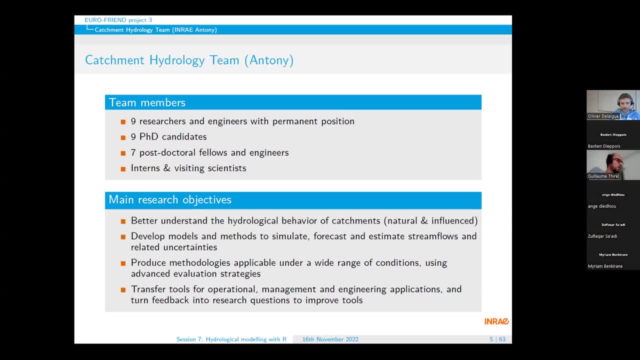 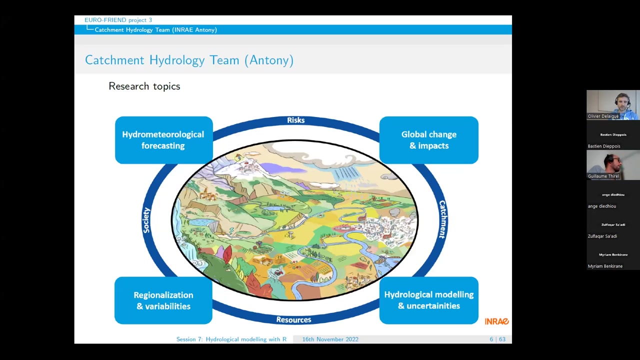 Meaning that we have methodologies on many, many catchments in order to have something that works on a very wide range of conditions. And finally, we do our research for operational Applications And it's also used for management, for engineering, Which means that we try to turn feedback into research questions to improve our tools. 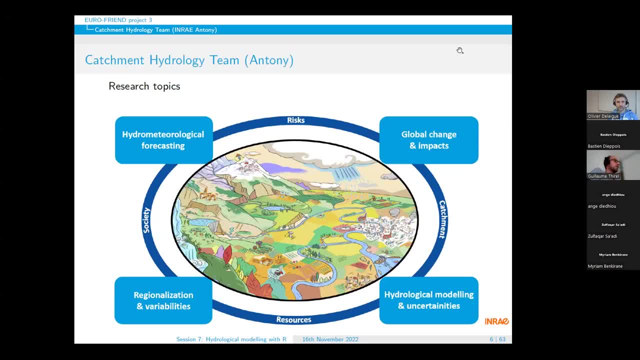 So, to summarize, our research topics are aggregated around the four topics Forecasting global change and impacts, generalizations and variabilities, And I don't just talk about that, But I talk about a lot of things. So I'm going to start with hydrological modeling and uncertainties, with some keywords like risk, society, resources and catchment. 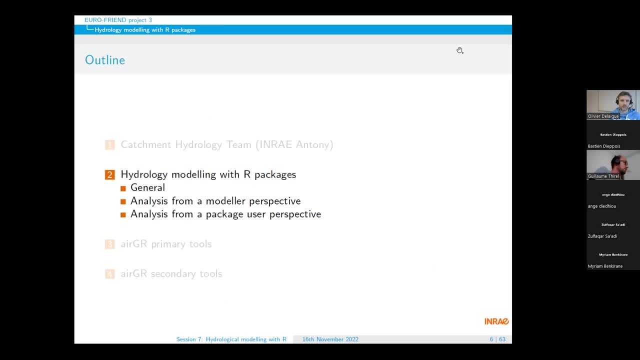 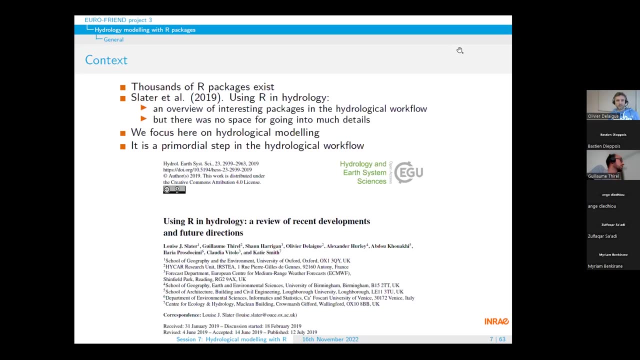 Okay, so now I'm going to start with the first scientific thing about hydrological modeling with R packages. Yeah, so this is actually. the rationale around this presentation is that we have many, many R packages, Like thousands of R packages, available in the official repository. 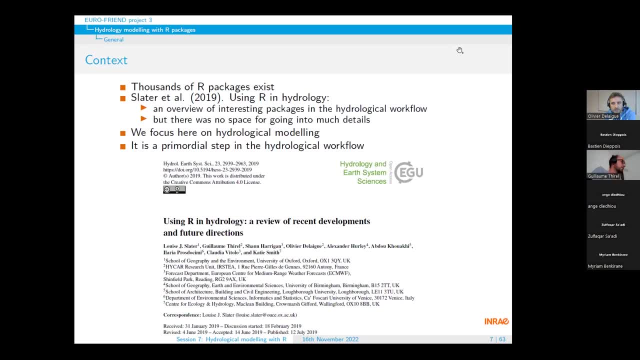 In 2019,, with Louis Slater and colleagues, we made a paper in HESS, which we have in this slide, In which we tried to assess what is available in R for doing hydrology. So it relies on workshops we have done at EGU for years. 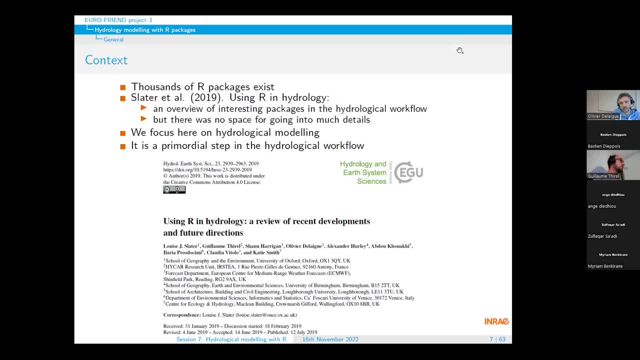 And we have a lot of work to do And we analyze the main packages that are available for the main steps of the hydrological workflow, Like applying data, retrieving data on archives, hydrological modeling and plots analysis and so on. But that's a lot of things. 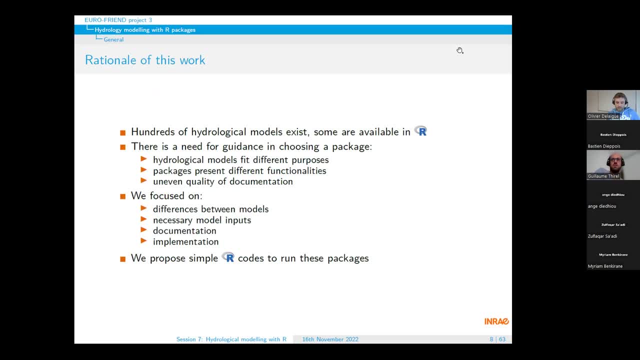 So we could not develop all the steps. That's why, after that work, we have done an additional work on hydrological modeling. So you all know that hundreds of models exist. There is a sentence saying that each modeler has its own hydrological model. 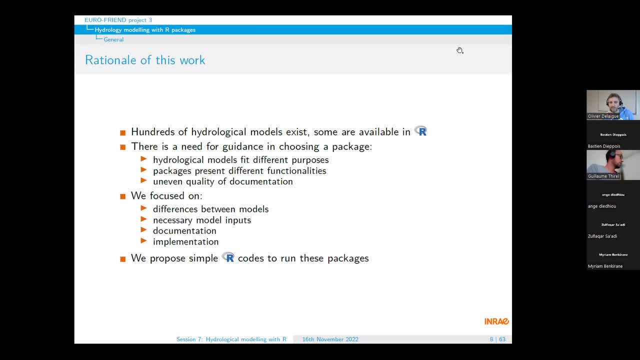 That's almost true, And despite of all these models existing, only some are available in R. But still we felt that there was a need for guidance in choosing a package Around this 10 to 20 packages available. First, because not all hydrological models fit all your specific topic. 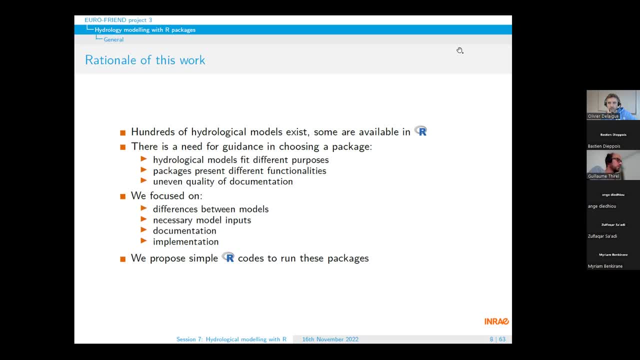 Also because the packages present very different functionalities And maybe the one you need is missing. And finally, we also knew that The The documentation was a very, very different between the packages, with some packages with very good documentation and some packages with no documentation at all. 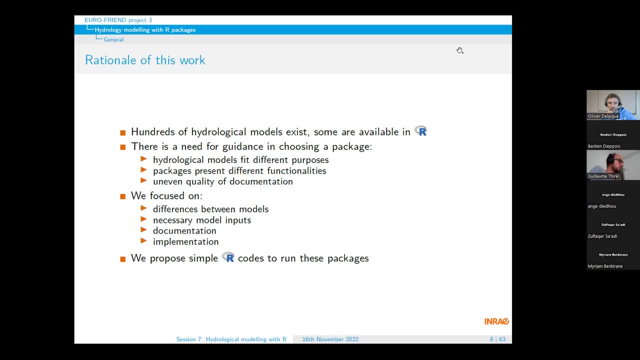 So in this work we focused on the differences between the models. We analyzed the different model inputs necessary, We analyzed the documentation and also how the packages were implemented, And We also proposed very simple R codes as additional supplementary material to run these packages. 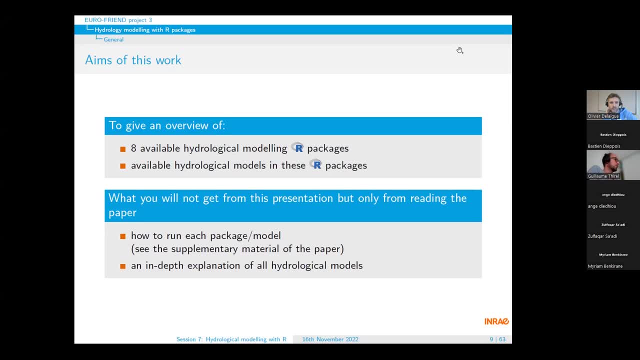 So in this work we will give an overview of the eight models- Sorry, in the eight packages that's proposed hydrological models And also we focus on the models that are available. But You will not get from this presentation How to run each single package or each single model. 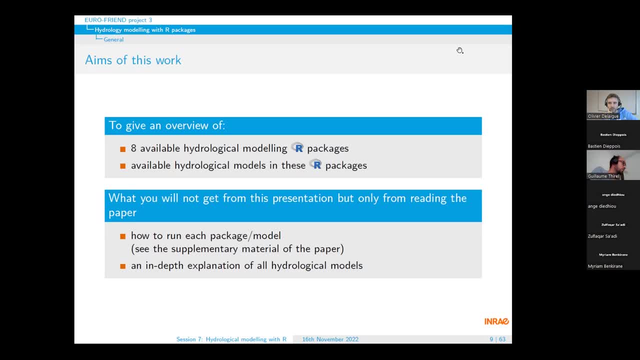 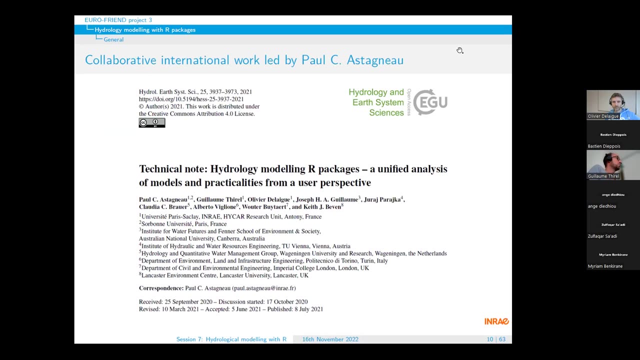 For this you have to check the Simple supplementary measure of the paper And also we will not have time to provide an in-depth explanation of all hydrological models. So this is a paper led by Paul C Staniel And for this work we worked. 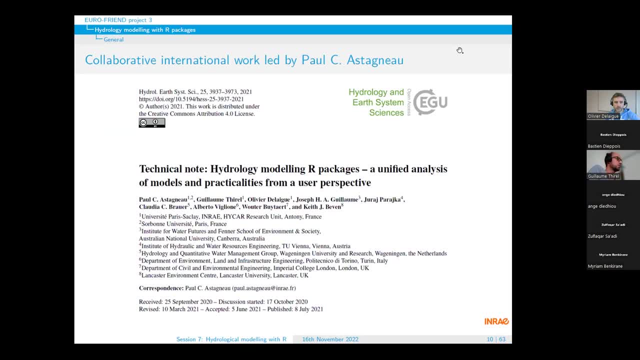 With an international team, Because we tried to To contact the developers of the different packages, to To have the best information about each package and each model, And so I invite you to To have a look, after the talk, at this paper. So here we'll focus on different things. 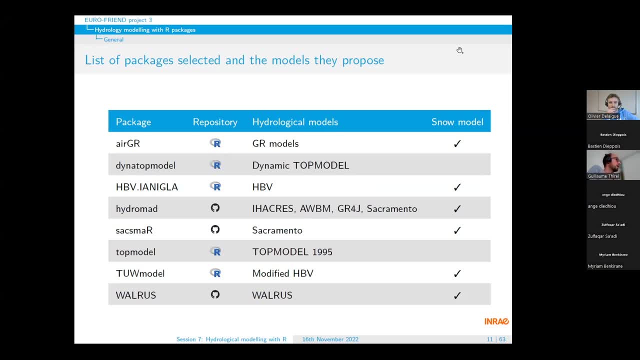 So here are the eight packages we analyzed. So Yeah, what we have in this table is the name of the package And also The models that are proposed in this In each package. So, for example, you can see that we have the GR models in two packages. 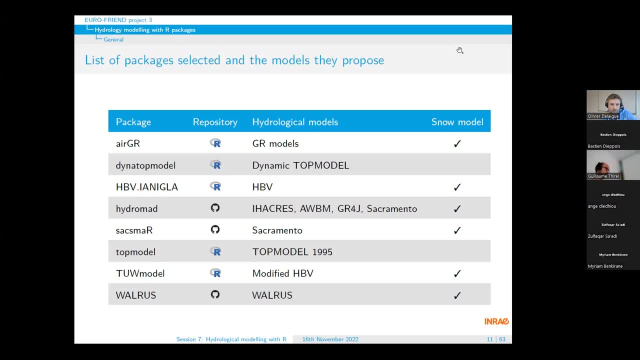 RTR and Hydromad. You have the top model package- Sorry, the top model model- In two packages: Top model and Dynatop model. Also, HPV is quite present In R In two packages HPV Yanigla. 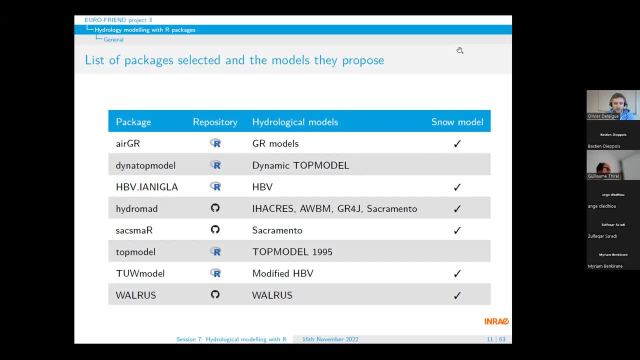 But also TUW model. And finally, you have some other Models: CyHackRest, AWBM, Sacramento, Where else? And We also- Yeah, We found these packages, But not only on the original, But not only on the official. 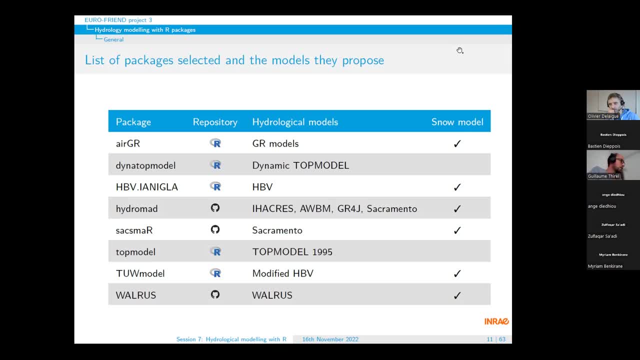 Repository, which is represented by the R symbol here. But we also found some packages which were only on GitHub And on the right column you can see that Not all packages propose no model, So that's a first way to decide which package to use. 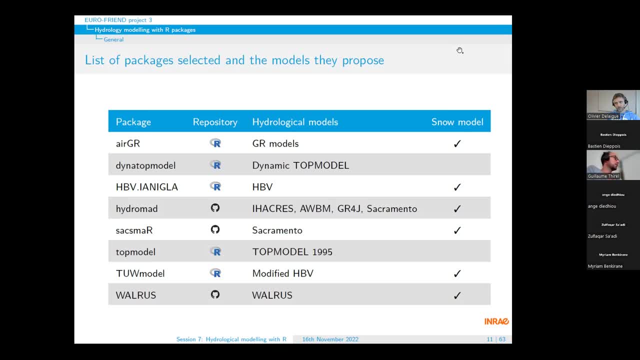 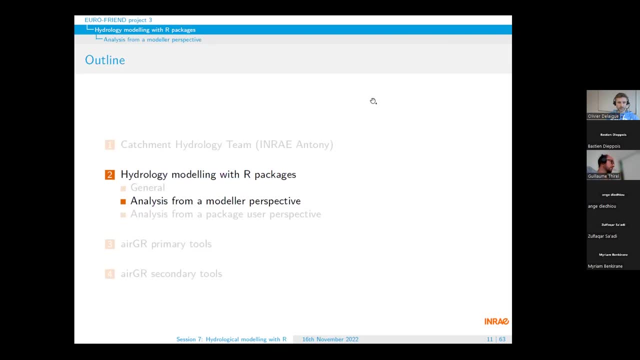 If you want to work on snowy basins, You can eliminate Two of the packages That are not Or not In the base, Yeah, So Let's start with a model Perspective analysis. So here, Yeah, You already have to. 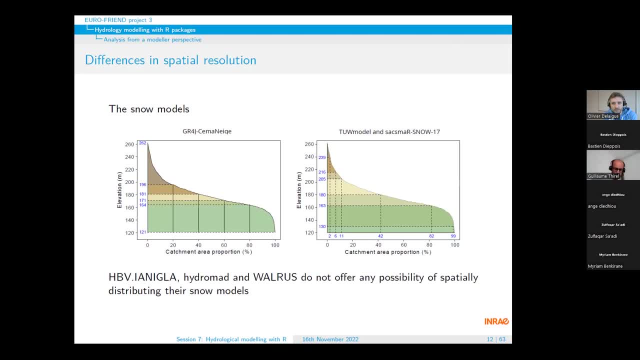 To To think as a model What you want to To represent in your basin. And The first thing that is abusive: If you have a snow in your basin, You need a snow mother So you Can take a look at it. 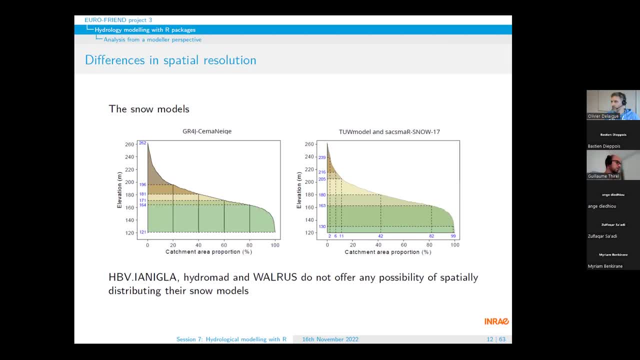 So This So, which means that you can eliminate two packages. but the second step of analysis on this is that snow models that are present in the packages can be very different, especially on the way the processes are presented. Some were on representing snow processes with the degree-day method. 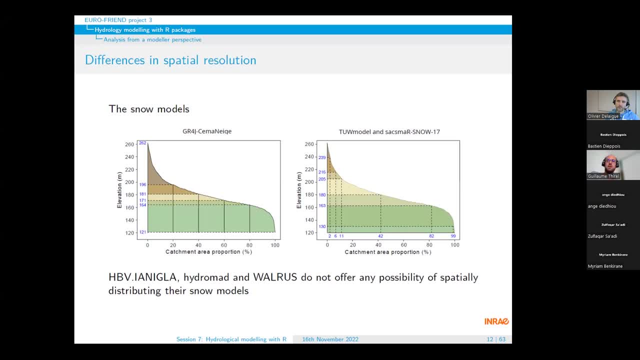 other ones were based on the energy balance method. And the second point that is very important is spatial resolution, because you all know that in mountainous areas there is a very strong orographic gradient on temperature and precipitation, And here we represent two ways of representing the heterogeneity on basins. 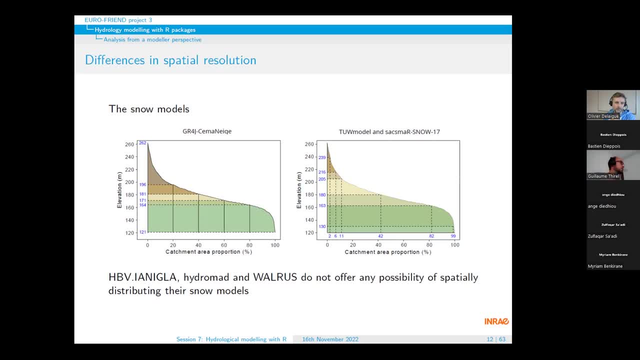 On the left, which is what we classically do with the GR model, and on the right, which is what we classically do with the GR model, meaning that we cut the basin with areas of different proportions, with the same proportion but different altitudes. 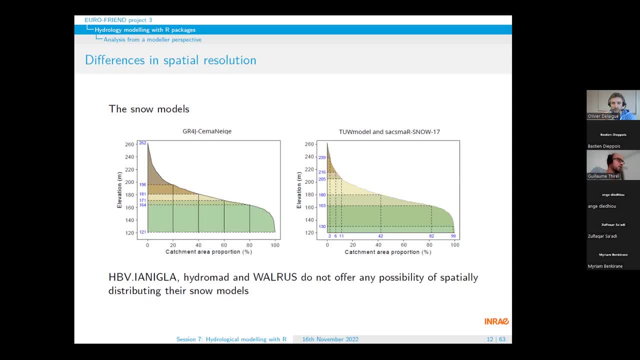 But this is done in a very different way in other packages where you can, for example, specify the different altitudes. And also you have to know that in some packages there is no spatial resolution in the snow model. So HBV, anigla, hydromat and walrus. 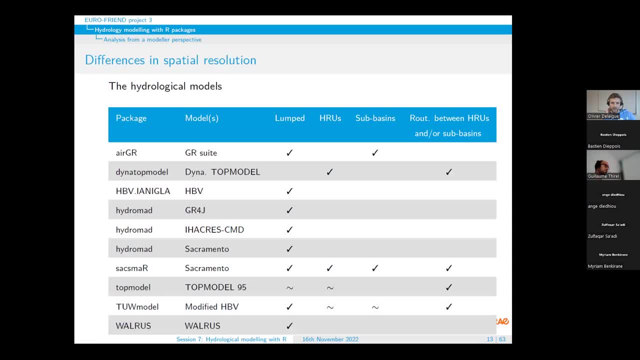 Regarding the hydrological models. here you also have a very, very large diversity in what you have in these packages. Our packages are supposed to be simple tools. The models that are proposed are most of the time lumped, meaning that you represent the basin as a whole. 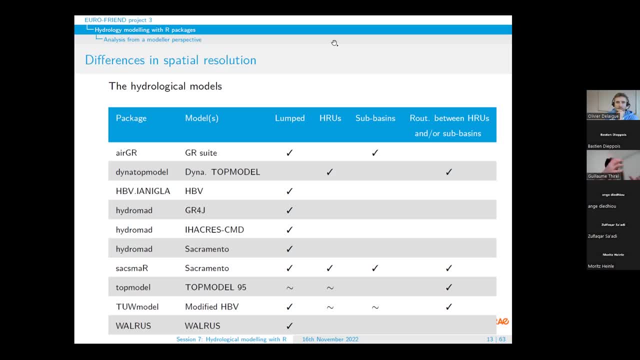 with aggregating precipitation temperature data and simulating the discharge only at the outlet. So this is the case for almost all packages. But some of them go further, like representing the basin with hydrological response units, HRUs. So this is the case of the Dynatop model. 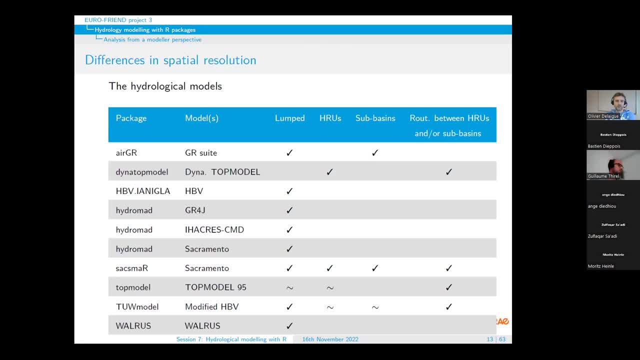 SAC, SMR, top model and TW model packages. You also have the possibility to have subbasins, so semi-distributed modeling of the cations, And you can also have routing between HRUs or subbasins. So this is also important in case. 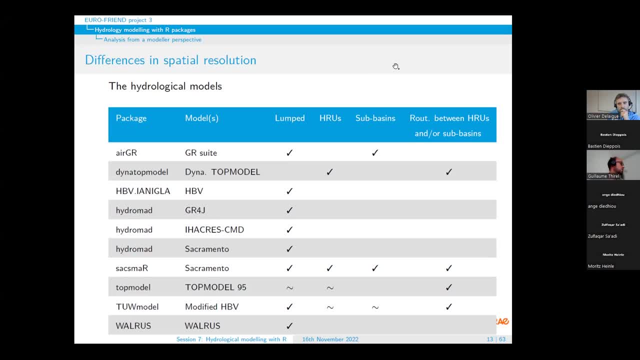 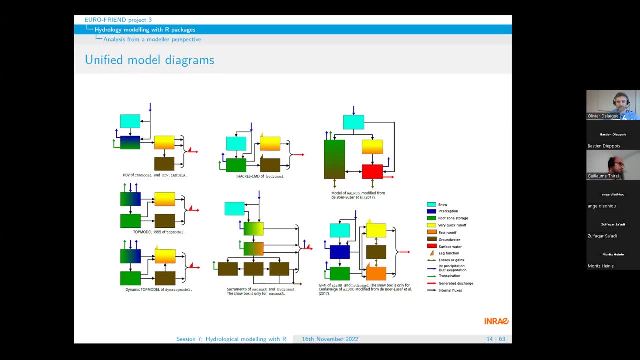 you want to represent a distributed basin. Of course, all models can be very different, So we made some effort to represent the processes implemented in the different models with a quite uniform representation. So this is what you have here, And this is a representation. 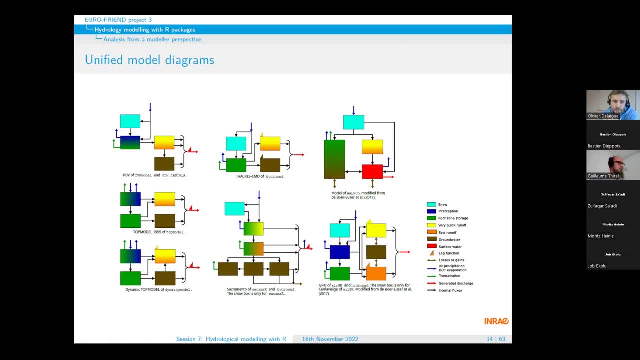 we already developed a couple of years before in the paper from De Boerheuser in 2017.. So I will not have time to go into details for each model, But what you have to see in these diagrams is that each box with a different color represents a different process. 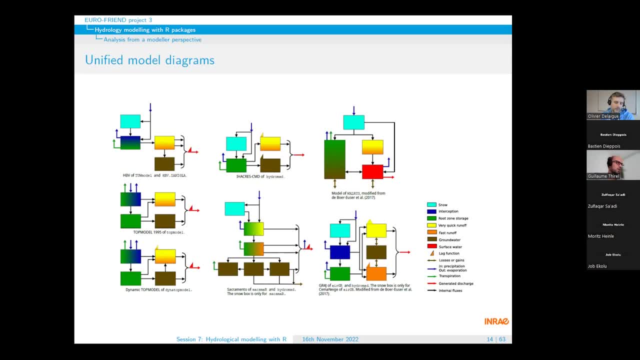 like snow interception, quick runoff, groundwater and so on. Each arrow is a flux And you have a description of how the total streamflow is obtained from the different compartments of the model. So, for example, if I focus on Walrus, 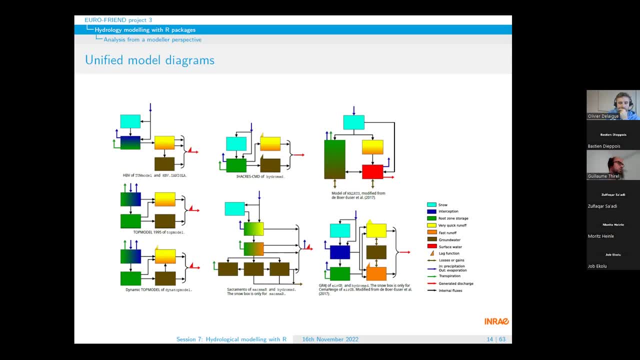 you can see that groundwater is very important, And the reason why it is the case is because Walrus was developed for lowland basins in the Netherlands. So, of course, if you want to work on a very responsive basin with intense rainfall, 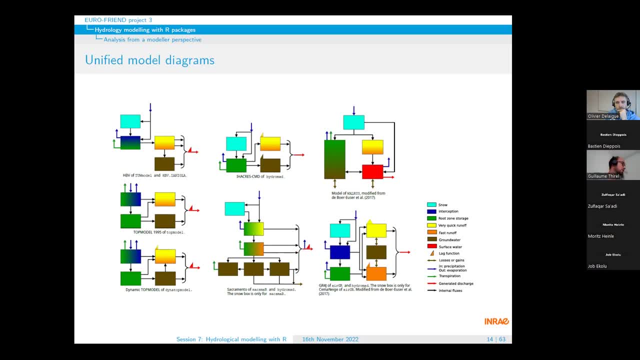 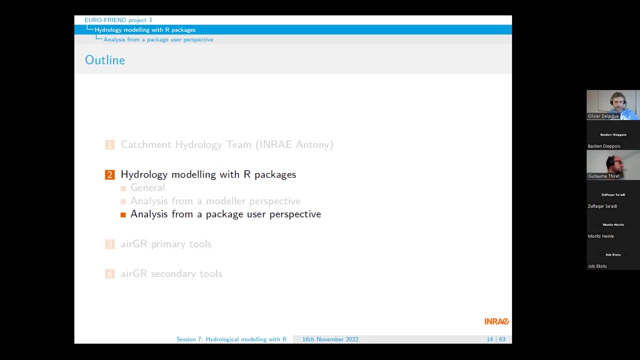 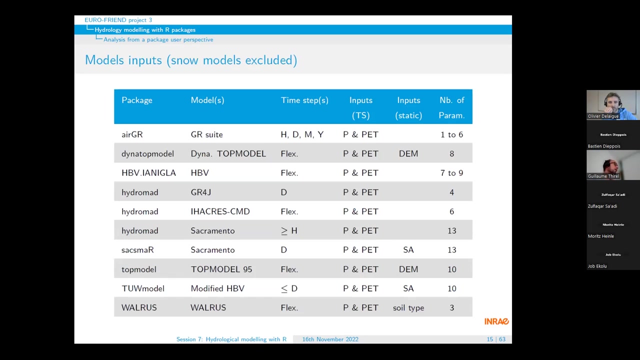 maybe Walrus is not the best solution. So this is a way to help people understand the different models available and make a choice on the package they will pick Now from a package user perspective, we made a couple of additional analyses with different indicators. 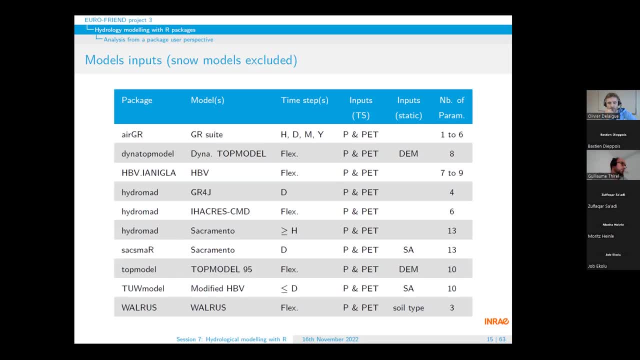 What is important is, of course, the inputs, So not all models need the same inputs, even if all need precipitation and potential evapotranspiration. Some of them need digital elevation models or the soil type, And if you don't have this data, 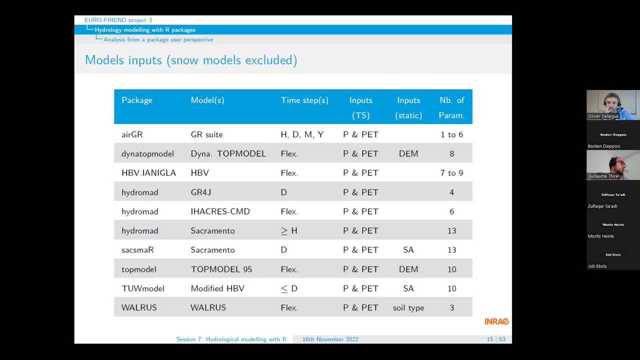 you cannot use this package, So we try to put this information into a simple table. And also the time step available for a different proposed model is very important because if you want to work on flash flood and the model only works on a daily or monthly time step, 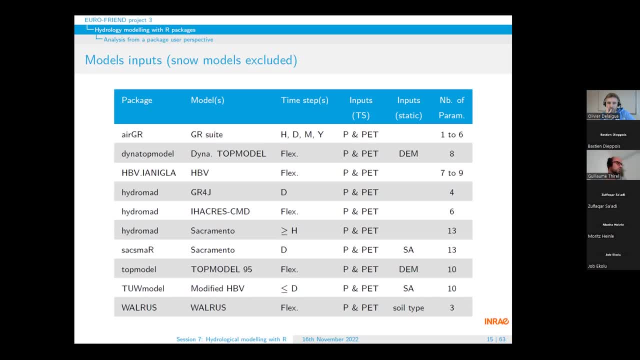 it will not be the best choice for you, So you need to focus only on the models working on a very fine time step. And last, on the right column, you have the number of parameters to optimize, which can be quite important, because the more parameters you have, 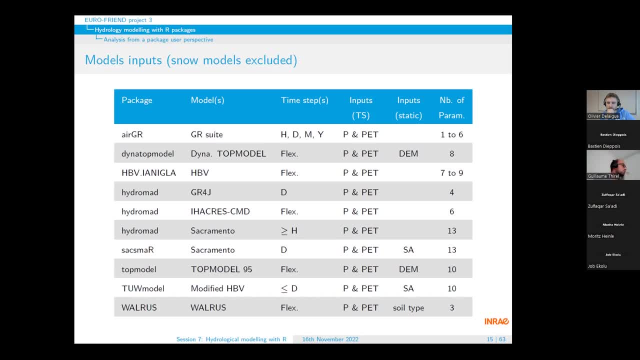 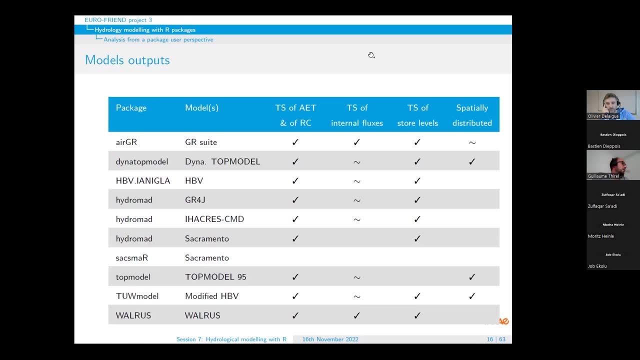 the more difficult it is to find the optimal parameter set. And also, of course, all models propose as an output the simulated discharge. but some packages also propose additional time series of internal fluxes or other compartments. So TS in this table stands for time series. 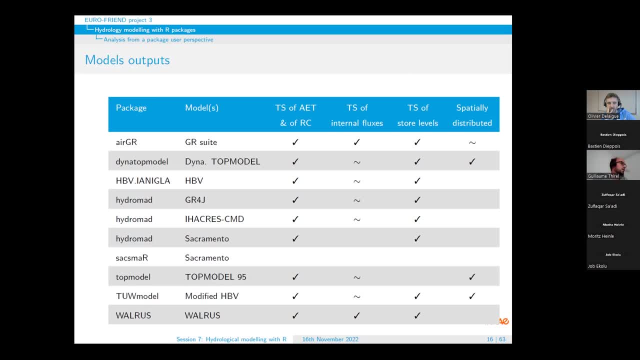 AET is actual evapotranspiration and RC is a runoff component. So, for example, you can see that the SAC-SMA-R package does not propose anything else than discharge as an output. So if you want anything else, this will not be your solution. 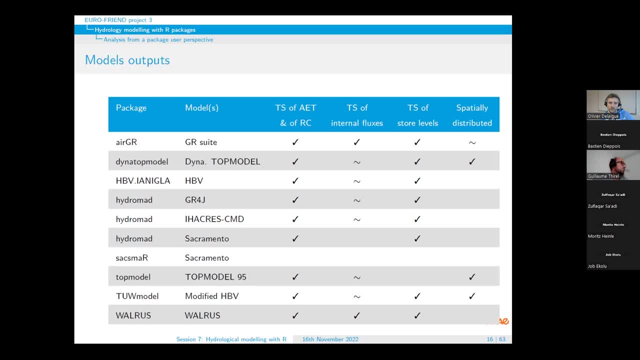 But you can see that if you want to have access to internal fluxes, then you do not have a very large choice, because when there is a till in the table, it means that you only have a couple of internal fluxes. So this can also guide your choice. 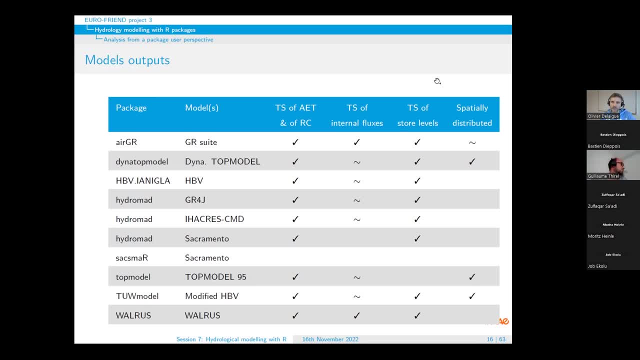 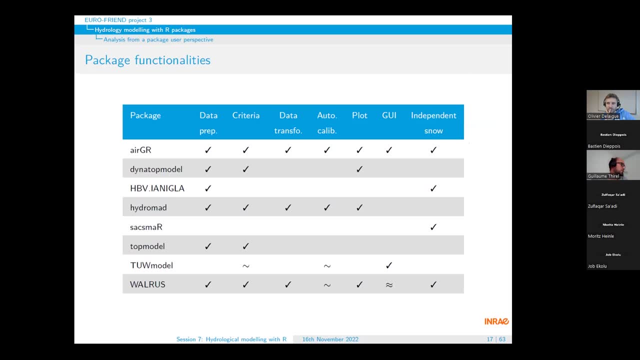 on the package or model you want to use And, in addition, the packages propose different functionalities. Of course, the basis is to have the hydrological model But, as I said, based on our first analysis on the Slater et al paper, 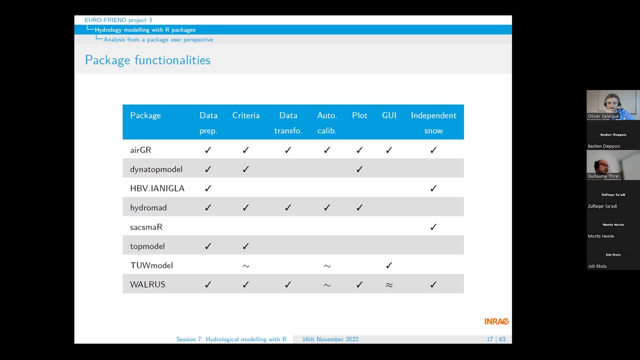 you need more. You need to prepare data. You can be happy to have access to criterion computation to assess the quality of your simulation. You can need a calibration algorithm. Sometimes it's quite difficult to make plots, So you can be very happy. 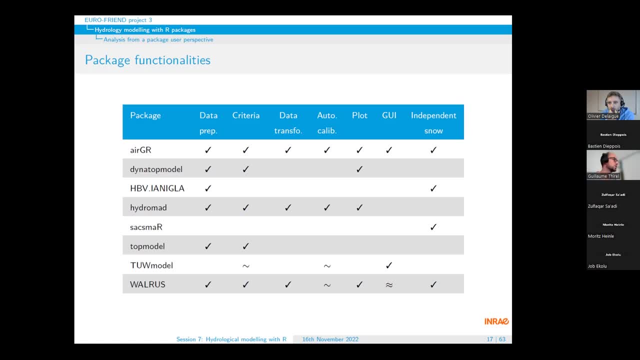 to have very basic plots in the package. You maybe want to have access to a GUI, an interface to manipulate the model, to do some preliminary tests before you use it, Before doing your modeling, And also maybe you want to work only on snow. 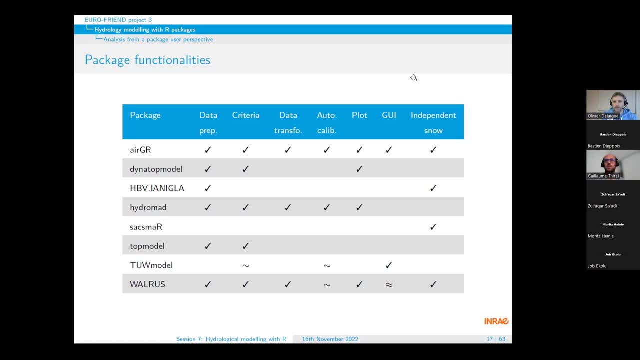 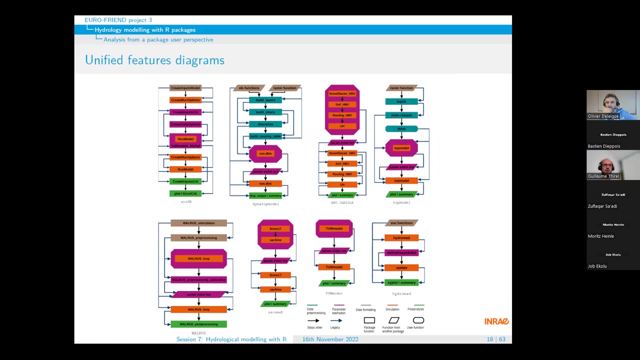 without going down to discharge. So some packages propose that, but not all of them. So this kind of table also shows what you can expect in the package before choosing one of them. Okay, We also propose very, very complicated diagrams here. 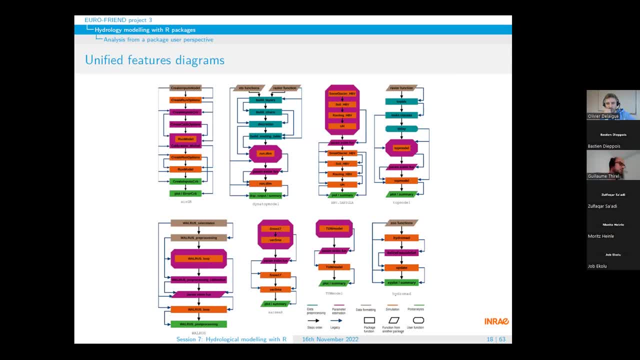 that I will not present into details. So this is really useful if you start using the package. So no worries if you don't understand that Here it's just for each package. we described the diff. We put the names of the functions. 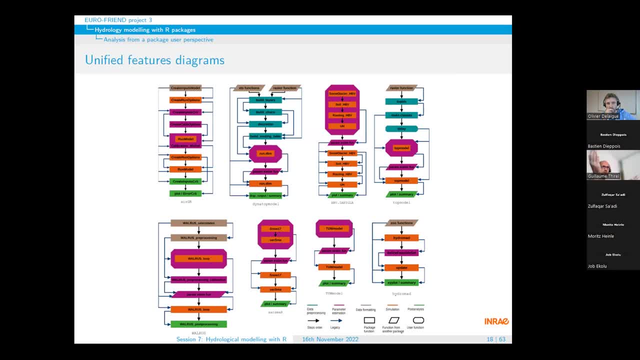 that you need to use to make a complete modeling exercise, from data preparation to modeling and to the analysis of the outputs. Why did we do that? It's because the more you can tune your modeling exercise, the more functions you will need, But still it's not very easy. 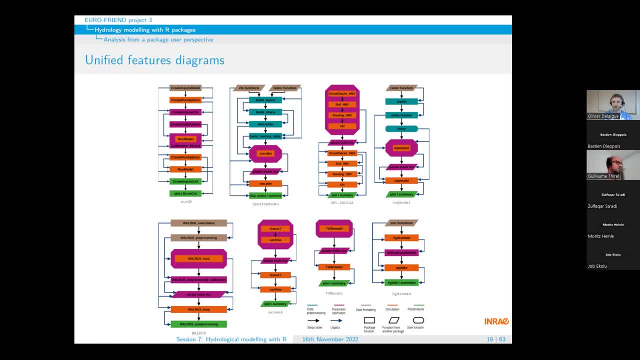 always to understand which function to use first and then which one you need to use, and so on, And it's very, It can be very difficult to understand the relationship between the different functions. So with this kind of graph, we hope that it's a bit more easy. 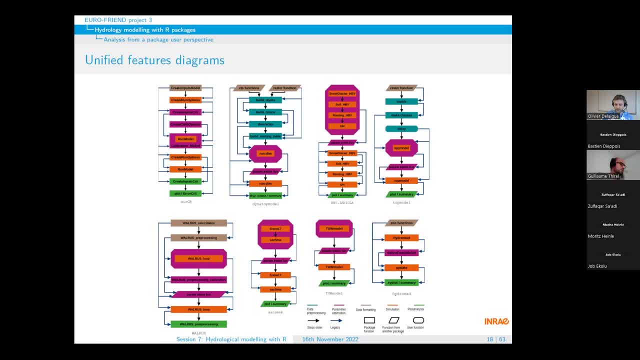 to understand and we try to put some different colors for the modeling step, data preparation, parameter estimation, stimulation and so on. So I will not say more about this, Because it's only needed when you start using the packages. And finally, 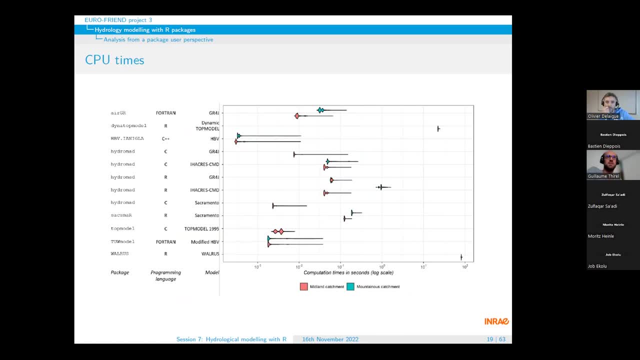 of course, we did some analysis of how fast the different packages are. Why did we do that? Because not all packages only include R code. This is something nice: With R, you can also use different programming languages, And especially some of them. 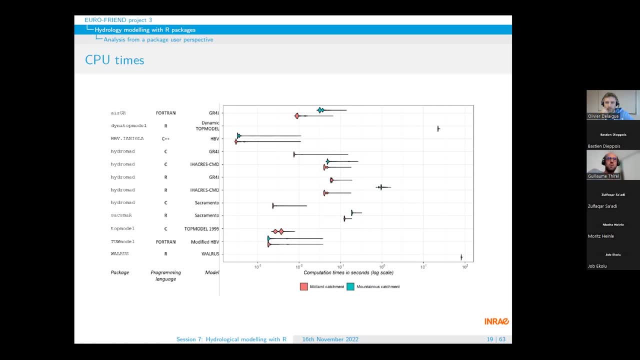 that can be compiled can be quicker to execute, which is very important when you want to do multiple runs for your models, So for uncertainty, analysis or also for calibration. So here we made many, many computations on the different models and the different packages. 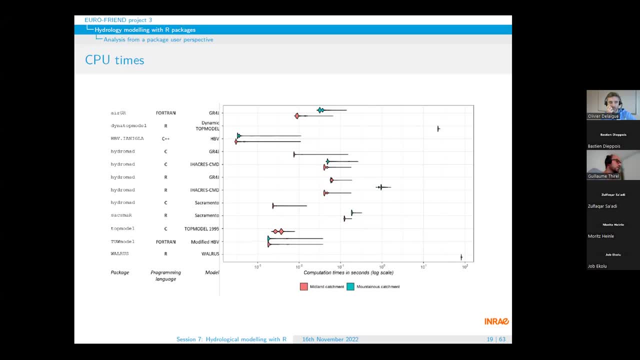 And we did that for a mountainous catchment in blue-green And we also did that for a midland catchment in orange. So the difference between the two is that you have a snow model or not, And here you can see that. 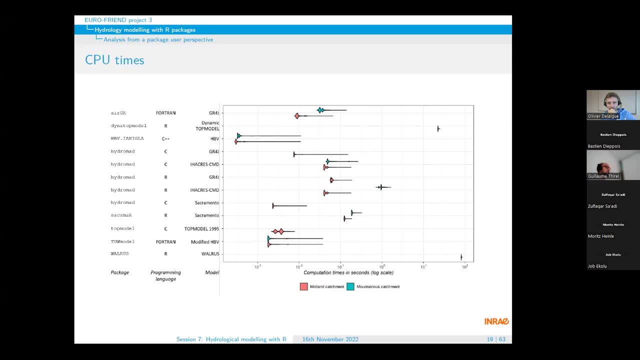 you have a very large panel of computation time So depending on the number of catchments you have for the modeling you want to do, this might guide your choice. also Because for some packages that need many seconds to do one run if you want to do a very complex. 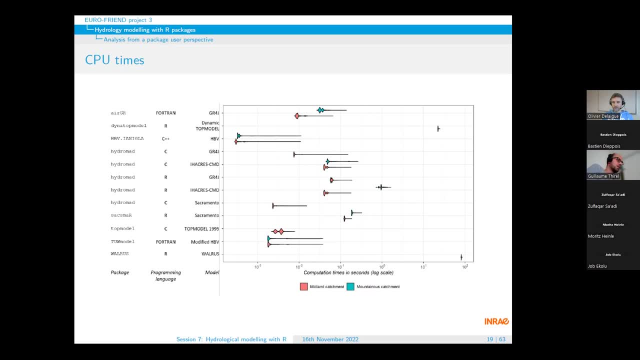 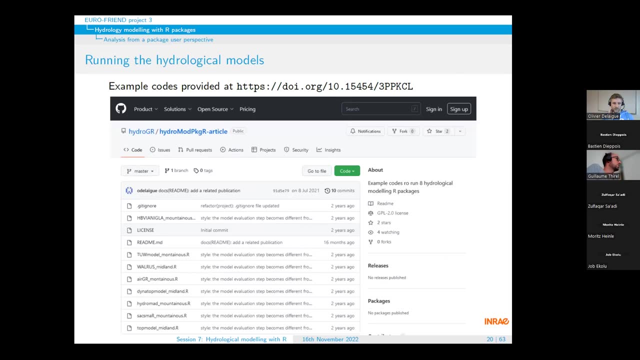 for example, Monte-Caro analysis. it might be more difficult, And so this is where we have put the codes to run the different models as the different packages. So these are very simple codes, just to prepare data to make a run. 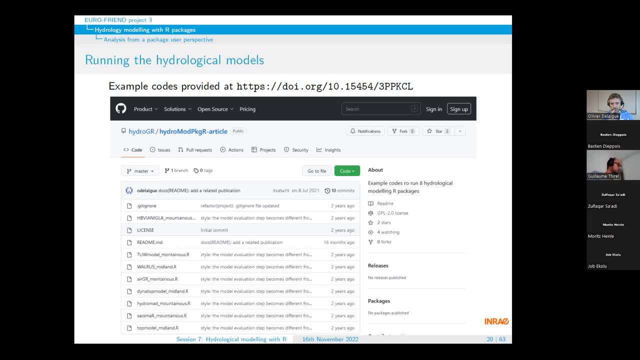 We did not include in these codes the calibration of the parameters after many discussions with our colleagues, And the main reason why we did that is because the calibration of parameters is something that has to be decided by users, based on what they want to do and the problems they have. 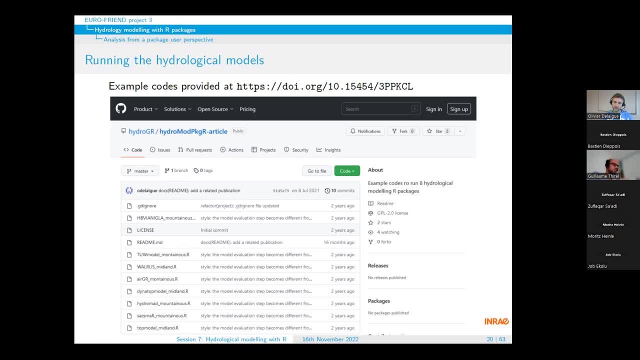 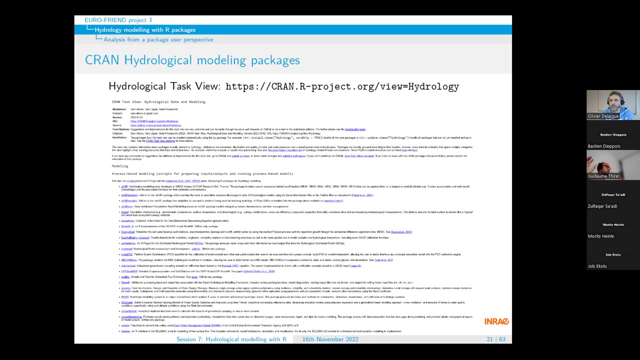 And there is no global solution that might be applied in every case. And to finish, to open a bit more the landscape around- that we can also check what we call a task view in the CRAN website, because we have a hydrological task view. 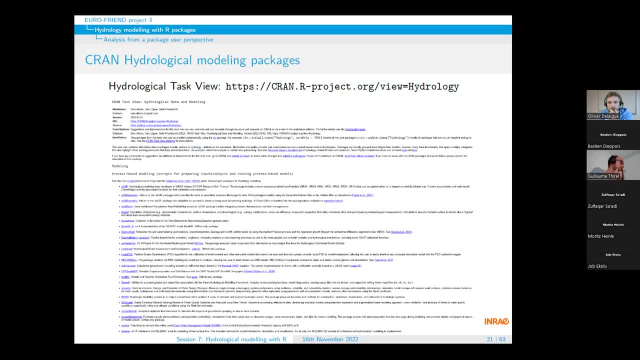 So a task view is something that it's a list of packages around the topic, And in this task view you have a quite complete and updated list of packages around the hydrological modeling or hydrological data and everything that goes around that, So it can be a very, very interesting. 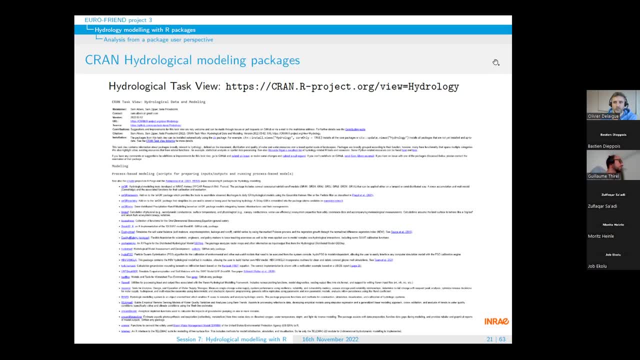 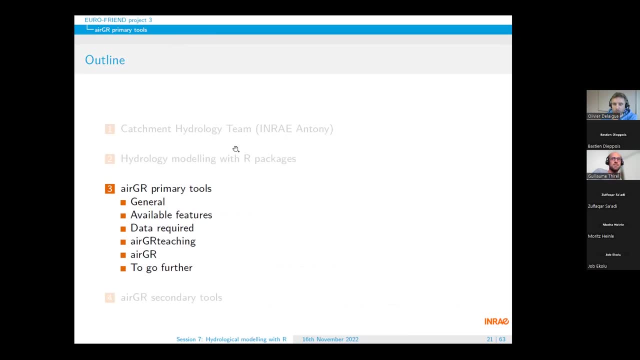 source of information for you also. And now we will focus on Ergo's main tools. So the objective of these tools- there are many objectives: to have a model core in Fortran. The goal to have a code in Fortran is to have a speed. 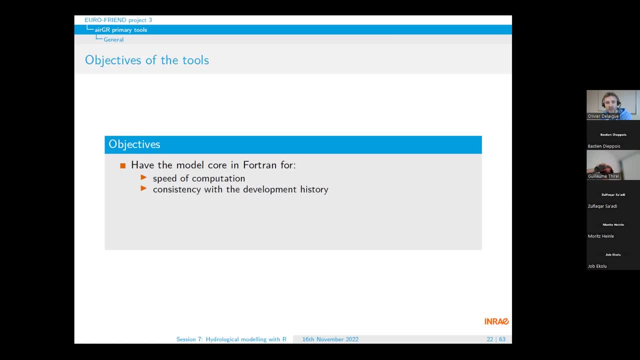 to ensure speed computation and the consistency with the development history of the GR model, And to use a more flexible language than the Fortran for additional functionalities And to have a tool that is free, open source and easy to disseminate. That's why we decide. 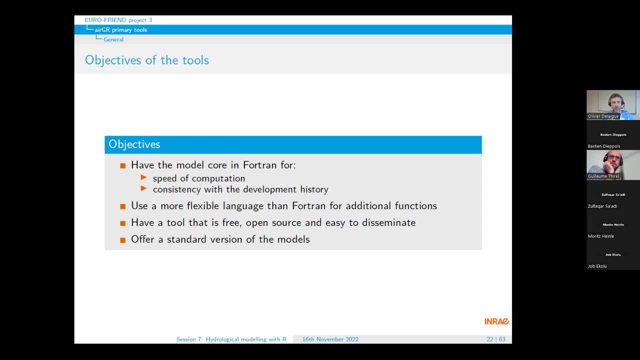 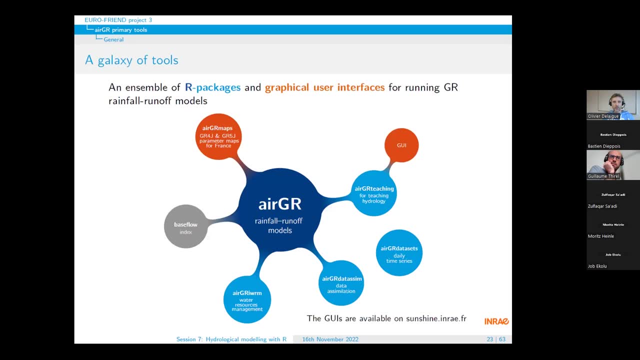 to develop the RGR package And we want to offer a standard version of the different model we developed. So that's why we developed many tools You can see on this graph. I will focus in the first time to RGR and RGR teaching. 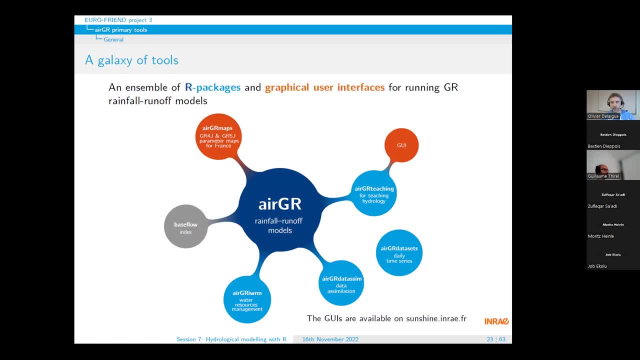 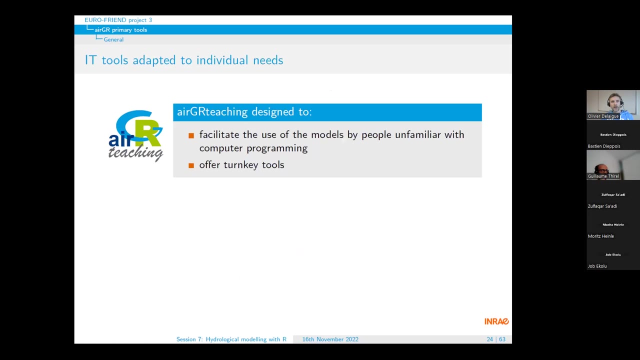 which are our packages, And we have also a graphical user interface, which are available on a shiny sunshine in-ray website. So let's go on RGR and RGR teaching. These tools are quite similar but adapted to individual needs. 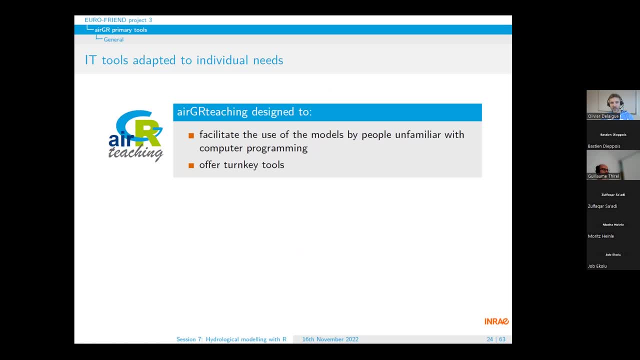 So RGR teaching is designed to facilitate the use of the models by people which are unfamiliar with computer programming. So it is a software that is designed to build and implement RGR And it offers turnkey tools. So it's developed. 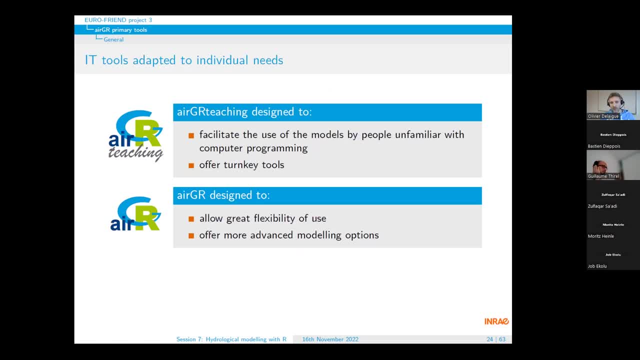 especially for students, And RGR is designed to allow great flexibility of use and offer more advanced modeling options. But in fact you have to keep in mind that RGR and RGR teaching offer the same hydrological models, But in fact 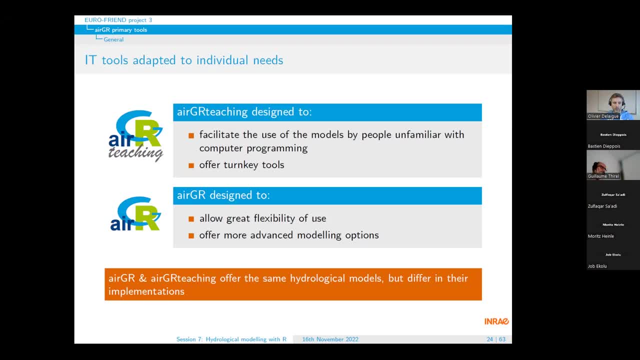 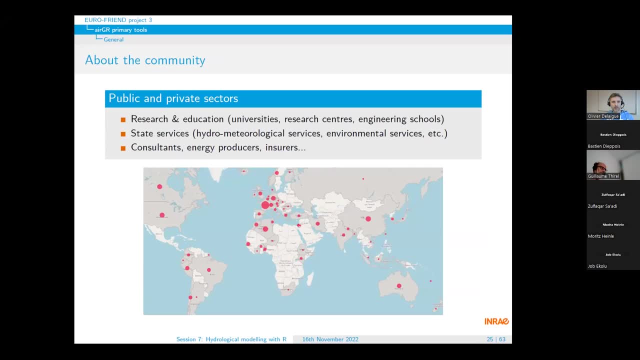 they differ just in their employment tension and their manner. uh about the community of the rgr packages. so the people who use these packages uh work in public or private sectors, as a research and education uh, as a university research centers and so on. uh also state services. i uh as a hydro meteorological services on very 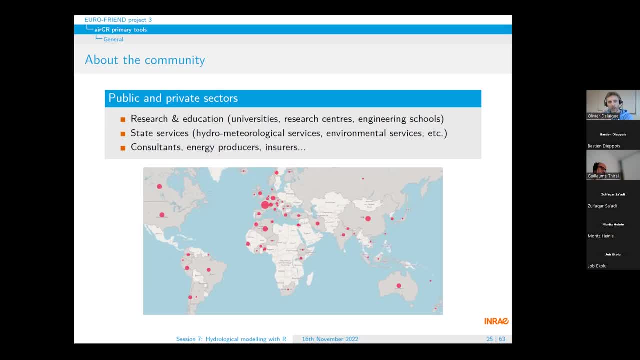 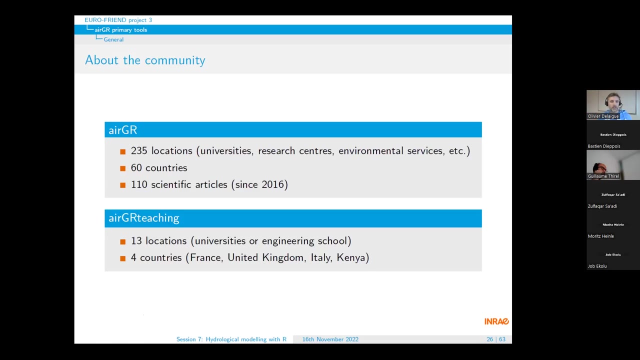 services and so on, and consultants, energy producer, insurers, so you can see on the map. but uh, it's uh about only the rgr package, which is used uh on all continents and we have counts more than 200 locations uh as university research centers and so on, who use 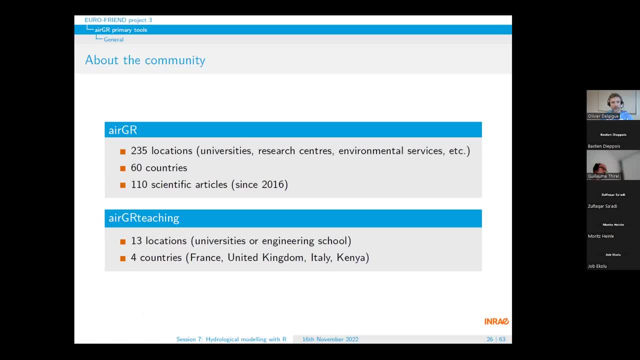 rgr more than 60 countries and uh. currently there are more than 100 scientific articles who use rgr and rgr teaching as it's developed for teaching hydrological modeling. it's less used and we we count 13 locations as universities and engineering school in france, united kingdom, italy and kenya. we use this package. 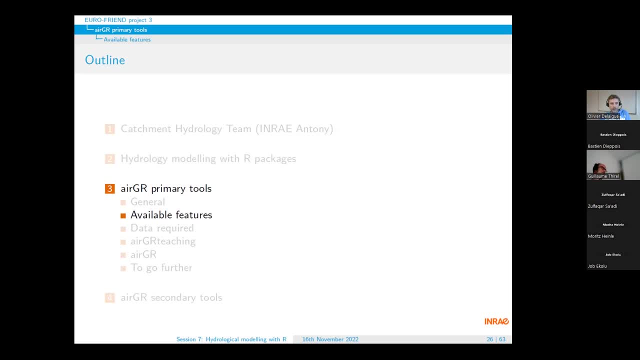 uh, i will focus on on available features. um, so the immediate features are: uh, the suit of the gr rainfall runoff models. i will, i will, uh will present them just after a snow model called semanage, a calibration algorithm, efficiency criteria and data processing and display tools. 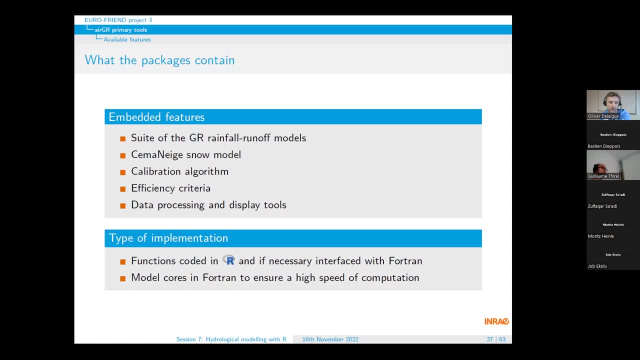 as i said previously, the type of, as i said previously, the type of, as i said previously, the type of implementation. so the implementation, so the implementation, so the. the package are in r. the package are in r. the package are in r, but they are embedded, they are linked, they. 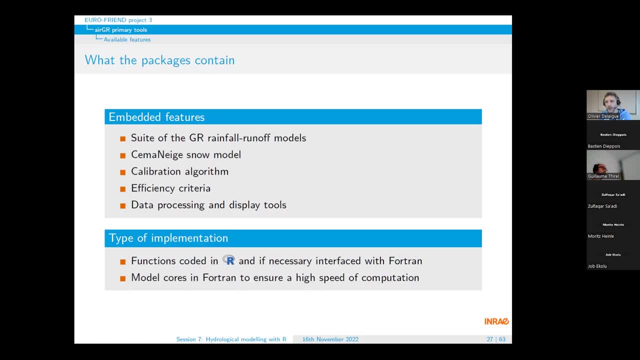 but they are embedded, they are linked, they, but they are embedded, they are linked. they are interfaced with fortran code to are interfaced with fortran code, to are interfaced with fortran code to ensure uh, ensure, uh, ensure, uh quickness and uh, quickness and uh. 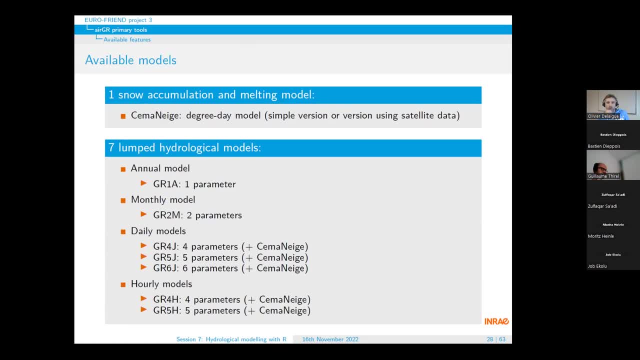 quickness and uh, yeah, yeah, yeah the model available. so, as i said, there the model available. so, as i said, there the model available. so, as i said, there is semanage, so it's a degree day model is semanage, so it's a degree day model. 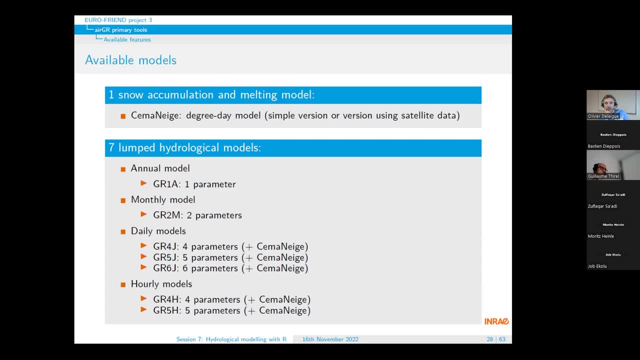 is semanage, so it's a degree day model to to, to. to simulate snow accumulation and melting. to simulate snow accumulation and melting. to simulate snow accumulation and melting model model model. there is a simple version in rgr, but there is a simple version in rgr, but 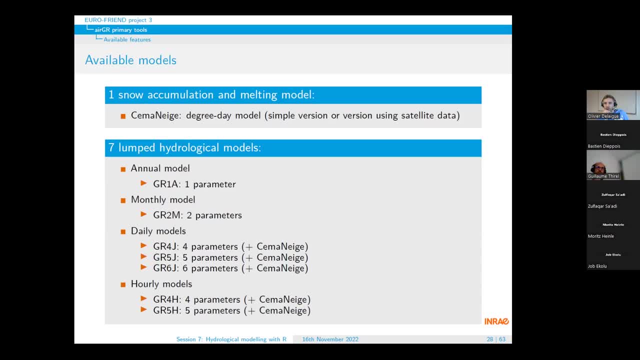 there is a simple version in rgr, but there is also a version. there is also a version. there is also a version which allows to use a satellite data, as which allows to use a satellite data, as which allows to use a satellite data as the modest data, for example. 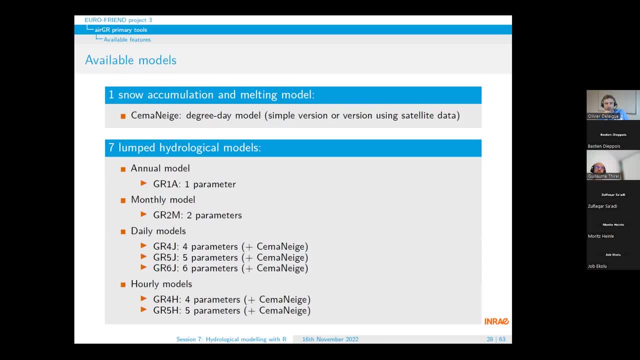 the modest data, for example. the modest data, for example. and in the and in the and in the suit of models. there are seven lumped suit of models. there are seven lumped suit of models. there are seven lumped hydrological models. hydrological models, hydrological models from. 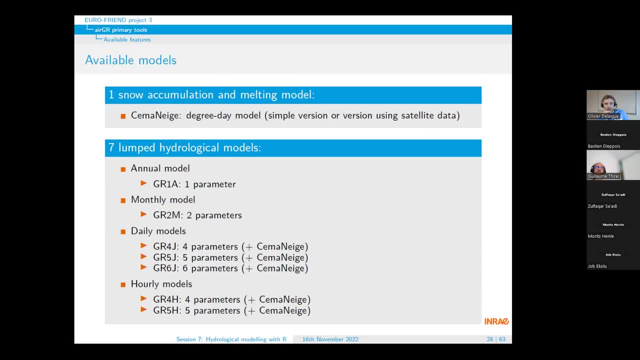 from: from the yearly to the early time step, the yearly to the early time step, the yearly to the early time step. so there is an annual model called gr1a, so there is an annual model called gr1a, so there is an annual model called gr1a with uh, with one parameter only. 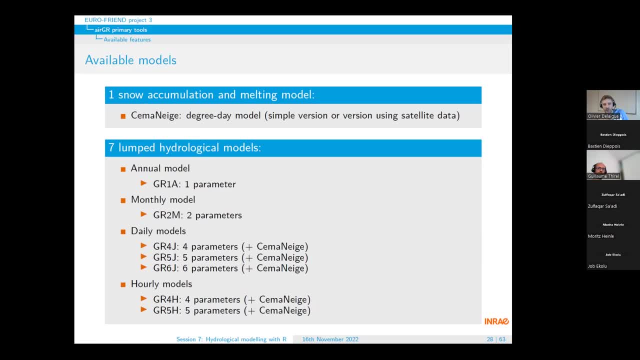 with uh, with one parameter, only with uh, with one parameter only. monthly model, three daily models. so the monthly model, three daily models. so the monthly model, three daily models. so the most famous is gr4j, but we, you can see, most famous is gr4j, but we, you can see. 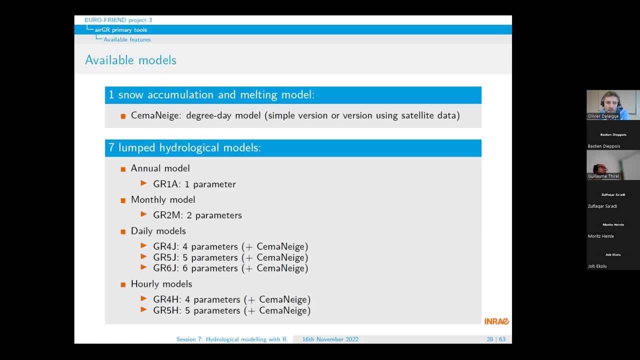 most famous is gr4j, but we, you can see that there are, that there are that there are gr5j and gr6j, gr5j and gr6j, gr5j and gr6j, which are more, which are more, which are more useful to 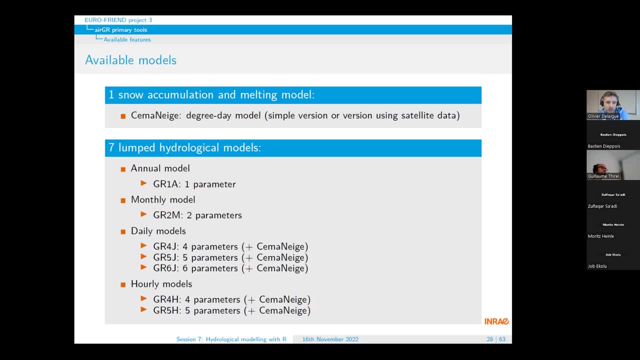 useful to. useful to to simulate low flows. to simulate low flows. to simulate low flows, and two early models, gr4h and gr5h, and two early models, gr4h and gr5h, and two early models, gr4h and gr5h, and the daily and the only models can be: 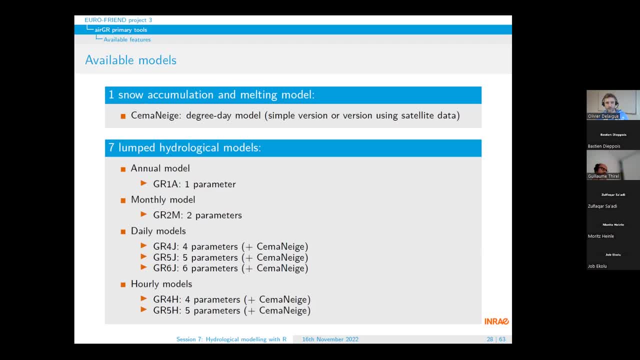 and the daily and the only models can be, and the daily and the only models can be coupled with uh the snow model, coupled with uh the snow model, coupled with uh the snow model. semanesh: the available criterion: uh are these ones. the available criterion: uh are these ones. 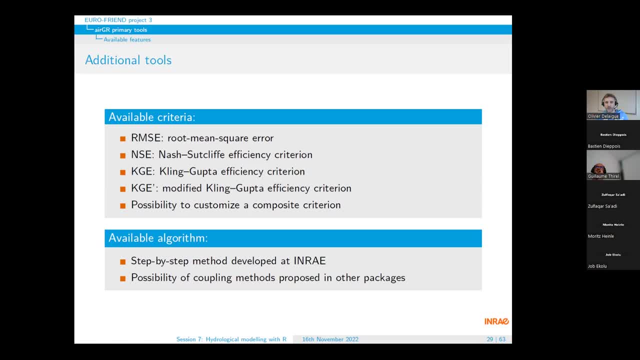 the available criterion. uh, are these ones. so the root means warrior the national. so the root means warrior the national. so the root means warrior the national. saskif efficiency criterion. the king and saskif efficiency criterion. the king and saskif efficiency criterion. the king and gupta efficiency criterion. 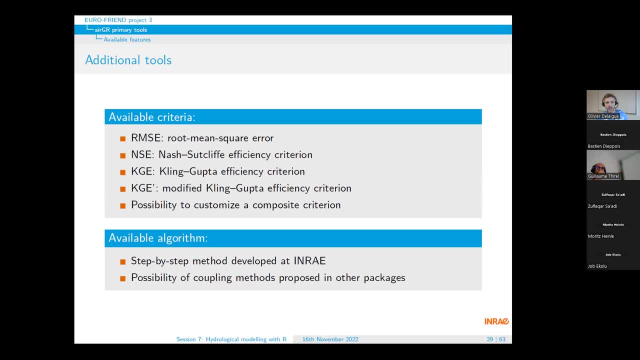 gupta efficiency criterion. gupta efficiency criterion, the, the, the modified version of the kge and it's modified version of the kge and it's modified version of the kge, and it's also possible also possible also possible to customize a composite criterion. to customize a composite criterion mixing different. 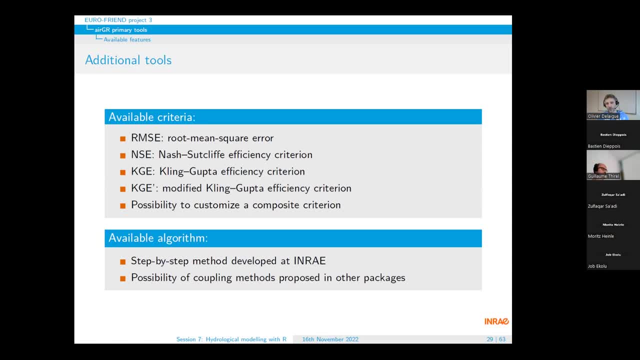 mixing, different mixing, different criteria and different criteria and different criteria and different spring flow transformations. we give with the package. we give with the package. we give with the package an algorithm to calibrate the model. so an algorithm to calibrate the model, so an algorithm to calibrate the model. so it's a step-by-step method developed at 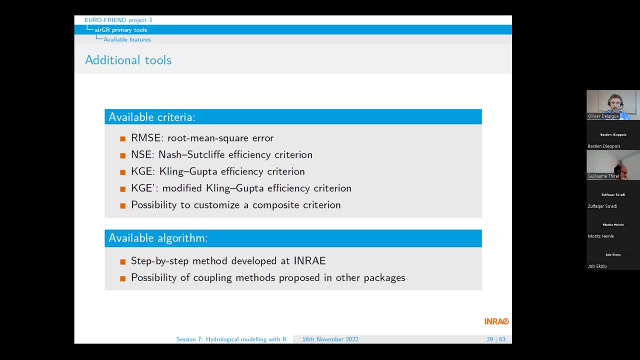 it's a step-by-step method developed at. it's a step-by-step method developed at inari, but it's also possible to couple inari. but it's also possible to couple inari. but it's also possible to couple. some other methods are as a mcmc or 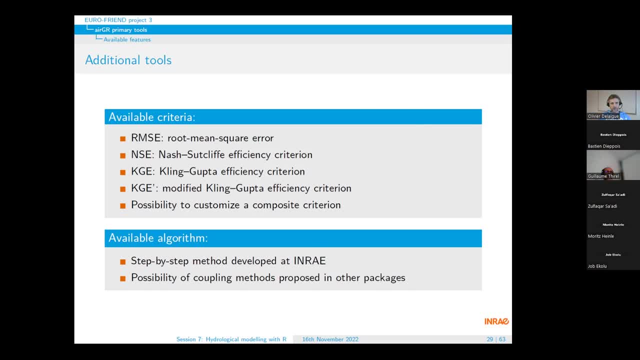 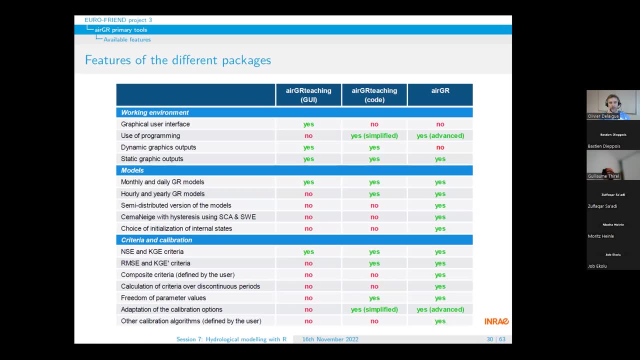 some other methods are as a mcmc, or some other methods are as a mcmc, or, and so on, and so on, and so on. methods methods. i will not detail all this table, but i will not detail all this table. but i will not detail all this table, but you can see here. 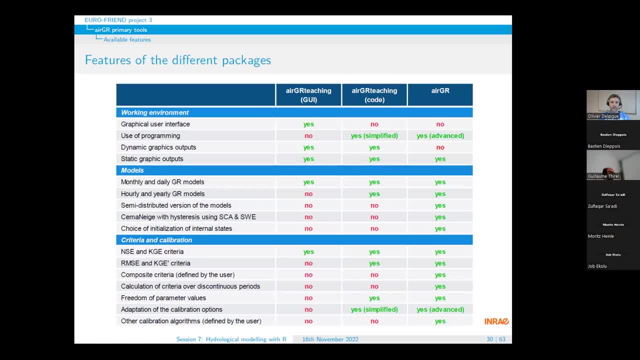 you can see here. you can see here the different option. you can use the different option. you can use the different option you can use with the different packages: lgr teaching allowed to. lgr teaching allowed to. lgr teaching allowed to. to launch a graphical user interface. but 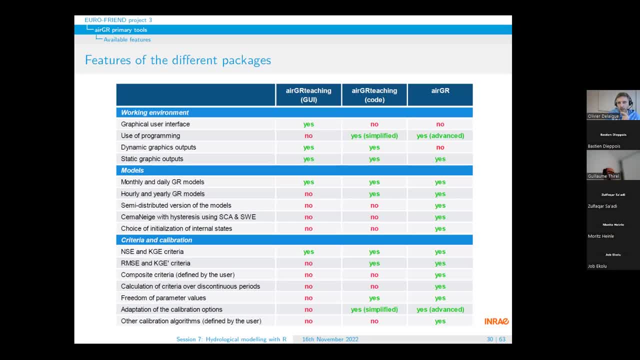 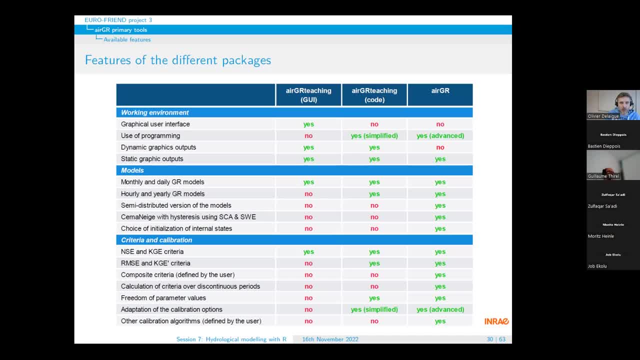 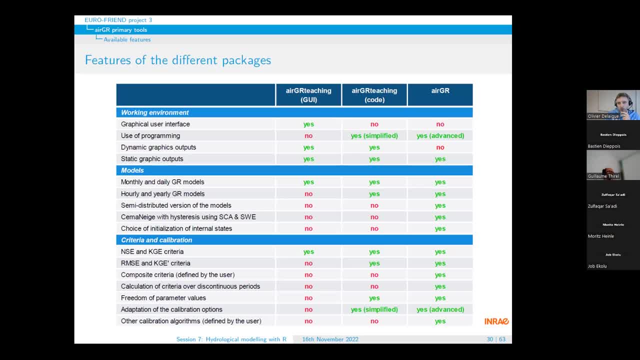 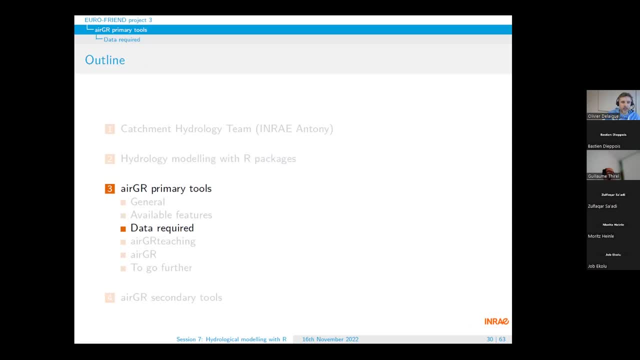 the graphical user interface allows to. the graphical user interface allows to use less options. use less options. use less options. and erger is a more complete tools to and. erger is a more complete tools to and erger is a more complete tools to use. but, in any case, the data required by the 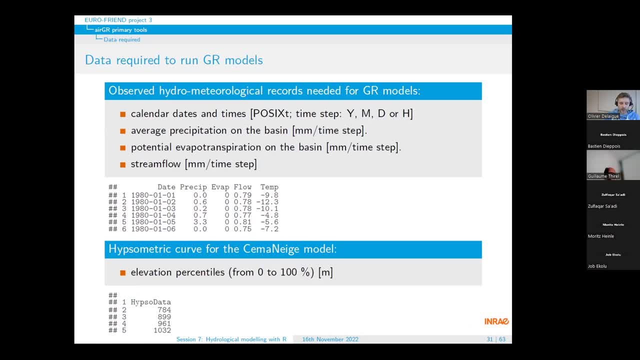 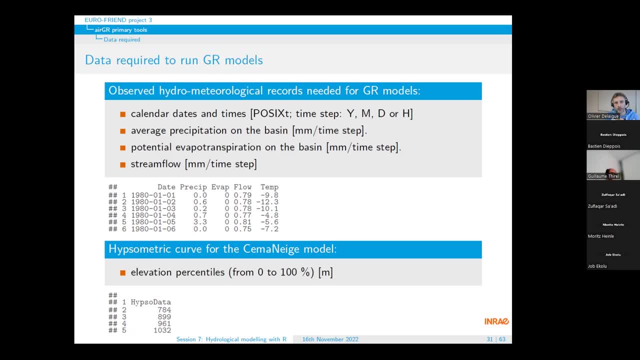 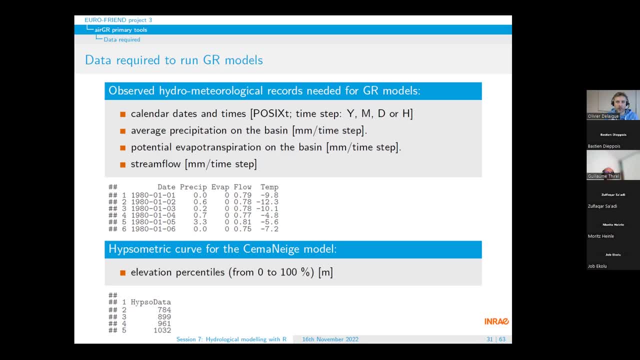 in r, it's in the posix t format. in r, it's in the posix t format and it depends of your model, but you and it depends of your model, but you and it depends of your model. but you need to have need to have need to have yearly, monthly, daily or only the time. 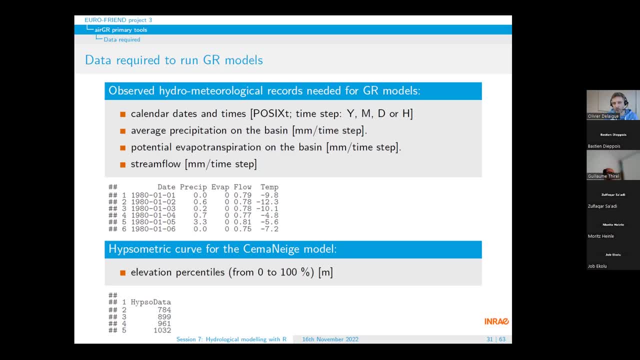 yearly, monthly, daily or only the time. yearly, monthly, daily or only the time, step, step, step, depending of if you use gr4j or depending of if you use gr4j, or depending of if you use gr4j or gr1a, gr1a, gr1a. you need obviously. 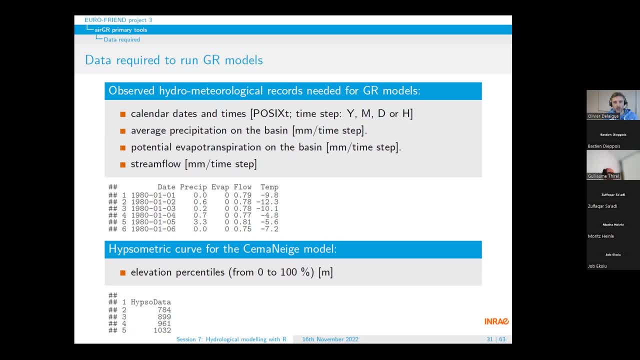 you need obviously. you need obviously the average precipitation on the. the average precipitation on the. the average precipitation on the. on the catchment in millimeters. on the catchment in millimeters. on the catchment in millimeters. the potential evaporator- evapotranspiration. the potential evaporator- evapotranspiration. 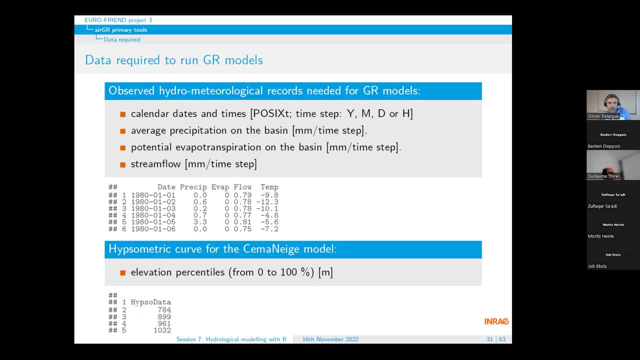 the potential evaporator, evapotranspiration on the catchment, on the catchment, on the catchment, and if you want to calibrate your model, and if you want to calibrate your model, and if you want to calibrate your model, you need the stream flow. 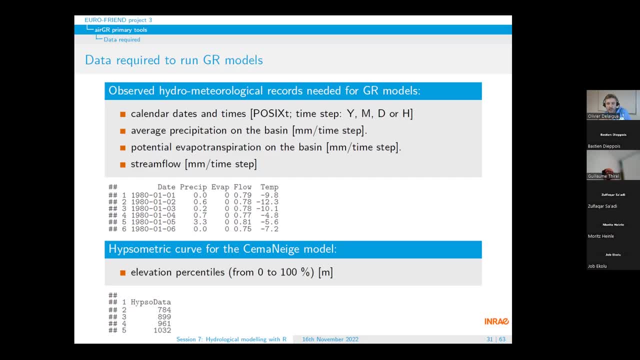 you need the stream flow, you need the stream flow all in millimeters, all in millimeters, all in millimeters. you can see that you have an additional. you can see that you have an additional. you can see that you have an additional. column with the temperature, column with the temperature. 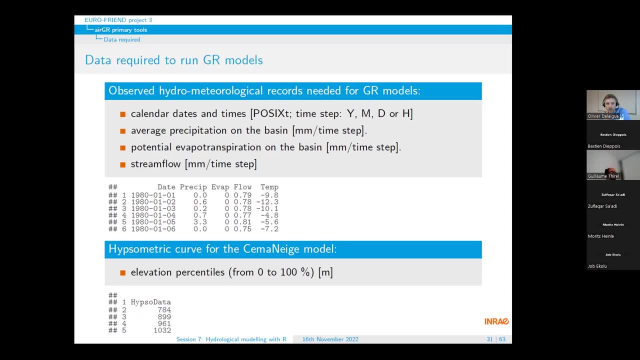 column with the temperature. it's, it's, it's when you use the semanage model and if you want to uh to activate the and if you want to uh to activate the and if you want to uh to activate the, the snow model, the snow model. 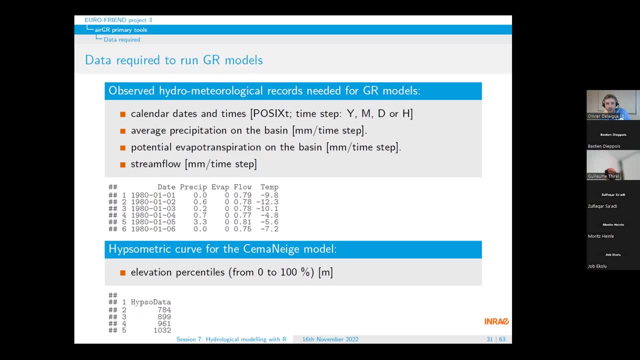 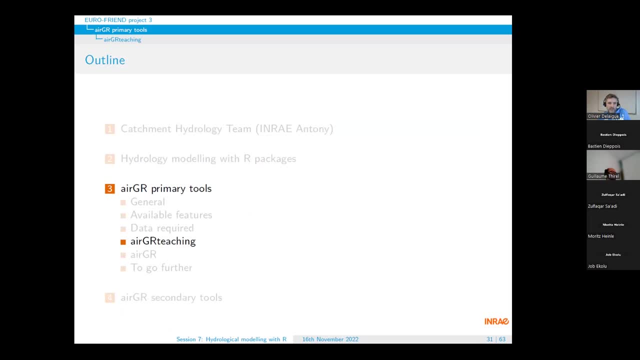 the snow model. you need the elevation percentiles of your, you need the elevation percentiles of your, you need the elevation percentiles of your catchments, and that's it, and that's it, and that's it. uh so, uh so, uh so. these data are required for rgr teaching. 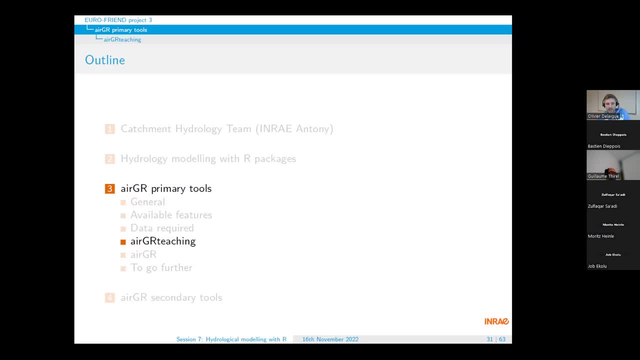 these data are required for rgr teaching. these data are required for rgr teaching, and rgr because, and rgr because, and rgr because there allows to use exactly the same, there allows to use exactly the same, there allows to use exactly the same models, models. 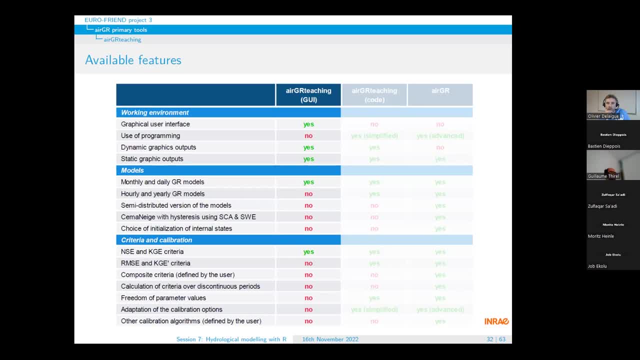 models, as i said previously, as i said previously, as i said previously. so i will focus in a first time to the, so i will focus in a first time to the. so i will focus in a first time to the graphical user interface of rgr teaching. graphical user interface of rgr teaching. 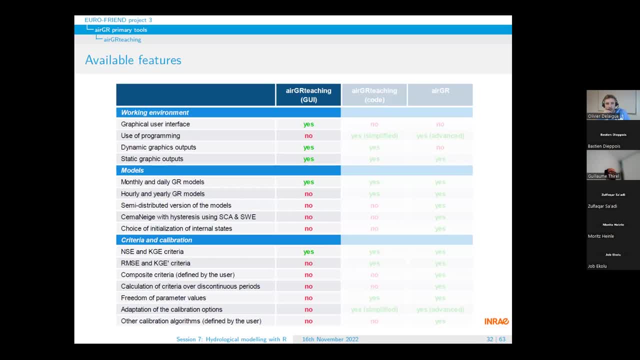 graphical user interface of rgr teaching. so in this case, you just need so. in this case, you just need so. in this case, you just need to launch one function and to launch one function and to launch one function and it will open in the browser. it will open in the browser. 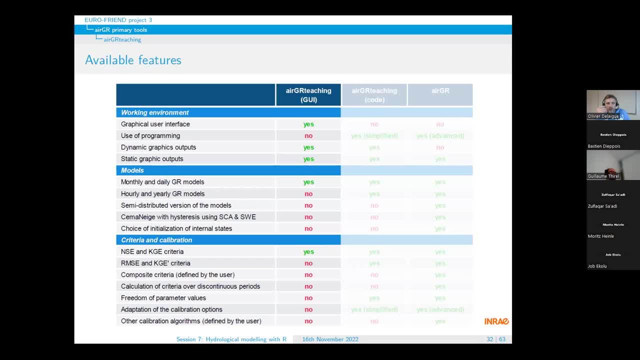 it will open in the browser the graphical user interface. the graphical user interface. the graphical user interface. you have some dynamic graphics. when you have some dynamic graphics. when you have some dynamic graphics, when, where you can zoom on, where you can zoom on, where you can zoom on, it's only possible to use in this. 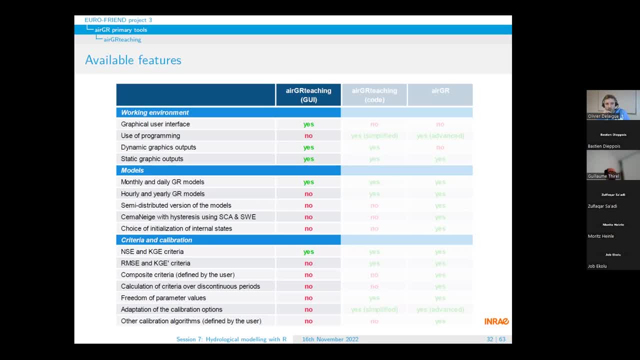 it's only possible to use in this. it's only possible to use in this interface the monthly and the daily interface, the monthly and the daily interface, the monthly and the daily models. models models, not the early models, not the early models, not a semi-distribution distributed. 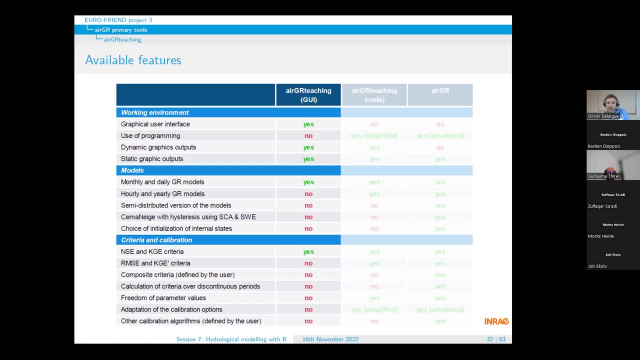 not a semi-distribution distributed, not a semi-distribution distributed. sorry version of the models, sorry version of the models, sorry version of the models. so it's quite limited, so it's quite limited, so it's quite limited. uh, uh, uh, the data needed are exactly the same. i. 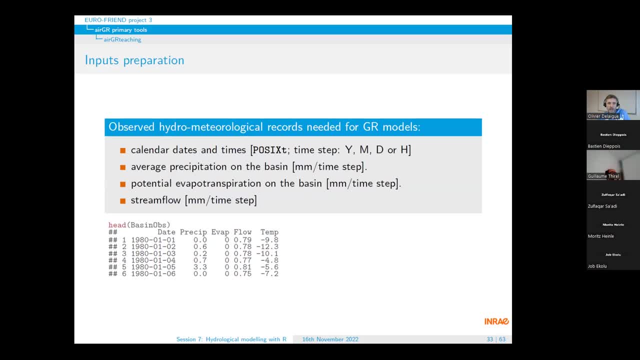 the data needed are exactly the same. i, the data needed are exactly the same. i present, present, present, previously so the dates. the previously so the dates, the previously so the dates. the precipitation, precipitation, precipitation, the potential evapotranspiration and the. the potential evapotranspiration and the. 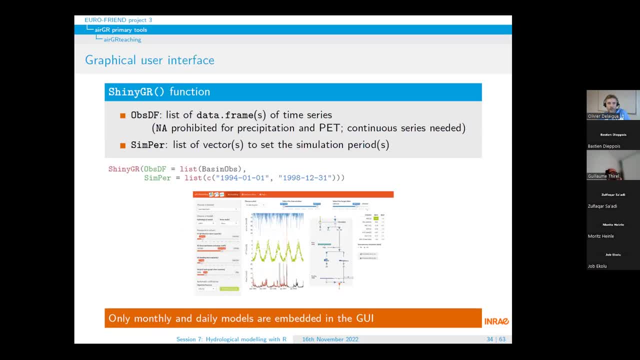 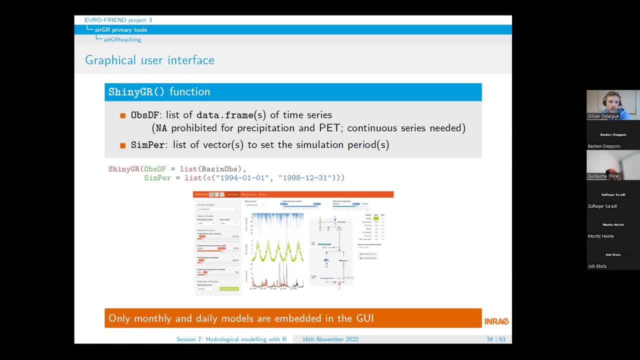 the graphical user interface. this, the graphical user interface, this function function is called chinese gr function function is called chinese gr function function is called chinese gr and you need to to put your time series and you need to to put your time series and you need to to put your time series and to set. 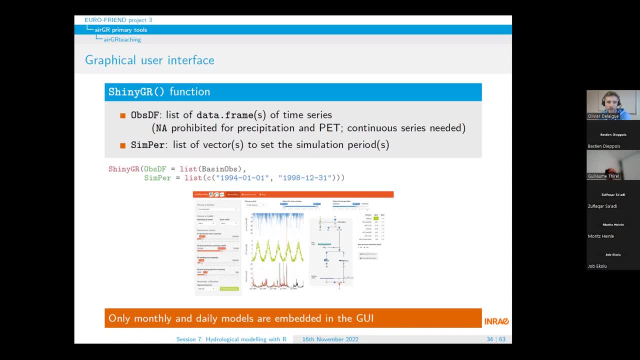 and to set, and to set the period you want to simulate on the period you want to simulate on the period you want to simulate on. you have a screenshot here of the. you have a screenshot here of the. you have a screenshot here of the graphical user interface. 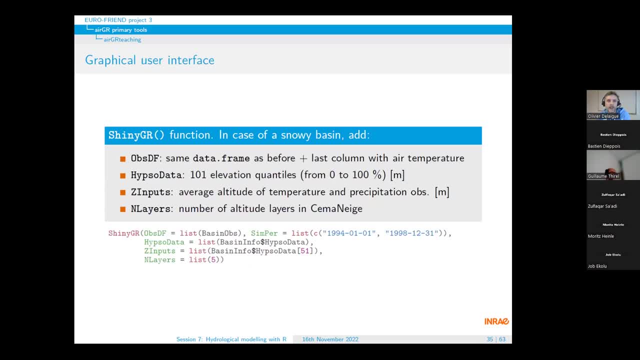 graphical user interface. graphical user interface: i, i will detail it, i, i will detail it, i, i will detail it just after. if you want to activate the snow, if you want to activate the snow, if you want to activate the snow model, model model, you need, uh, the asymmetric data. 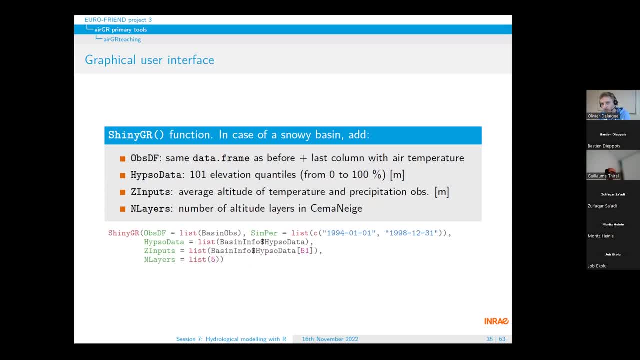 you need uh the asymmetric data. you need uh the asymmetric data: the average altitude of the temperature, the average altitude of the temperature, the average altitude of the temperature, and the and the and the precipitations, precipitations, precipitations and the number of layers and the number of layers. 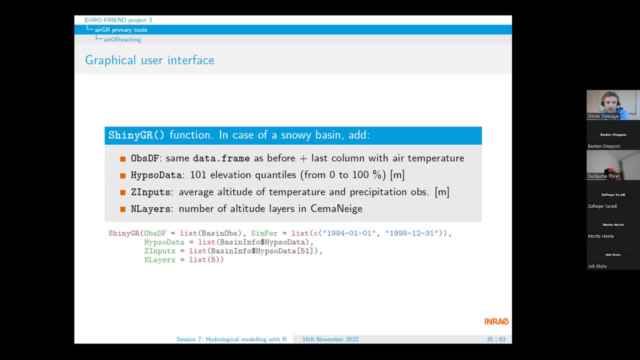 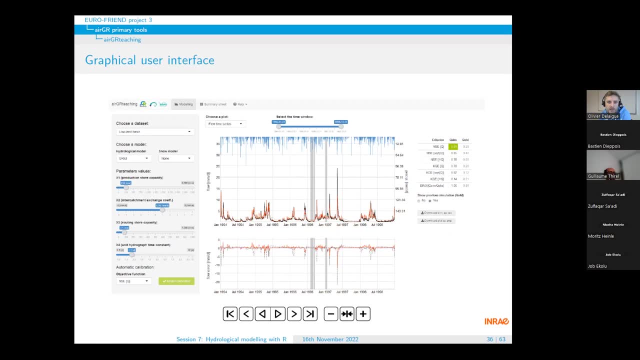 and the number of layers to compute the snow model. so here you have a screenshot of the. so here you have a screenshot of the. so here you have a screenshot of the graphical user interface. graphical user interface. graphical user interface. so it's open in your browser. so it's open in your browser. 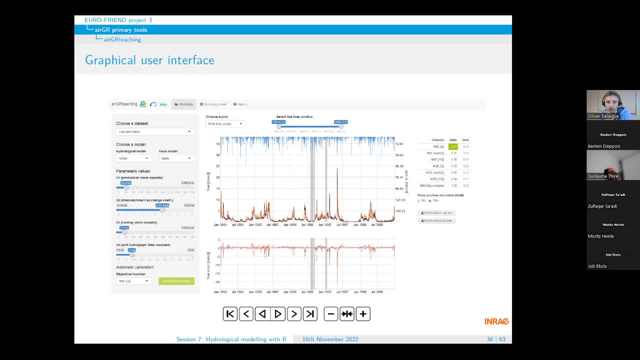 so it's open in your browser. it's: uh, there is also a demo. it's- uh, there is also a demo. it's: uh, there is also a demo interface available on the web interface, available on the web interface, available on the web as you launch it. as you launch it. 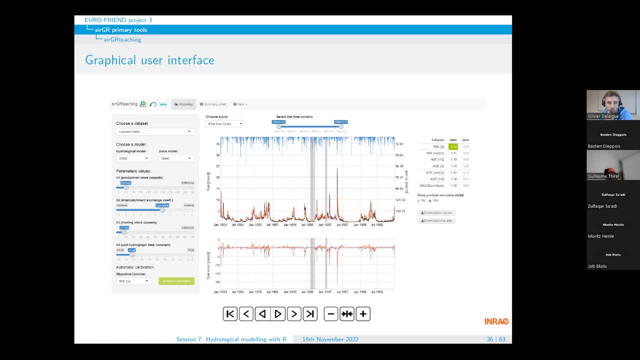 as you launch it from r. you can put from r. you can put from r. you can put your own data, your own data, your own data with, without any problems. you can see with, without any problems. you can see with, without any problems. you can see, here on the left, a panel where you 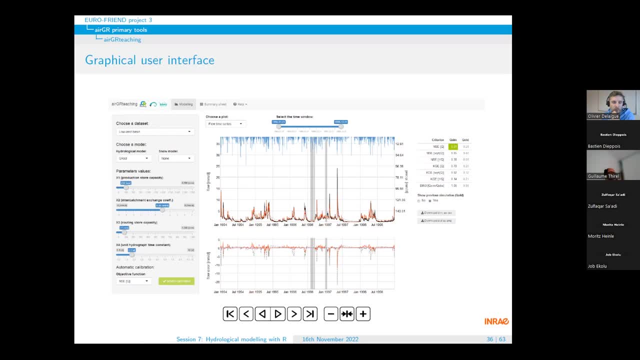 here on the left, a panel where you here on the left, a panel where you choose your catchment. if you have a, choose your catchment. if you have a, choose your catchment. if you have a list list- list of time series- you can choose your model. 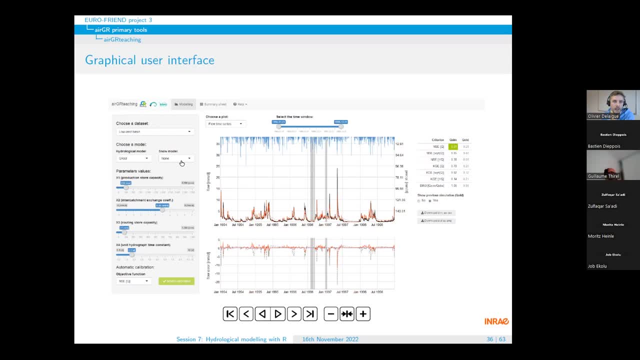 of time series. you can choose your model of time series, you can choose your model between, between between the daily and the monthly model, the daily and the monthly model, the daily and the monthly model, and you can and you can and you can activate, activate, activate or not the snow model. 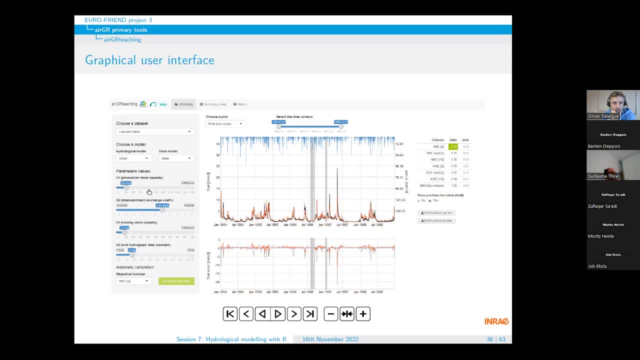 or not the snow model or not the snow model, you can, you can. you can set the different parameter value, set the different parameter value, set the different parameter value, and, and, and. it changed on the central panel, so on. it changed on the central panel, so on. it changed on the central panel. so on the central panel, you can see. 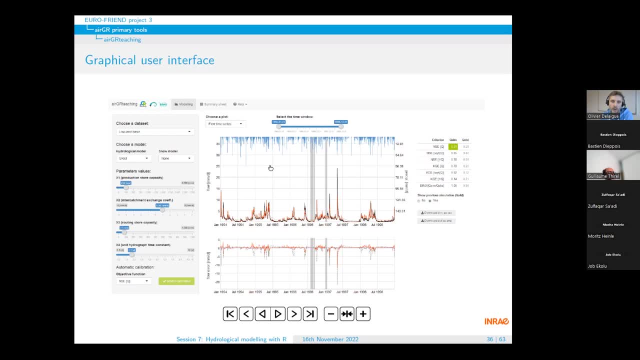 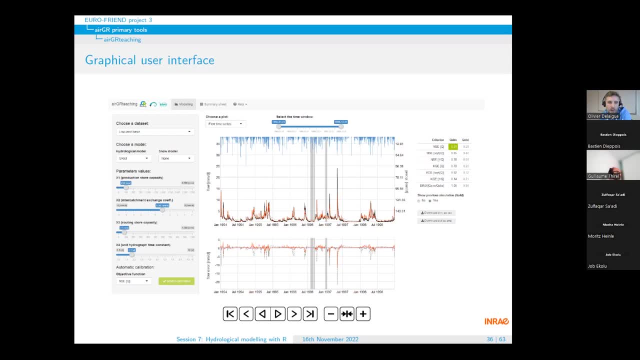 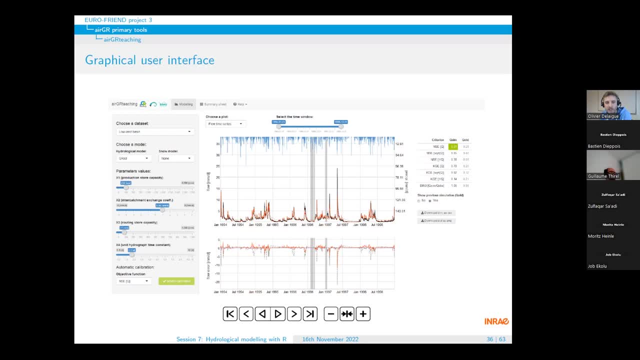 move the slider on the left panel, it will change. it will change. it will change the simulated stream flow so you can see the simulated stream flow. so you can see the simulated stream flow, so you can see in real time, in real time, in real time, the effect. 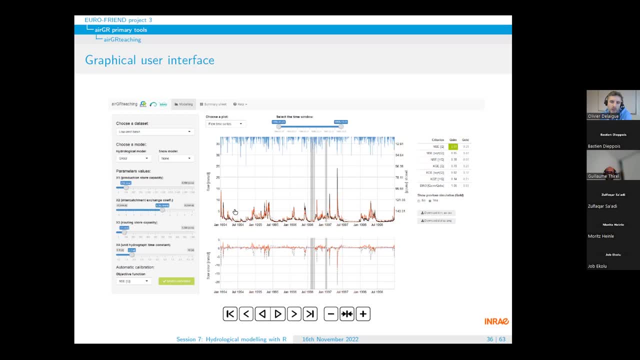 the effect, the effect, the different parameters, the different parameters, the different parameters. besides, you have the error of the. besides, you have the error of the. besides, you have the error of the model, model, model, on each time, on each time, on each time, time, step time, step, time, step. on the right, you have the. 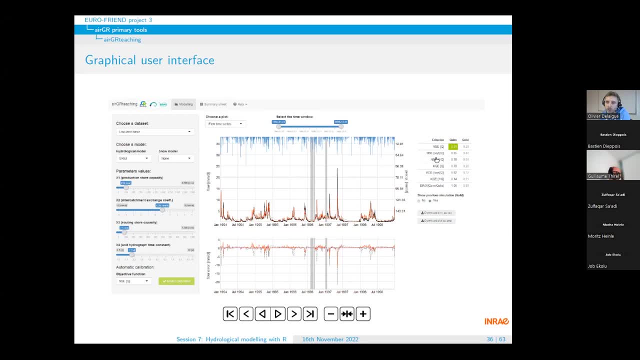 on the right. you have the on the right. you have the criterion values of the criterion values, of the criterion values of the nash and the kge nash and the kge. nash and the kge on the display time series so you can simulate the stream flow. it's 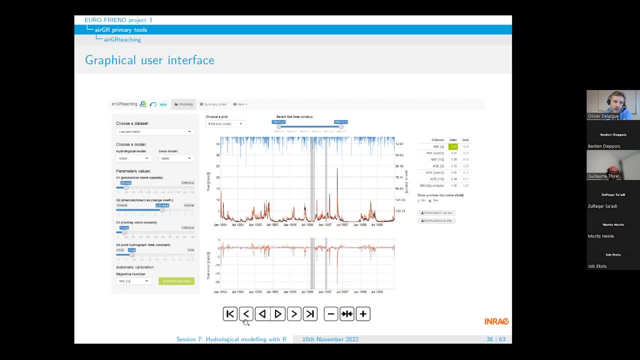 so you can simulate the stream flow. it's so you can simulate the stream flow. it's also possible to calibrate, also possible to calibrate, also possible to calibrate the model. so, on the on the left, you the model. so on the on the left, you. 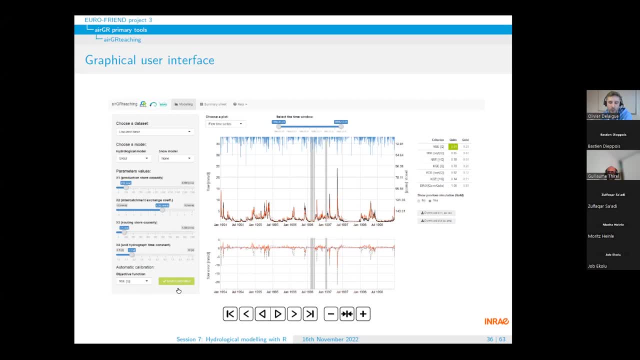 the model. so, on the on the left, you have the green button, have the green button, have the green button and if you click on this button, you can, and if you click on this button, you can, and if you click on this button, you can calibrate the model. 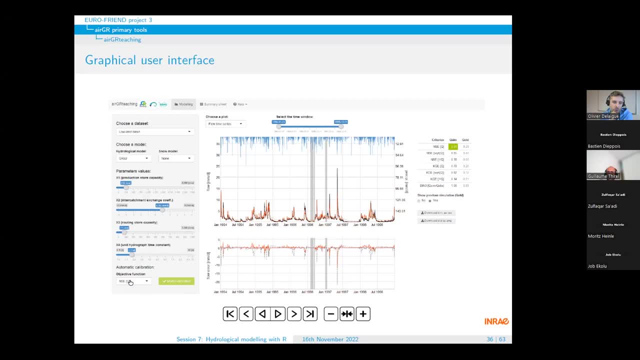 calibrate the model. calibrate the model using a setting objective function. so using a setting objective function, so using a setting objective function, so you can choose between the nash and the, you can choose between the nash and the, you can choose between the nash and the kge. 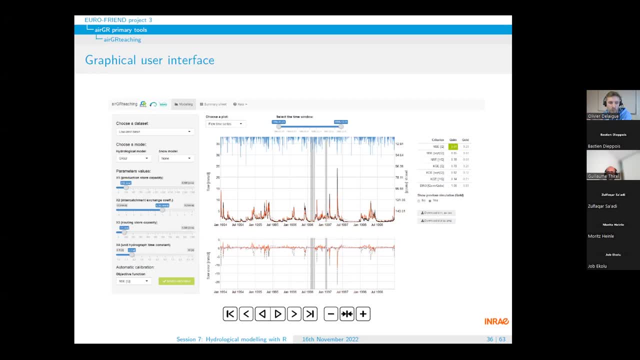 kge, kge, and you can apply it on and you can apply it on, and you can apply it on raw stream flows, or on raw stream flows, or on raw stream flows, or on on transform and stream flow as a, on transform and stream flow as a. 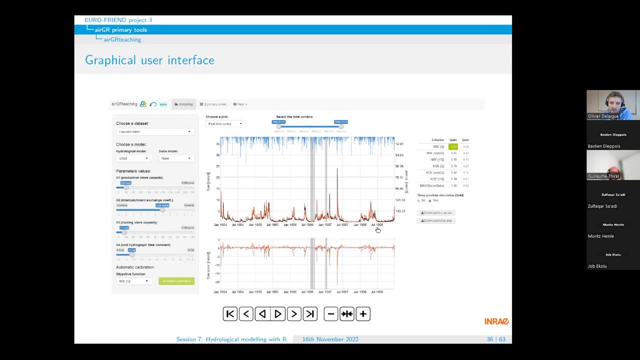 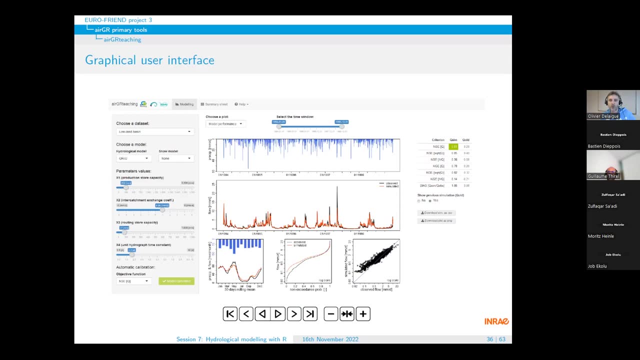 on transform and stream flow as a: the square root string flows, for example. the square root string flows, for example, the square root string flows, for example. so this is the main panel. so this is the main panel. so this is the main panel. you have also different graphics so you can analyze your results. 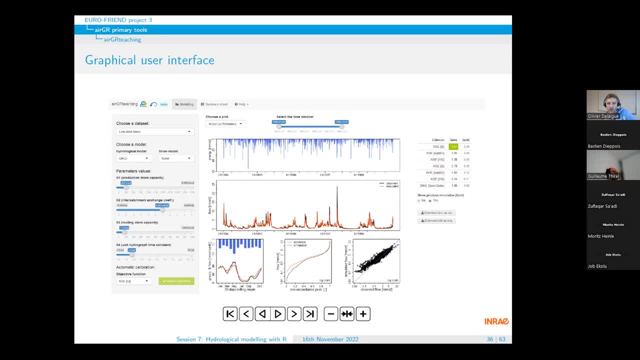 you have also different graphics so you can analyze your results. you have also different graphics so you can analyze your results, displaying the- the regime of the. so you can analyze your results. displaying the- the regime of the. so you can analyze your results. displaying the- the regime of the precipitation as the stream flows. 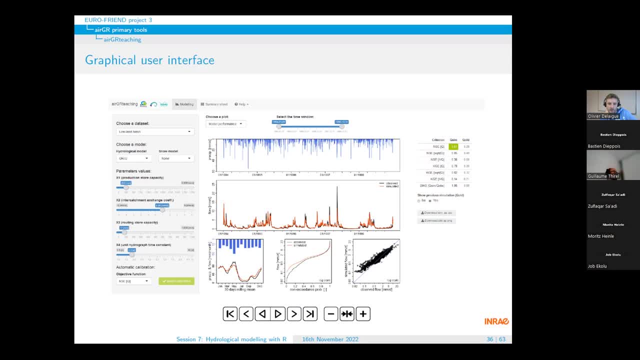 the relation between the simulated and the, the relation between the simulated and the, the relation between the simulated and the observed observed, observed flows and also the. the stream flows are ordered by by values. the stream flows are ordered by by values. the stream flows are ordered by by values. so you can see if your model is is quite 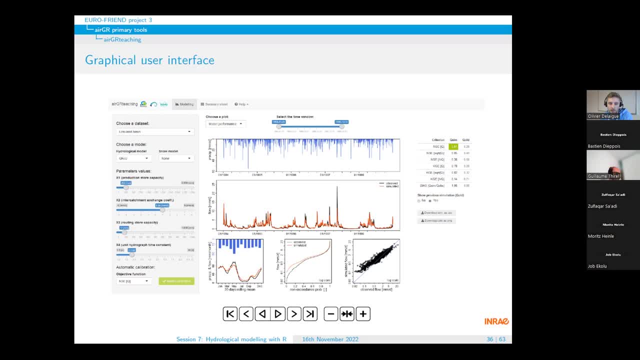 so you can see if your model is is quite. so you can see if your model is is quite correct or not with this graphical output and with the criterion on output, and with the criterion on output, and with the criterion on the right- the right, the right panel. 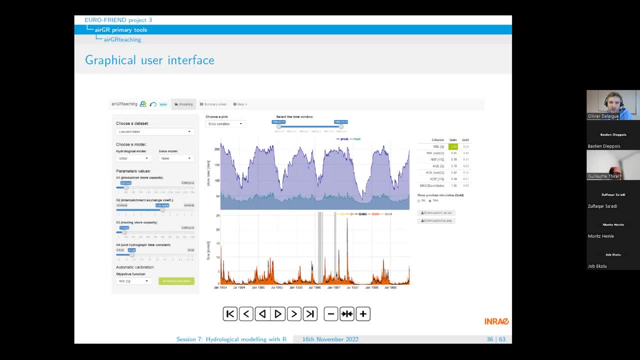 panel panel. you can also have a look. you can also have a look, you can also have a look of the state variables of the state variables of the state variables of the models as store levels of the models, as store levels of the models, as store levels, and the different fluxes. 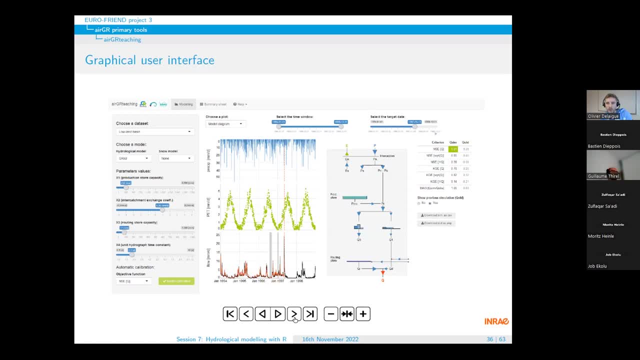 and the different fluxes and the different fluxes and finally, it's also possible, and finally, it's also possible, and finally, it's also possible to have a look of the different fluxes, to have a look of the different fluxes, to have a look of the different fluxes inside. 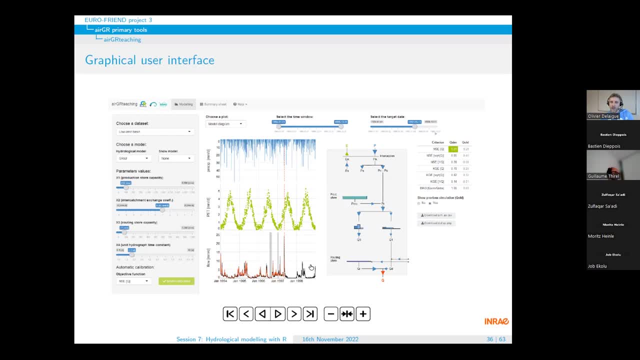 inside, inside the diagram of the model, the diagram of the model, the diagram of the model, and you can see here and you can see here and you can see here the production store, the production store, the production store and the routing store, and the routing store and the routing store at a setting. 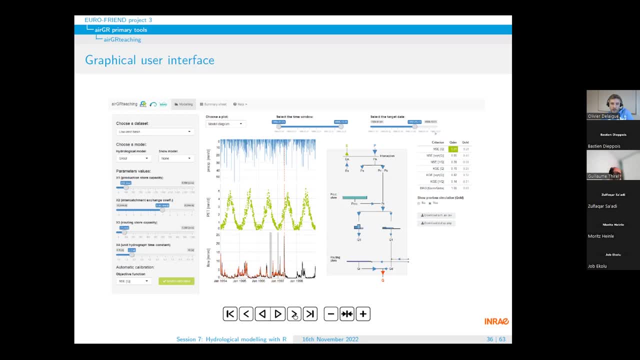 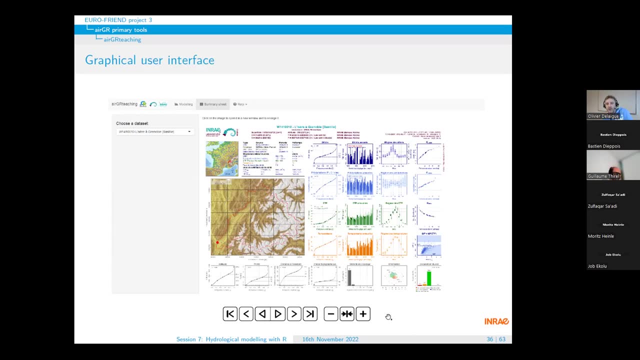 at a setting, at a setting date, if you, if you, if you have some french catchment, it's also have some french catchment, it's also have some french catchment. it's also possible to have an overview, possible to have an overview, possible to have an overview of the. 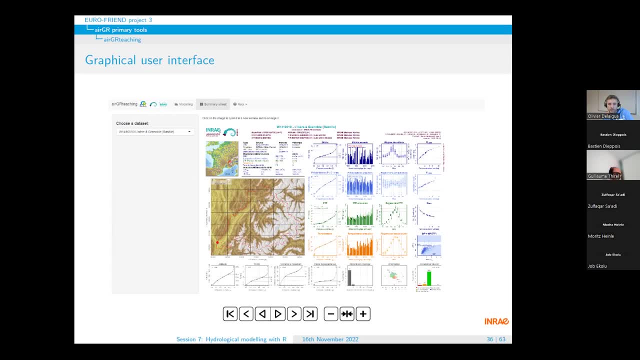 of the of the of a summary of the data. so it's a of a summary of the data. so it's a of a summary of the data. so it's a graphical overview. graphical overview, graphical overview, but it's only available for french. but it's only available for french. 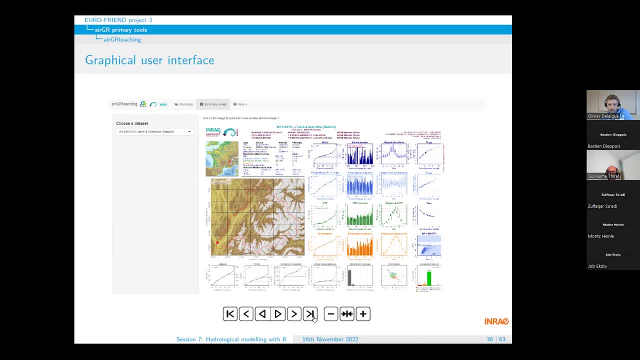 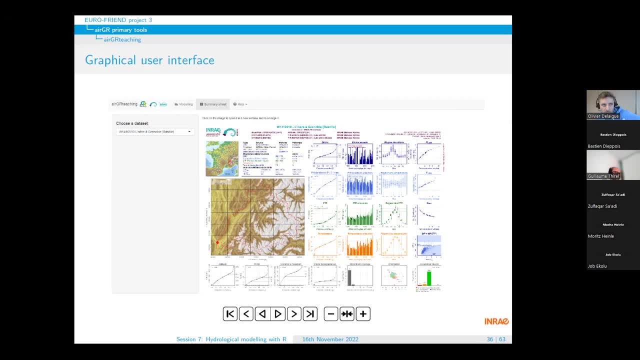 graphical user interface from ara or ara or ara. or. there is a demo on the web with. there is a demo on the web with. there is a demo on the web with: quantity with two catchment quantity with two catchment quantity with two catchment time series. 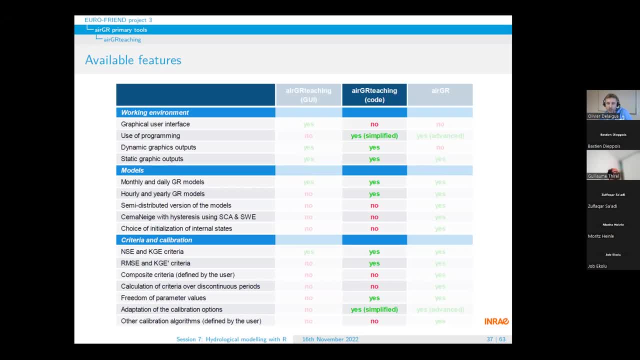 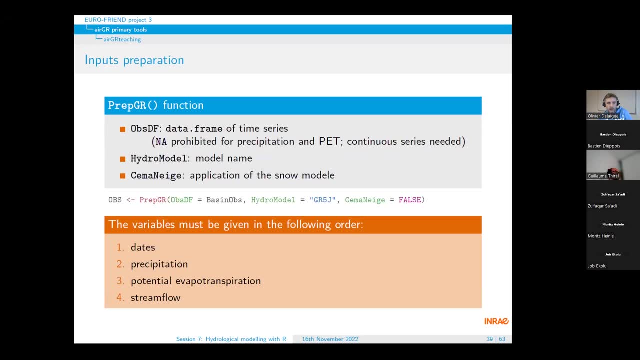 it's also possible to run rgr teaching. it's also possible to run rgr teaching. it's also possible to run rgr teaching using very simple code, using very simple code, using very simple code. so you need exactly the same data. so you need exactly the same data. 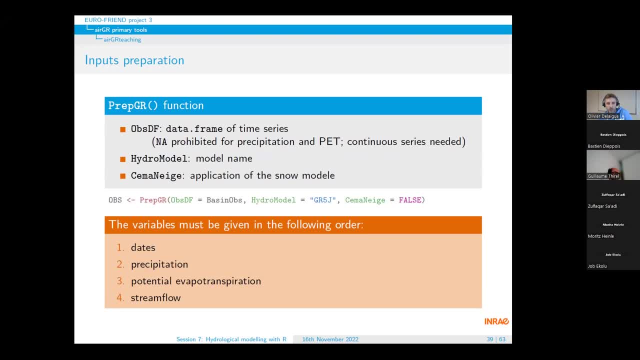 so you need exactly the same data and there is one function to prepare, and there is one function to prepare and there is one function to prepare the data. so you give your time series, the data, so you give your time series, the data, so you give your time series and you 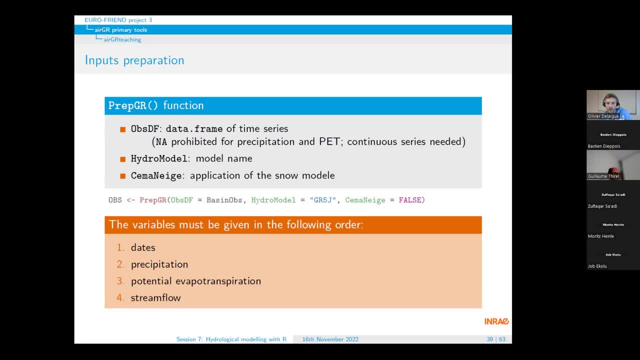 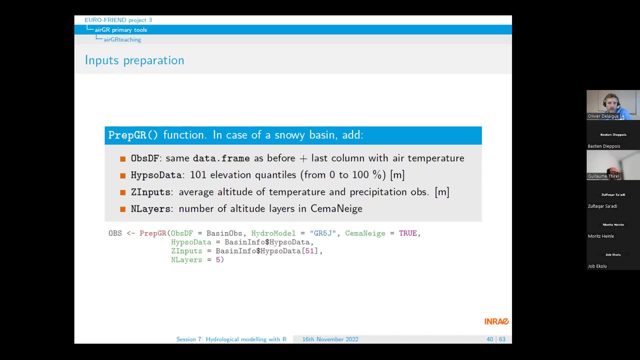 and you and you set the model you want to use and if you set the model you want to use and if you set the model you want to use and if you want to use the snow model or not want to use the snow model or not want to use the snow model or not, so it's a prep gr function after that. 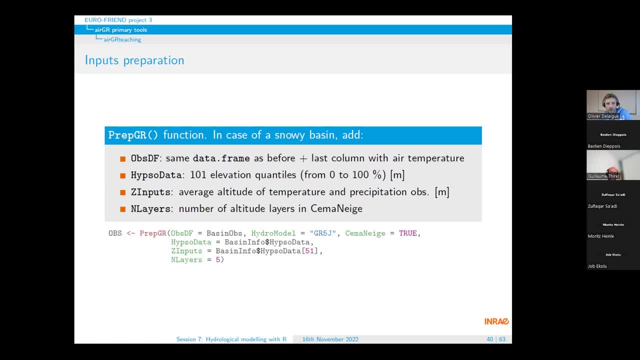 so it's a prep gr function after that. so it's a prep gr function after that: uh, yeah, it's the same. if you want to uh, yeah, it's the same. if you want to uh, yeah, it's the same. if you want to apply the snow model. 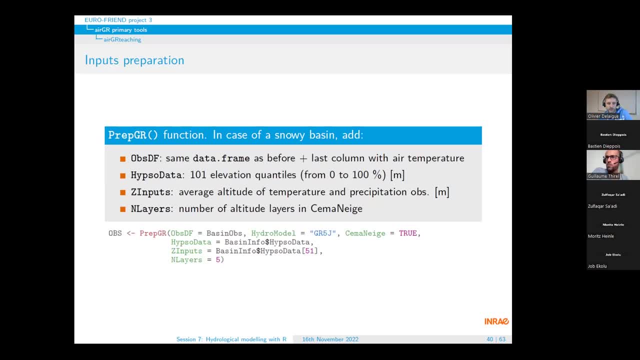 apply the snow model. apply the snow model. you need the, you need the. you need the hypsometric data, hypsometric data, hypsometric data. you can have a look, you can have a look, you can have a look on your time series just using the plot. 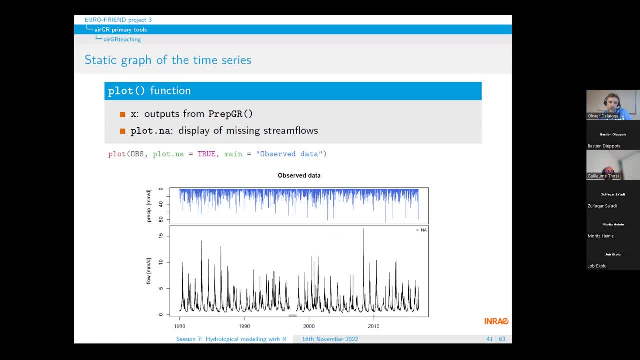 on your time series just using the plot on your time series, just using the plot function. on. on the up on the output of function. on on the up on the output of function. on on the up on the output of the prep gr function: the prep gr function. 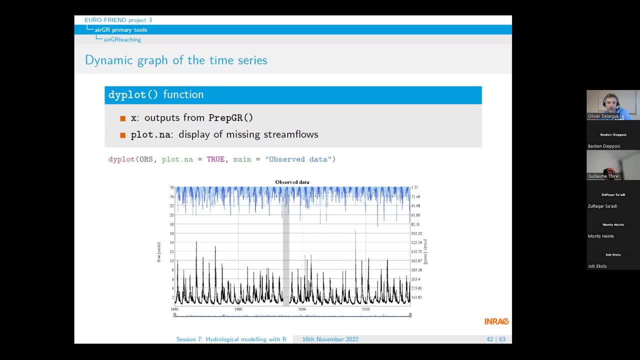 the prep gr function. so it's a static one. it's also possible, so it's a static one. it's also possible, so it's a static one. it's also possible to have a dynamic one and to zoom on and to have a dynamic one and to zoom on, and. 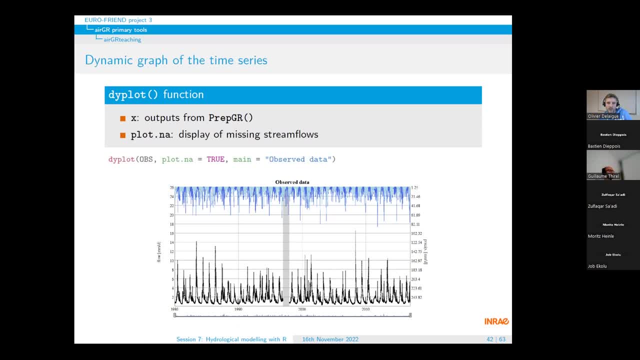 to have a dynamic one and to zoom on and to to to move the mouse on and to read the move the mouse on and to read the move the mouse on and to read the values of the data, values of the data, values of the data, and after that you can calibrate your. 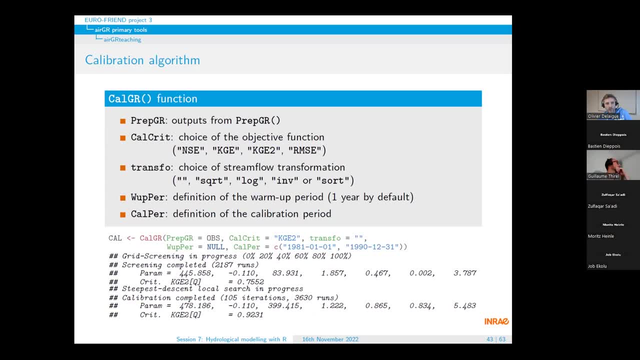 and after that you can calibrate your, and after that you can calibrate your model using the card gr function. so you model using the card gr function, so you model using the card gr function so you can set a warmer period and you have to, can set a warmer period and you have to. 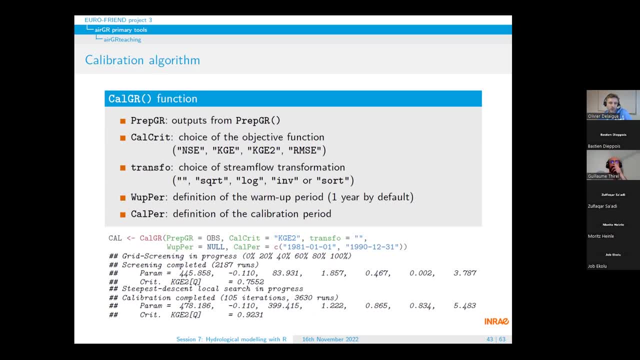 can set a warmer period and you have to set, set, set a simulated period, and in one second you a simulated period, and in one second you a simulated period, and in one second you have the result, have the result, have the result of your calibration. so we have the set. 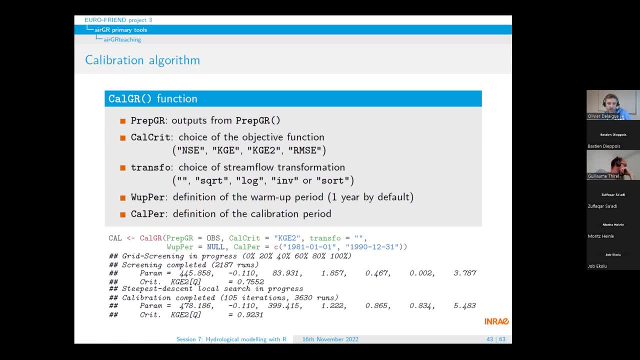 of your calibration. so we have the set of your calibration. so we have the set of the parameters and the value of your. of the parameters and the value of your. of the parameters and the value of your criterion, criterion, criterion: you can also have some graphical outputs. you can also have some graphical outputs. 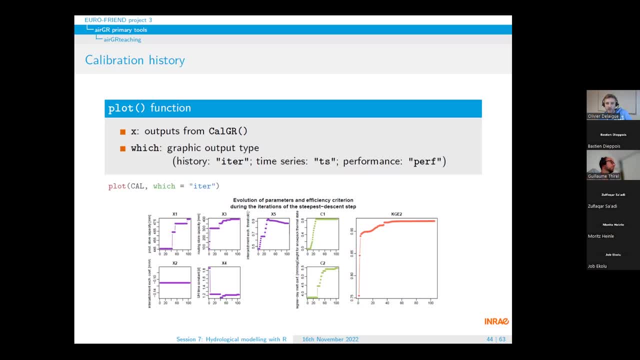 you can also have some graphical outputs as the evolution of the parameter, as the evolution of the parameter, as the evolution of the parameter during the iteration of the calibration, during the iteration of the calibration, during the iteration of the calibration. you can have a. you can have a. 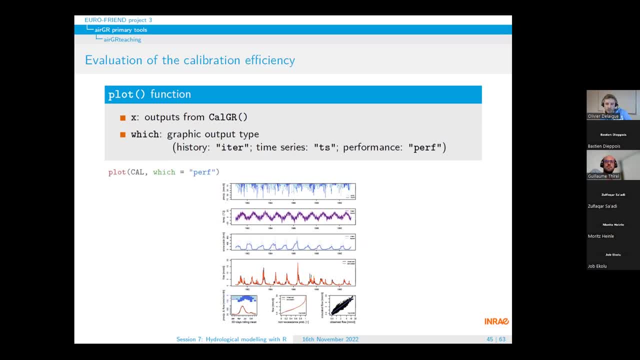 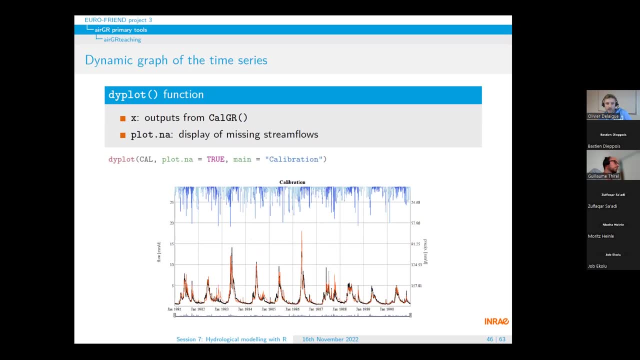 you can have a summary plot to analyze summary plot. to analyze summary plot, to analyze the calibration results, the calibration results, the calibration results, and you can also display the time. and you can also display the time and you can also display the time series with a static or dynamic. 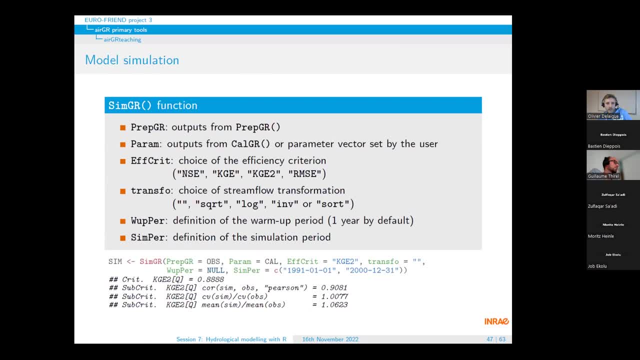 series with a static or dynamic series, with a static or dynamic graphics. if you want to evaluate, if you want to evaluate, if you want to evaluate your, your model on another period- you your your model on another period. you your your model on another period. you can use the sim jar function. you give. 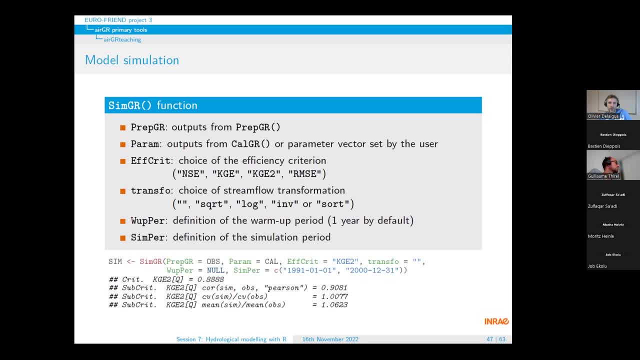 can use the sim jar function you give, can use the sim jar function. you give the time series, the time series, the time series, the set of parameter you want to test and the set of parameter you want to test and the set of parameter you want to test and you can. 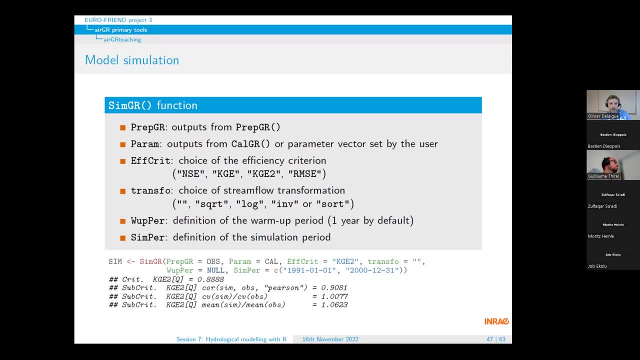 you can. you can simulate your stream flows, simulate your stream flows, simulate your stream flows, and you can evaluate it, and you can evaluate it and you can evaluate it, choosing your criterion and your choosing your criterion and your choosing your criterion. and your transformation: transformation, transformation, as previously. 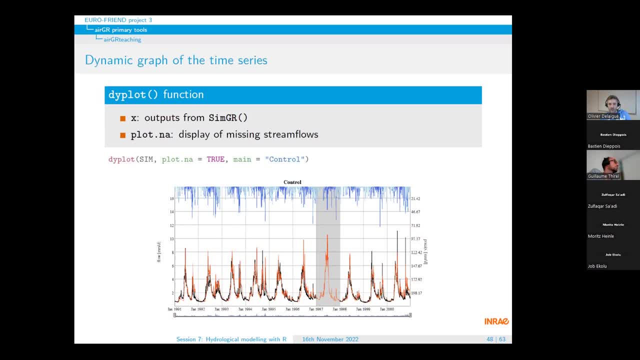 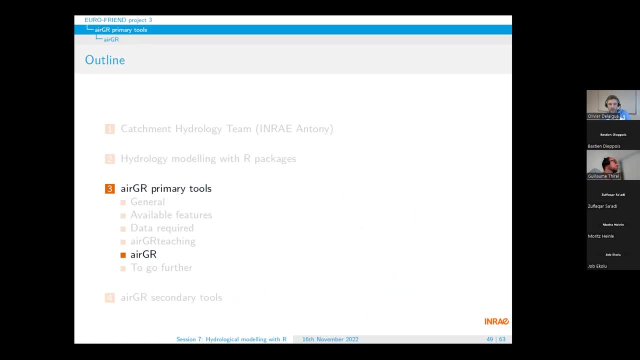 as previously, as previously, and you also have some, and you also have some, and you also have some graphical outputs. i will not detail, i will not detail, i will not detail all the function of the lgr package. because all the function of the lgr package, because 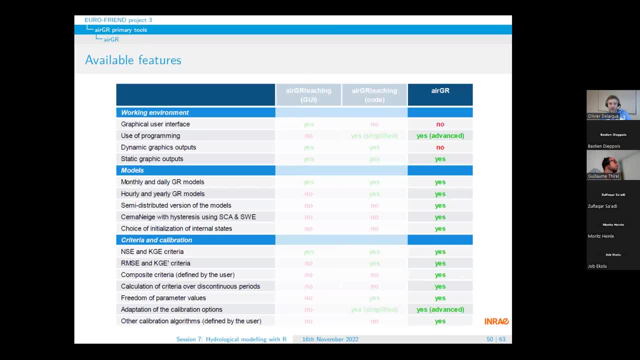 all the function of the lgr package, because there are too many functions, there are too many functions, there are too many functions, but, but, but i just want to focus on the. i just want to focus on the. i just want to focus on the, the fact why. 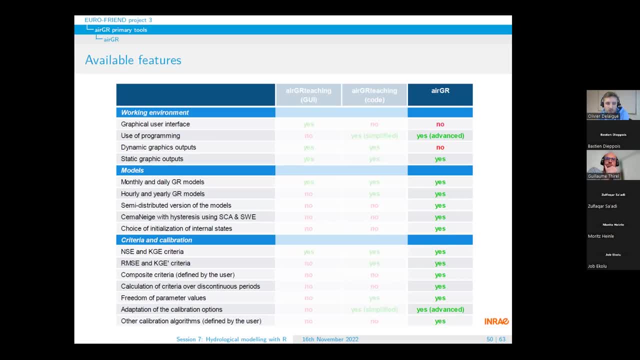 the fact, why the fact? why that? that that you can have the most, you can have the most, you can have the most options using this one options, using this one options, using this one, so you can, for example, use satellite data. so you can, for example, use satellite data. 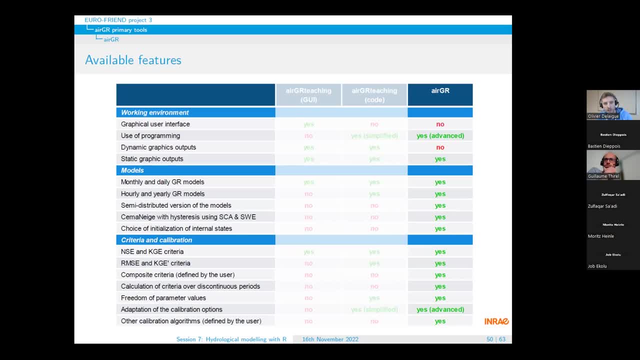 so you can, for example, use satellite data, which is not the case using lgr teaching, which is not the case using lgr teaching, which is not the case using lgr teaching. you can choose the initialization of. you can choose the initialization of. you can choose the initialization of internal states. 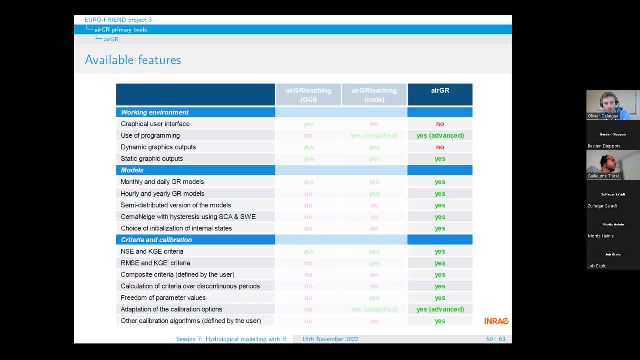 internal states, internal states. using this package, using this package, using this package, you can, you can, you can define your composite criterion, to define your composite criterion, to define your composite criterion. to calibrate, calibrate, calibrate the model, the model, the model. you can, you can, you can calculate a criteria over this continuous. 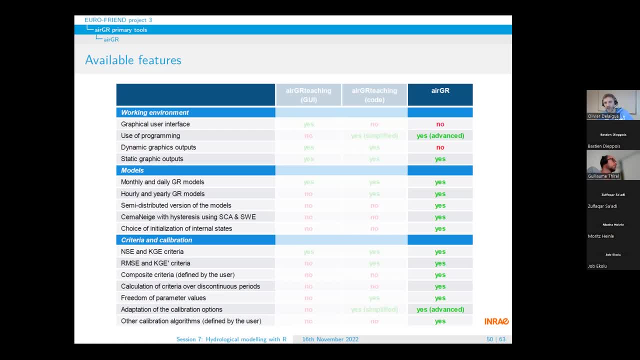 calculate a criteria over this continuous, calculate a criteria over this continuous period, period, period, and so on, so and so on, so and so on. so it's a more complete tools. it's a more complete tools. it's a more complete tools, and just to and just to. 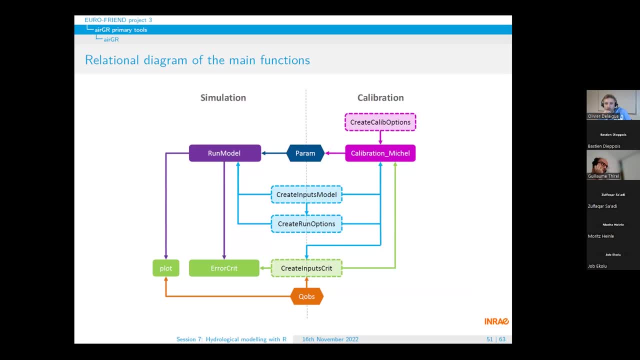 and just to to. to display all the links of the to. to display all the links of the to. to display all the links of the function, function, function. whereas this graph, whereas this graph, whereas this graph, to explain all the links between the. to explain all the links between the. 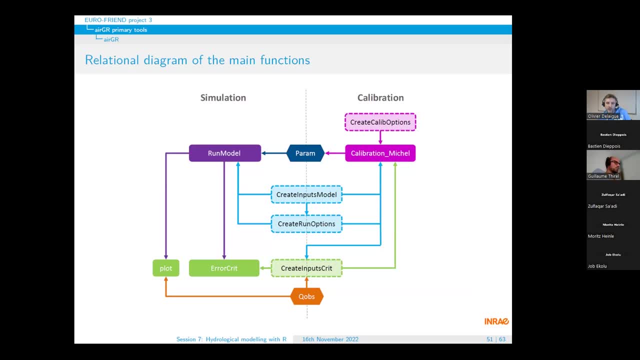 to explain all the links between the features, features, features. so you can see that there there is more. so you can see that there there is more. so you can see that there there is more function, as in rgr teaching function, as in rgr teaching function. as in rgr teaching. so when you start, you you can use rgr. 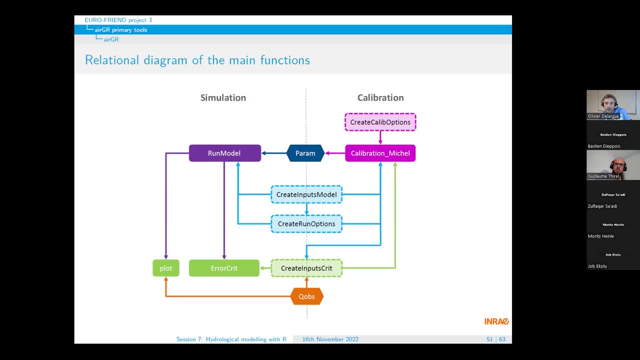 so, when you start you, you can use rgr. so, when you start you, you can use rgr, teaching which is more simple, teaching which is more simple, teaching which is more simple, and you can and you can, and you can use it with all the, use it with all the. 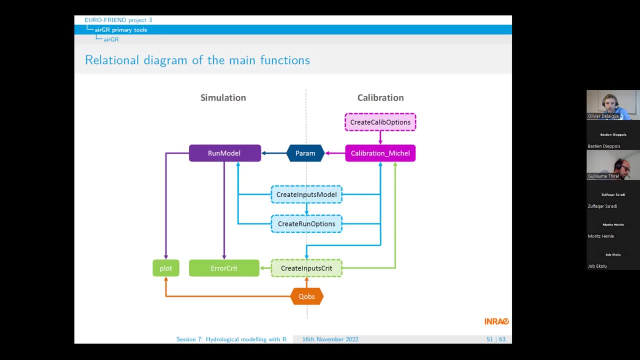 use it with all the the gr models. so it's the gr models, so it's the gr models. so it's quite easy to, quite easy to, quite easy to to taking on and to taking on and to taking on, and maybe more easy to, to start with gr. 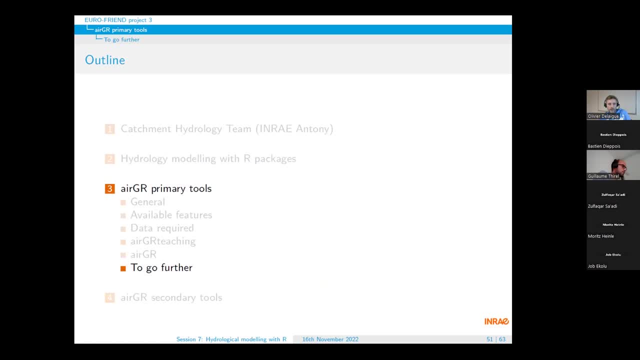 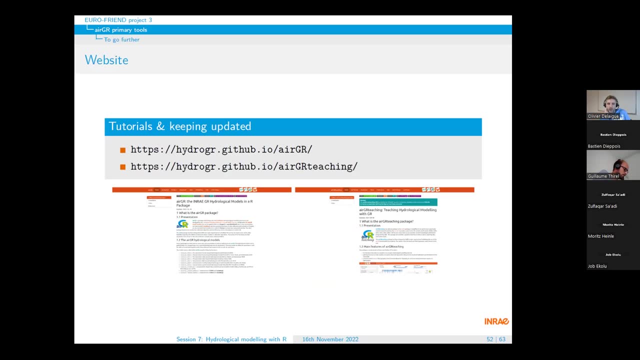 maybe more easy to to start with gr, maybe more easy to to start with gr, models, models and uh. it's also possible to to have some tutorials available in the, to have some tutorials available in the, to have some tutorials available in the web to, for example, to 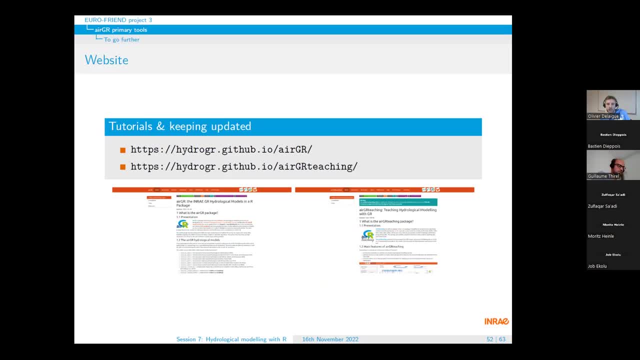 web to, for example, to web to, for example, to. to couple, to couple, to couple another, another, another algorithm to calibrate your model as algorithm to calibrate your model as algorithm to calibrate your model as mcc, for example, mcc, for example mcc, for example, to to. 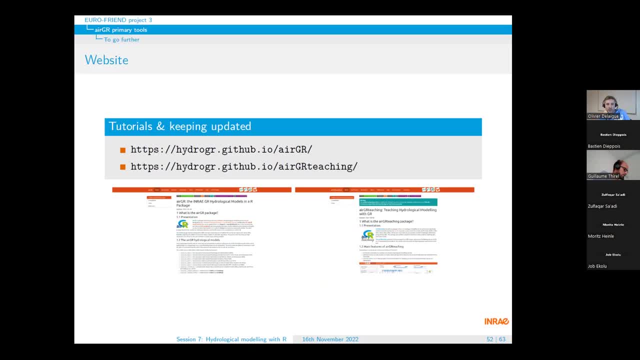 to: to use a semi-distributed, to use a semi-distributed, to use a semi-distributed, semi-distributed version of gr models and semi-distributed version of gr models and semi-distributed version of gr models, and so on, so you can have a look on these. 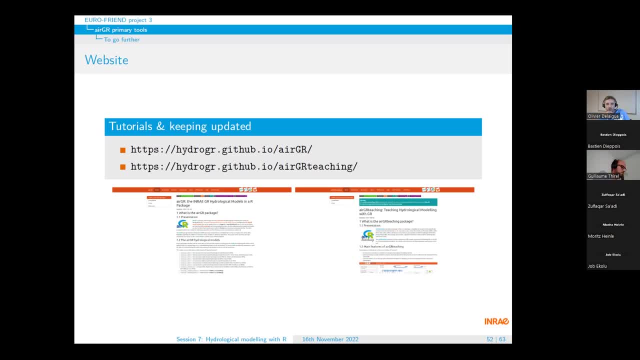 so on. so you can have a look on these, so on. so you can have a look on these two websites, two websites, two websites to get some additional tutorials. and to to get some additional tutorials. and to to get some additional tutorials. and to keeping updated: keeping updated. 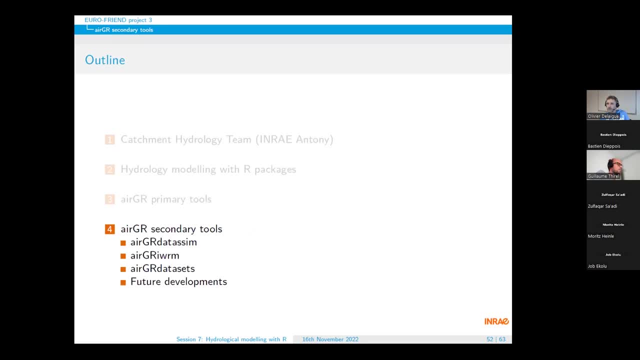 keeping updated of the news of the package. thank you, yes. so just to finish, i will thank you. yes, so just to finish, i will thank you. yes, so just to finish, i will see a couple of see a couple of see a couple of other tools, um, so the first one is: 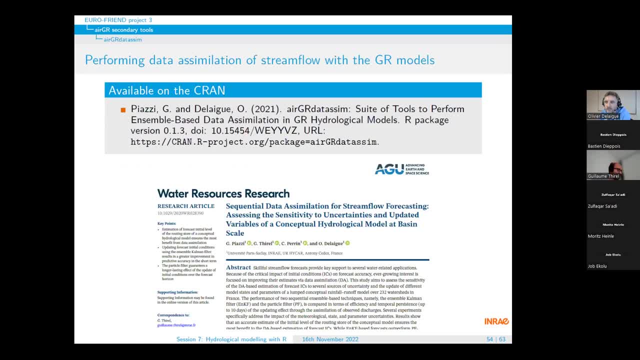 other tools, um. so the first one is other tools, um. so the first one is data sim: um data sim, um data sim, um, yeah, so, yeah, so, yeah, so so this is uh. yeah, i don't assume sorry. so this is uh, yeah, i don't assume sorry. 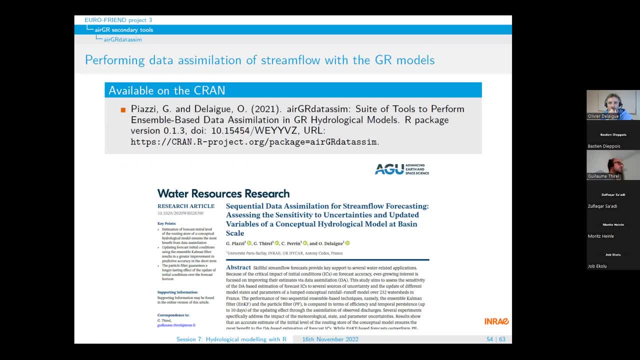 so this is uh, yeah, i don't assume, sorry. uh, so, uh, so, uh. so this package is for data simulation of. this package is for data simulation of. this package is for data simulation of streamflow: streamflow: streamflow within uh- different jr models. within uh- different jr models. 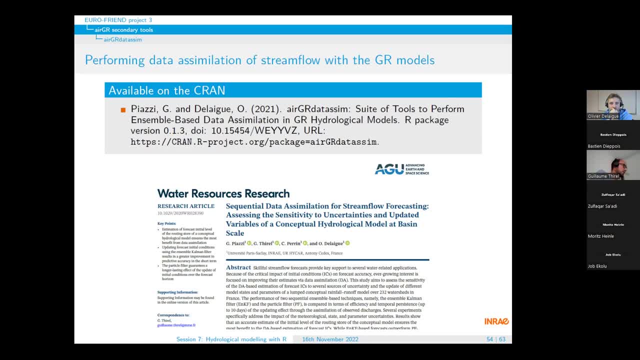 within uh different jr models. so this is a package that was implemented. so this is a package that was implemented. so this is a package that was implemented by olivier and gaia piazzi, by olivier and gaia piazzi, by olivier and gaia piazzi, which is on the crown, and we have a 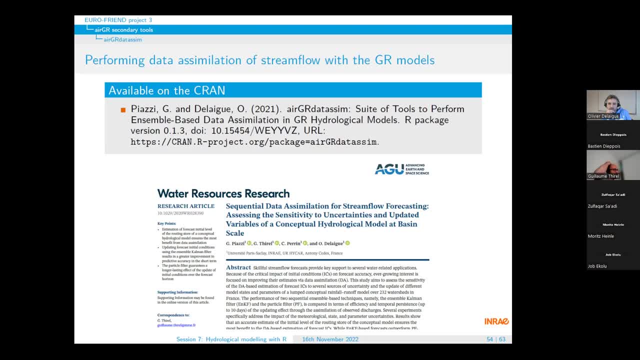 which is on the crown and we have a which is on the crown and we have a paper about the methodology that we paper about the methodology that we paper about the methodology that we we put it into the package which is: uh, we put it into the package which is uh. 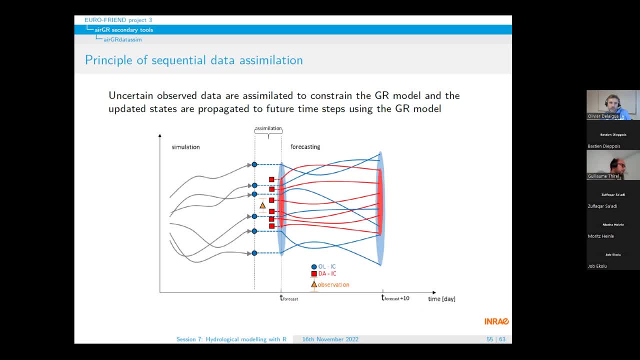 we put it into the package which is: uh, this one in wrr, this one in wrr, this one in wrr. so this package proposes so this package proposes. so this package proposes two methods for sequential data, two methods for sequential data, two methods for sequential data- different. 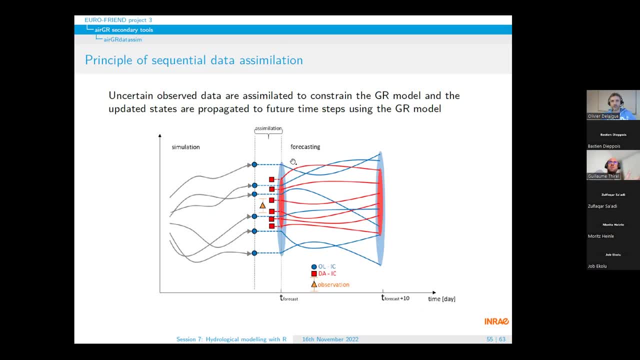 different, different simulation of models. simulation of models. simulation of models based on information you have so observe. based on information you have so observe, based on information you have so observe. data, data, data, and and and the methods we we used, our ensemble. the methods we we used, our ensemble. 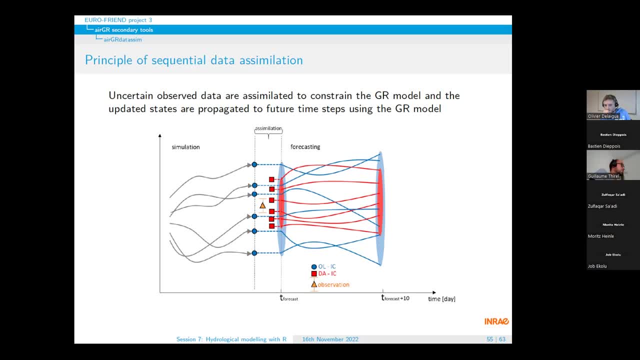 the methods we. we used our ensemble data simulation method. data simulation method. data simulation method. meaning that, um. meaning that, um. meaning that, um. so this is what you, what you have on the. so this is what you, what you have on the. so this is what you, what you have on the on the graph. so you have the gray hours. 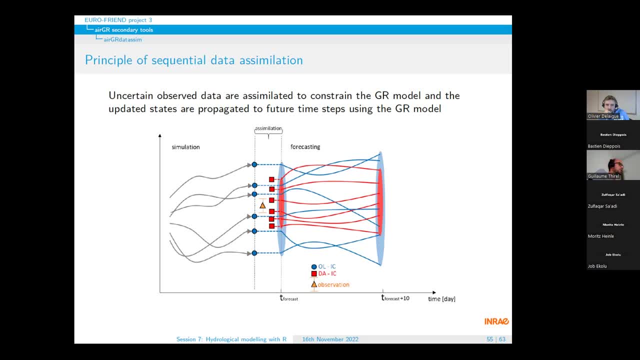 on the graph. so you have the gray hours on the graph. so you have the gray hours with a, with a, with a different simulation, different members, different simulation, different members, different simulation, different members. you arrive at the time step. you arrive at the time step. you arrive at the time step where you have an observation, an. 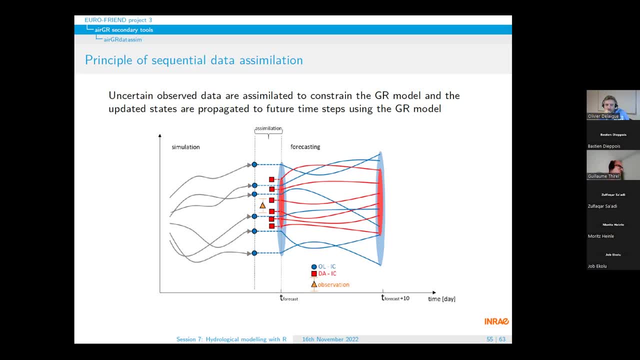 where you have an observation, an where you have an observation, an observation here in the range, with a observation here in the range, with a observation here in the range, with a intensity range, intensity range, intensity range, and, and, and. so you compare your simulations to that. so you compare your simulations to that. 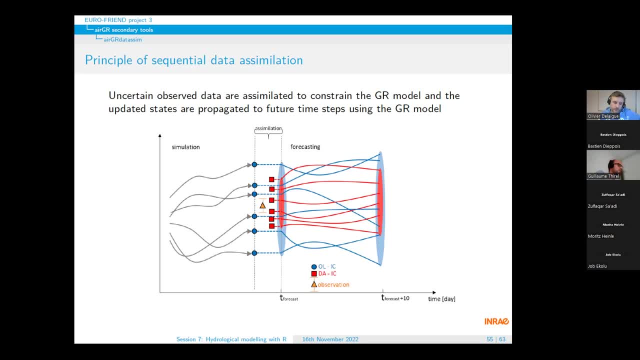 so you compare your simulations to that which gives you an updated, which gives you an updated, which gives you an updated ensemble of ensemble of ensemble of starting point for the next time step, starting point for the next time step, starting point for the next time step, which are the red boxes. 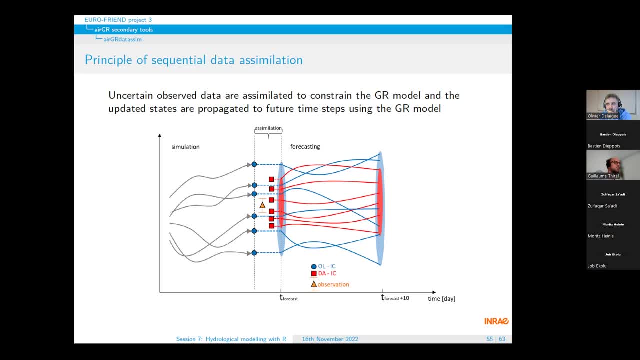 which are the red boxes, which are the red boxes, and you propagate this initial state to, and you propagate this initial state to, and you propagate this initial state to the next, the next, the next time step where you have a time step, where you have a time step where you have a observed data. 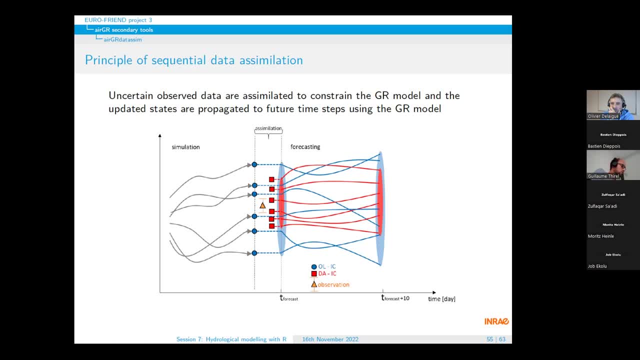 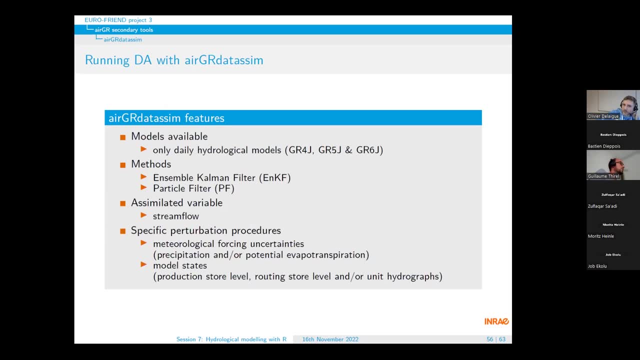 observed data. observed data. so this is very important for, so this is very important for, so this is very important for ideological forecasting, ideological forecasting, ideological forecasting. so this is the basic methodology, so this is the basic methodology. so this is the basic methodology, what we propose in the package. 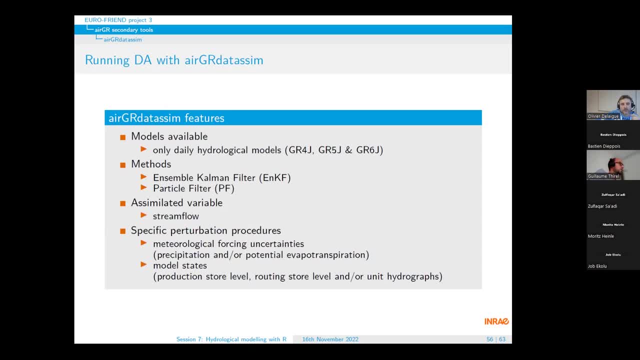 what we propose in the package. what we propose in the package are data streaming methods that work for. are data streaming methods that work for? are data streaming methods that work for three, three, three. daily models: gr4j, gr5j, dr6j. daily models: gr4j, gr5j, dr6j. 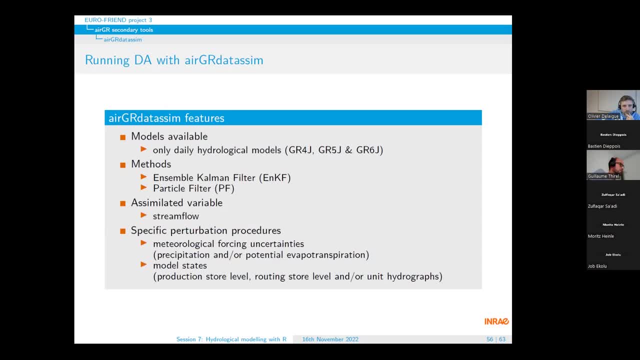 daily models: gr4j, gr5j, dr6j. we have two very classical data. we have two very classical data. we have two very classical data submission methods: the ensemble cameron submission methods, the ensemble cameron submission methods, the ensemble cameron filter filter filter, but also the particle filter. uh, what we 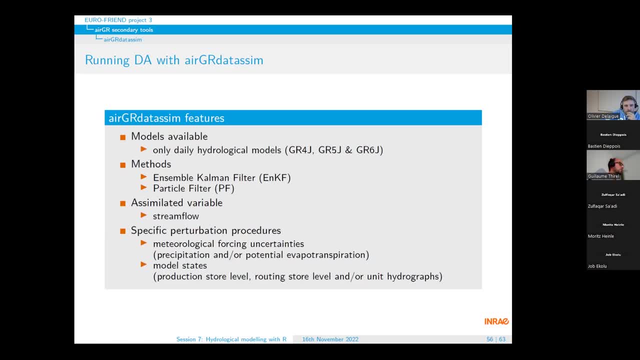 but also the particle filter. uh, what we, but also the particle filter, uh, what we can assimilate is observed stream flow. can assimilate is observed stream flow can assimilate is observed stream flow. and to: to perform the data estimation we. and to to perform the data estimation we. 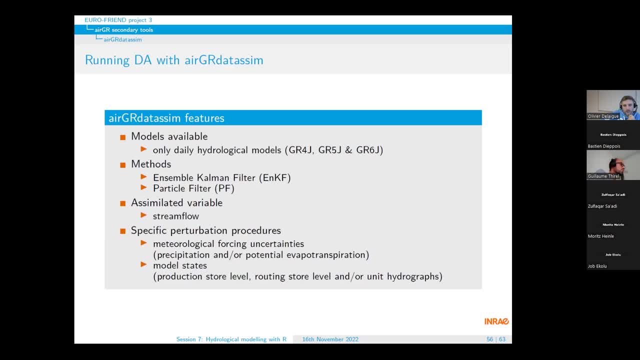 and to to perform the data estimation. we we have some procedures for perturbating different things. perturbating different things, perturbating different things. so first of all uh meteorological, so first of all uh meteorological. so first of all uh meteorological forcing, forcing. 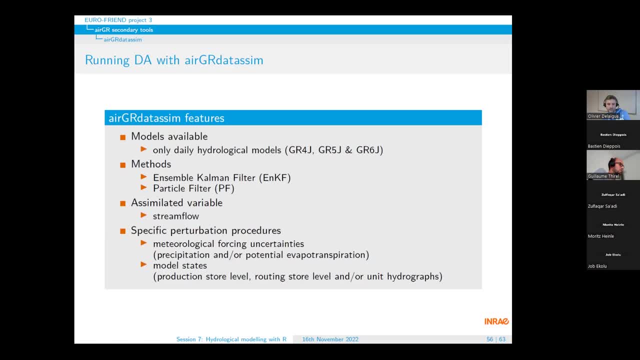 forcing, which is a main uncertainty. so you, you, which is a main uncertainty. so you, you, which is a main uncertainty, so you, you can, can, can perturb precipitation and potential perturb precipitation and potential perturb precipitation and potential evapotranspiration, evapotranspiration. 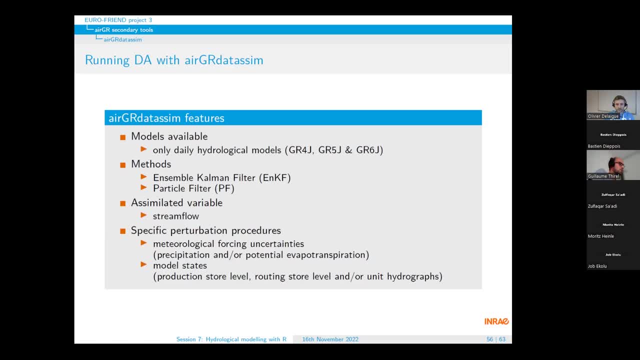 evapotranspiration, evapotranspiration, but you can also perturb a model. but you can also perturb a model. but you can also perturb a model: state, state state. so the different stores in the model of. so the different stores in the model of. 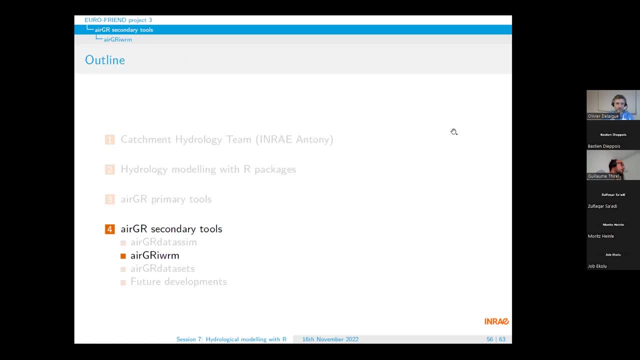 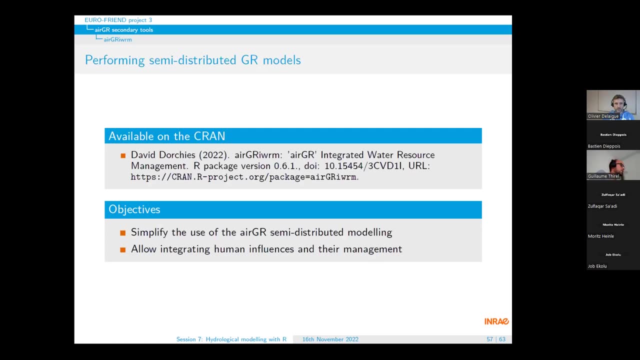 so the different stores in the model of the unit hydrographs um. so the second package we wanted to um. so the second package we wanted to um so the second package we wanted to present is lgr iwrm. present is lgr iwrm. present is lgr iwrm. so iwrm stands for integrated water. 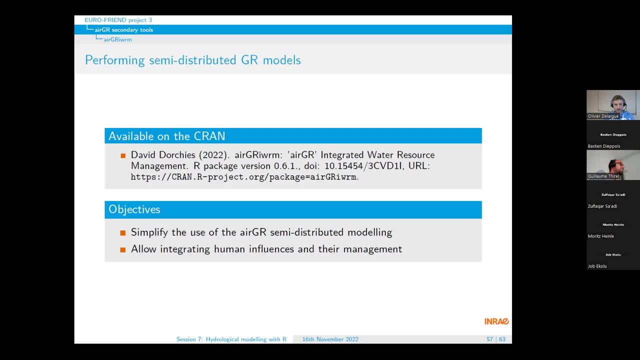 so iwrm stands for integrated water, so iwrm stands for integrated water resources, management resources, management resources, management, um, um, um. so this is also a package that we have on, so this is also a package that we have on, so this is also a package that we have on the crown: uh, developed, developed by a. 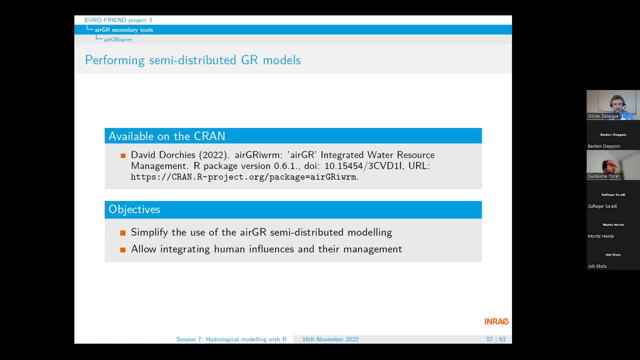 the crown uh developed, developed by a. the crown uh developed developed by a colleague of colleague of colleague of us, david dorshi, which actually uses us, david dorshi, which actually uses us. david dorshi, which actually uses rgr but adds rgr but adds rgr but adds a layer around it to ease. 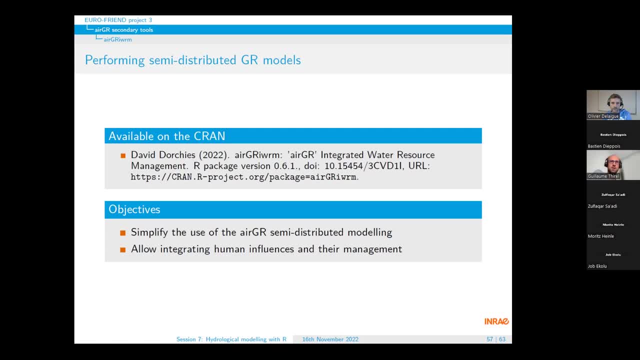 a layer around it to ease a layer around it. to ease it's used for semi-distributed modeling. it's used for semi-distributed modeling. it's used for semi-distributed modeling because performing semi-distributed, because performing semi-distributed, because performing semi-distributed modeling, when you have 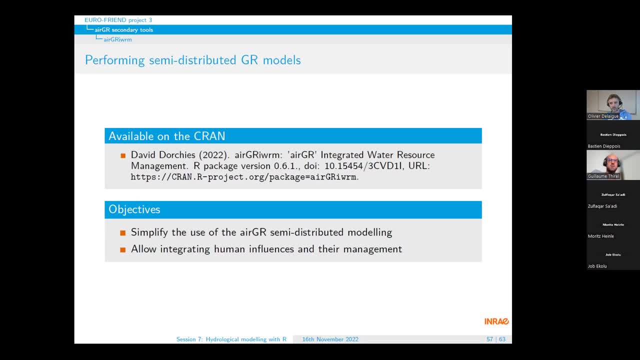 modeling, when you have modeling, when you have one or two basins- upstream is one or two basins, upstream is one or two basins upstream- is quite easy with rgr, but quite easy with rgr, but quite easy with rgr. but when you have a very large basin with 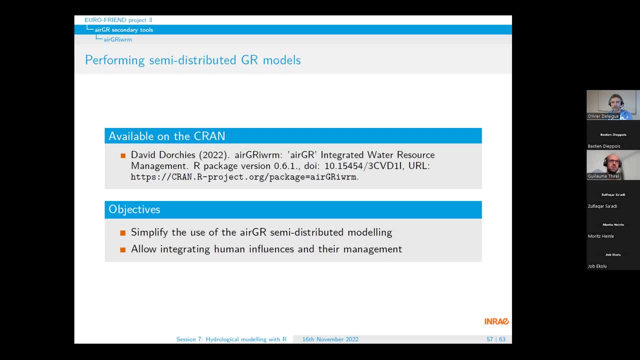 when you have a very large basin, with when you have a very large basin with 100 of catchment flowing into 100 of catchment flowing into 100 of catchment flowing into, into, into the others, it's it can become, into into the others, it's it can become. 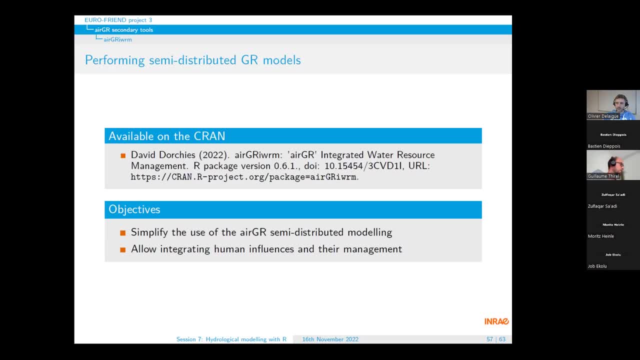 into, into the others it's, it can become very, very, very difficult to to cut that um in this. difficult to to cut that um in this. difficult to to cut that um in this package. we propose a way to just um package. we propose a way to just um. 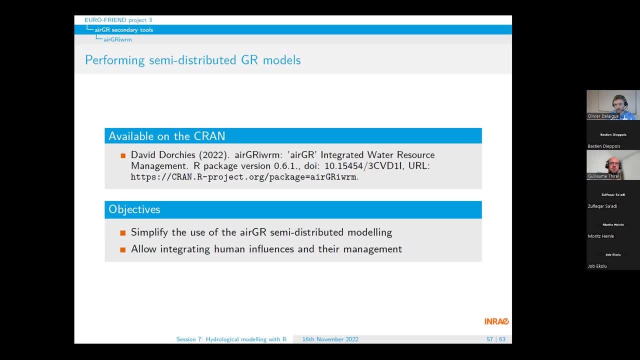 package. we propose a way to just um fill in a data frame and uh fill in a data frame, and uh fill in a data frame, and uh, and, and, and, it, it. it rents. the different functions in the rents. the different functions in the rents: the different functions in the correct order. 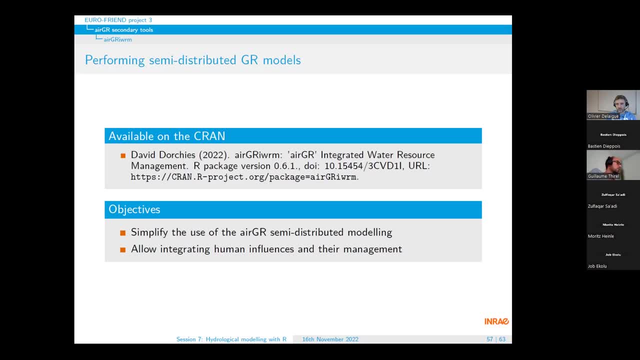 correct order. correct order um. that's why we have integrated water, um. that's why we have integrated water um. that's why we have integrated water. resistance management in the name of the resistance management, in the name of the resistance management, in the name of the package package. 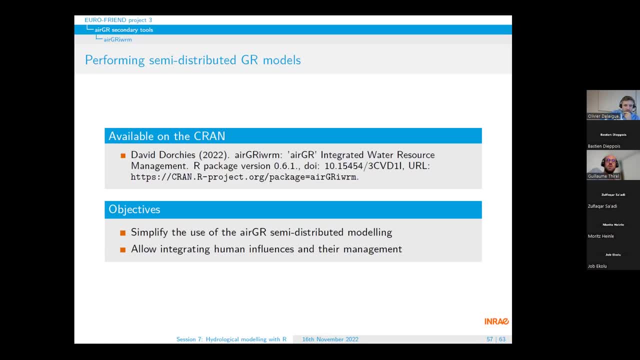 package, so we can do two different things. um so we can do two different things. um so we can do two different things: um integrating, integrating, integrating, integrating, integrating. integrating uses that we know observed uses, so you uses that we know observed uses, so you uses that we know observed uses, so you can inject that or withdraw water, and 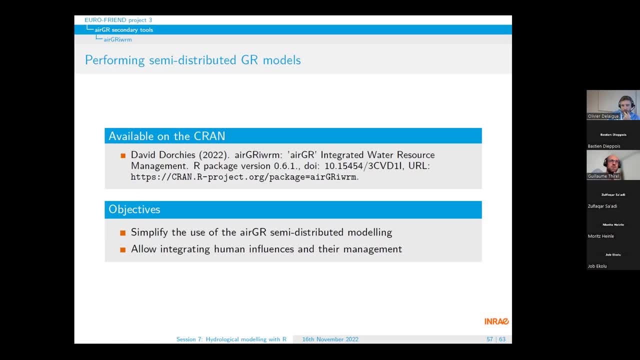 can inject that or withdraw water, and can inject that or withdraw water, and directly, directly, directly, somewhere in the basin where influence is, somewhere in the basin where influence is, somewhere in the basin where influence is. but you can also implement. but you can also implement. but you can also implement water uses, models and. 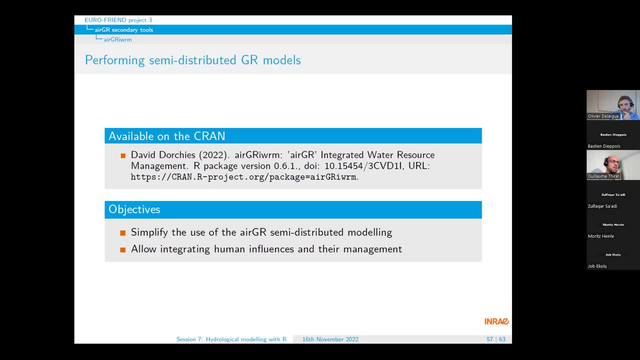 water uses models and water uses models and and the way um the uses are managed and the way um the uses are managed and the way um the uses are managed- if you have a reservoir and so on, if you have a reservoir, and so on, if you have a reservoir, and so on. so this is very useful for 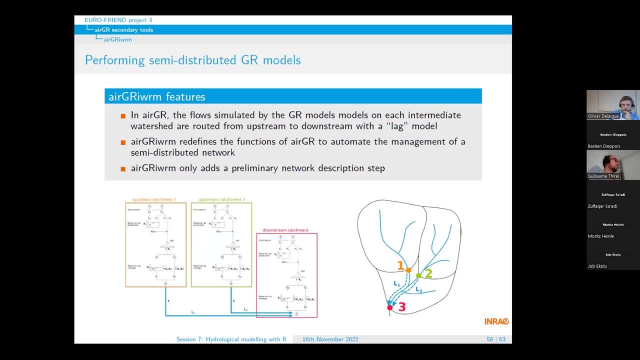 so this is very useful for. so this is very useful for clanmate change and adaptation, clanmate change and adaptation, clanmate change and adaptation methods, methods, methods. so to go into more details, so to go into more details, so to go into more details, what you have in ng, in rgr, is a 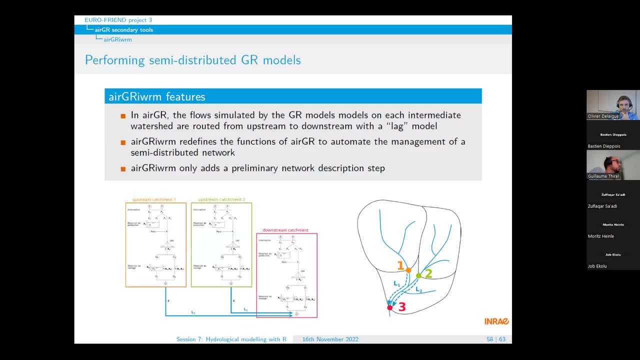 what you have in ng in rgr is a. what you have in ng in rgr is a very simple way to to, very simple way to, to very simple way to to uh to go from upstream to downstream, uh. to go from upstream to downstream. uh. to go from upstream to downstream with a lag model. 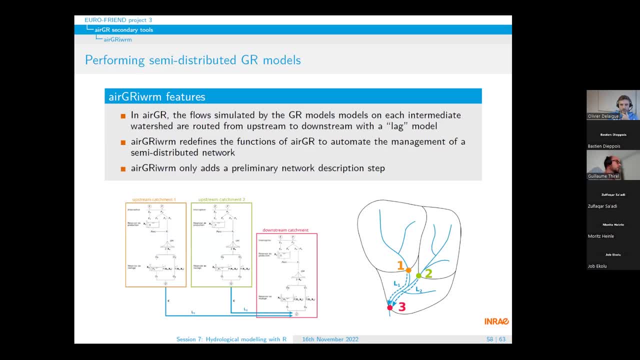 with a lag model, with a lag model in the jar models, in the jar models, in the jar models, and what rgr iwrm proposes is to to and what rgr iwrm proposes is to to and what rgr iwrm proposes is to to automate. 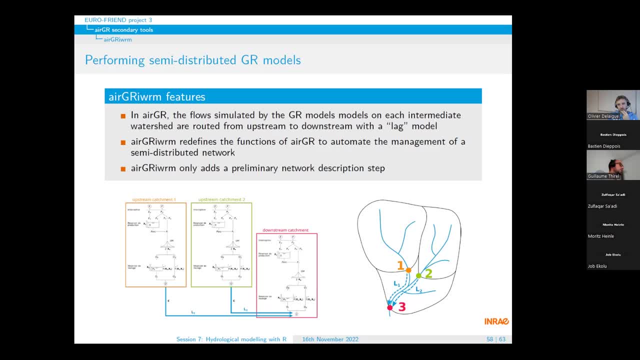 automate, automate the way the semi-distributed network is, the way the semi-distributed network is the way the semi-distributed network is. uh, uh, uh is uh handled. so is uh handled, so is uh handled. so this is what you have, uh on the, on the. 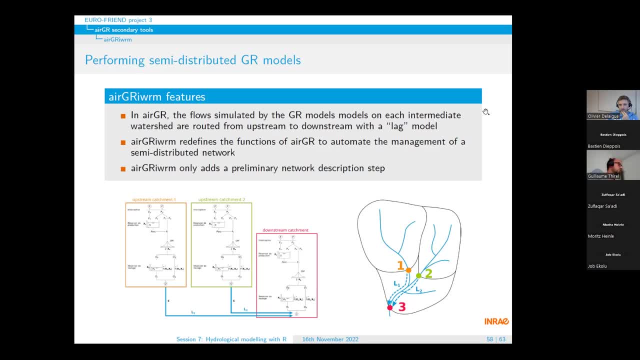 this is what you have uh on the on the. this is what you have uh on the on the bottom of the bottom of the bottom of the, on the slide, on the slide, on the slide. on each upstream catchment, you run. on each upstream catchment, you run. 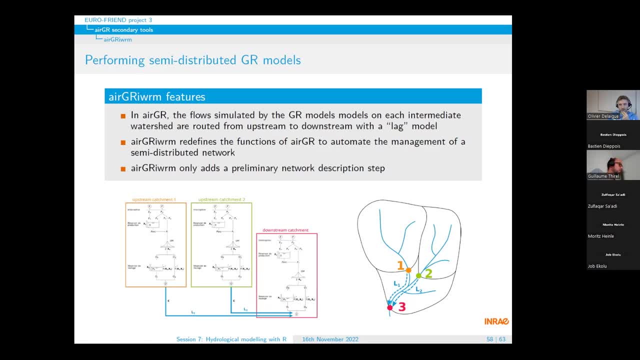 on each upstream catchment, you run, you run a jar model and you take the simulated discharge and you, you take the simulated discharge and you, you take the simulated discharge and you lag it to the, lag it to the, lag it to the output, to the, to the outlet of the. 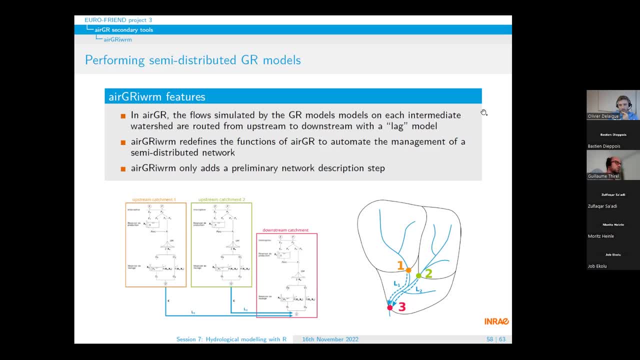 output to the, to the outlet of the output, to the, to the outlet of the downstream catchment, and you add the downstream catchment and you add the downstream catchment and you add the simulation of the downstream part of the simulation of the downstream part of the. 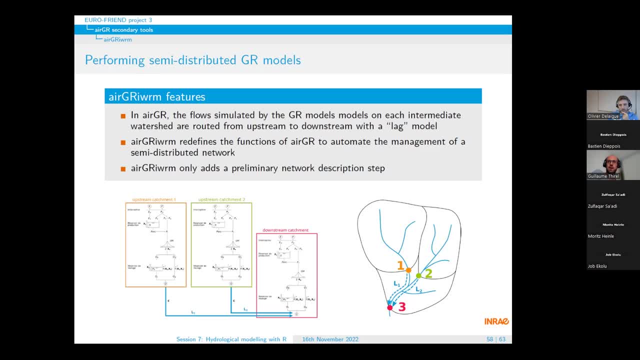 simulation of the downstream part of the catchment to have the total stream flow catchment. to have the total stream flow catchment. to have the total stream flow flowing out of the catchment, flowing out of the catchment, flowing out of the catchment. so you just have to add one function to 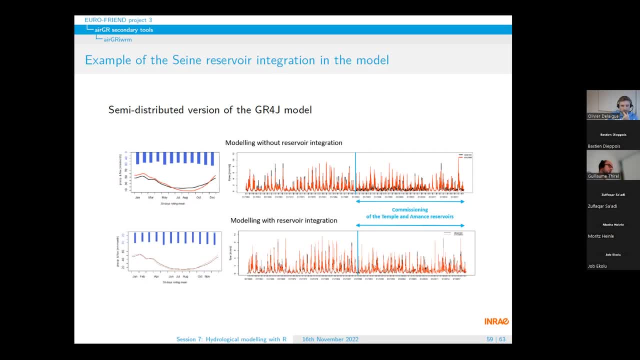 so you just have to add one function to. so you just have to add one function to to run this, to run this, to run this. this is an example of this is an example of this is an example of what you can get, what you can get, what you can get from. 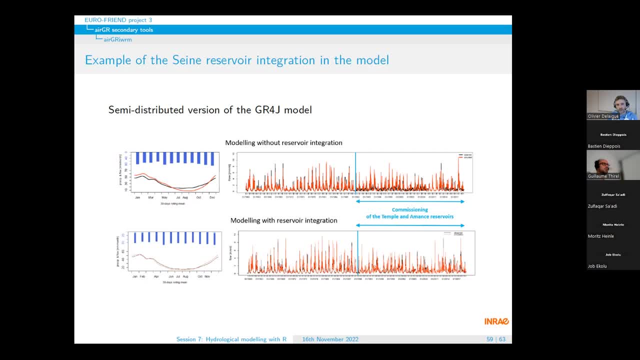 from from running this package. so here we are in running this package. so here we are in running this package. so here we are in the same basin, the same basin, the same basin. so the sand is a river flowing. so the sand is a river flowing. so the sand is a river flowing through paris. 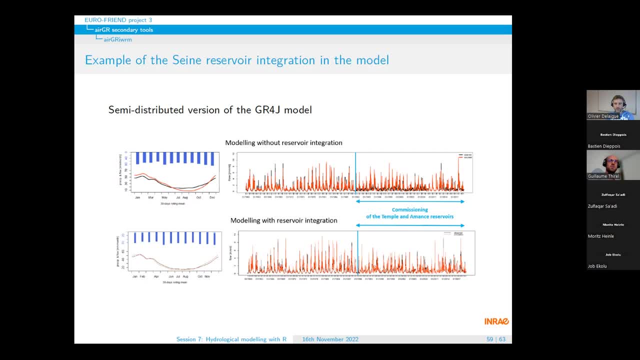 through paris, through paris, very upstream to paris, you have a very, very upstream to paris, you have a very, very upstream to paris. you have a very, very large reservoirs that aim very large reservoirs, that aim, very large reservoirs that aim both at mitigating flows and 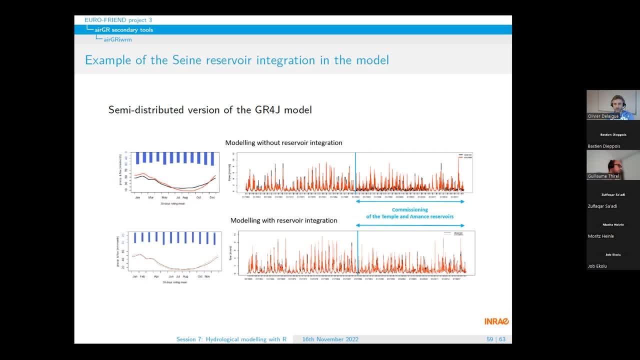 both at mitigating flows and both at mitigating flows, and and also low flows, and also low flows and also low flows. so two different, two opposite objectives. so two different, two opposite objectives. so two different, two opposite objectives. and and and we are lucky, we have very long time. 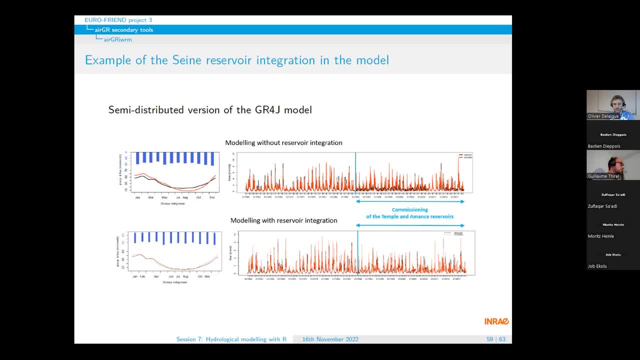 we are lucky, we have very long time. we are lucky, we have very long time. series here and, for example, for series here and for example, for series here and for example, for one tributary, one tributary, one tributary. we have data before and after. 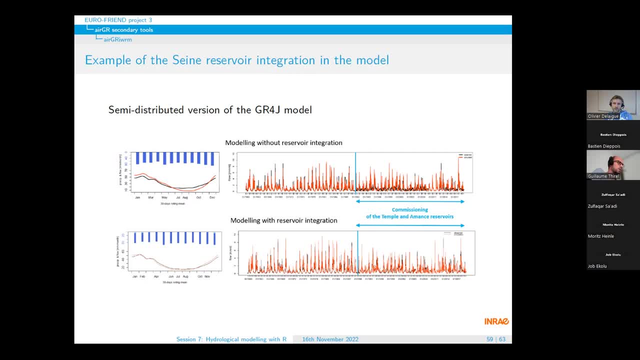 we have data before and after. we have data before and after the building of the building, of the building of two reservoirs, two reservoirs, two reservoirs. so so so you can see on the on the top picture, you can see on the on the top picture. 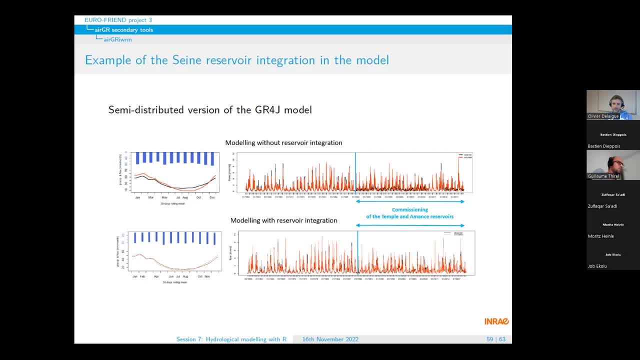 you can see on the on the top picture, that that that you can represent well the time series. you can represent well the time series. you can represent well the time series before the construction in, before the construction in, before the construction in 1990, 1990. 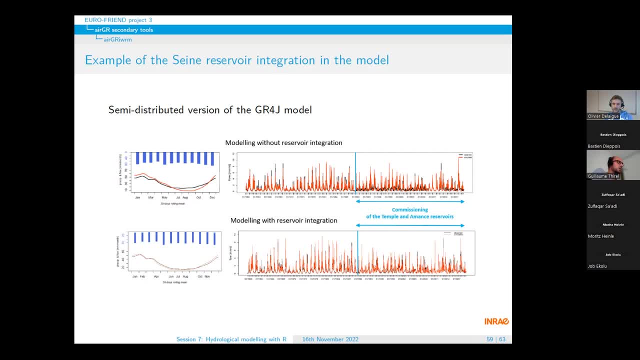 but after the construction, uh just. but after the construction, uh just. but after the construction, uh just. running a gr model is not enough. running a gr model is not enough. running a gr model is not enough because, because, because the seasonal cycle is the seasonal cycle is the seasonal cycle is modified a lot. and if you, if you plot the, 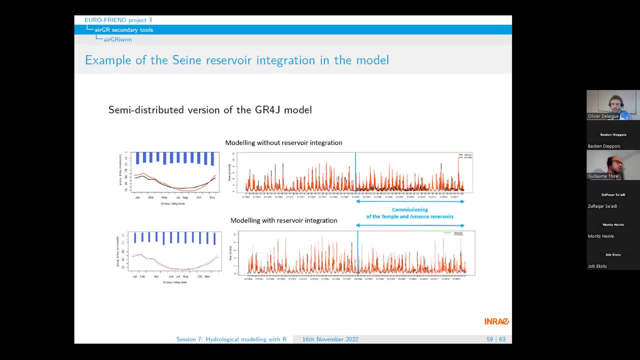 modified a lot. and if you, if you plot the modified a lot, and if you, if you plot the rich, rich, rich seasonal cycle, you, you can see that very seasonal cycle. you, you can see that very seasonal cycle. you, you can see that very easily, you, easily, you. 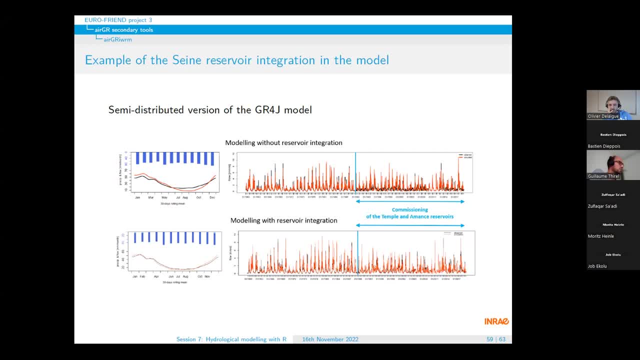 easily you overestimate floods and you underestimate, overestimate floods and you underestimate, overestimate floods and you underestimate low flows, low flows, low flows. because you don't take into account the, because you don't take into account the, because you don't take into account the reservoir. 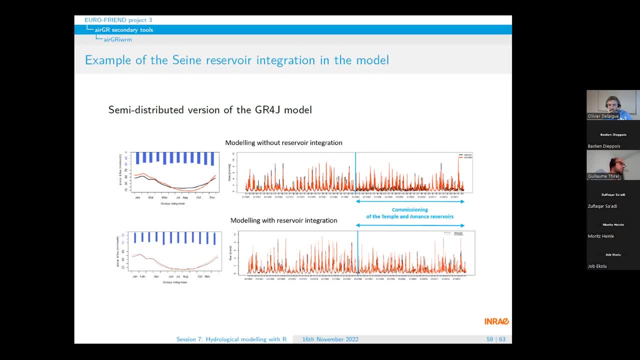 reservoir, reservoir, but if you use rgrw arm and take into. but if you use rgrw arm and take into, but if you use rgrw arm and take into account the reservoir account, the reservoir account, the reservoir which is the bottom part of the slide. 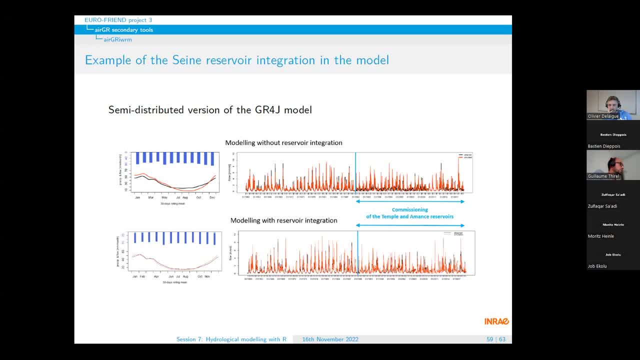 which is the bottom part of the slide, which is the bottom part of the slide. you see that, both, you see that, both you see that both regime, the discharge regime, but also the regime, the discharge regime, but also the regime, the discharge regime, but also the, the time series of stream flow simulated. 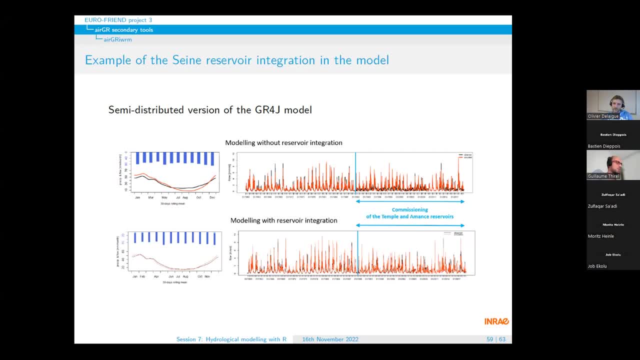 the time series of stream flow simulated, the time series of stream flow simulated after 1919 are very well after 1919, are very well after 1919, are very well represented. then we have a very, very new package, rgr. then we have a very, very new package rgr. 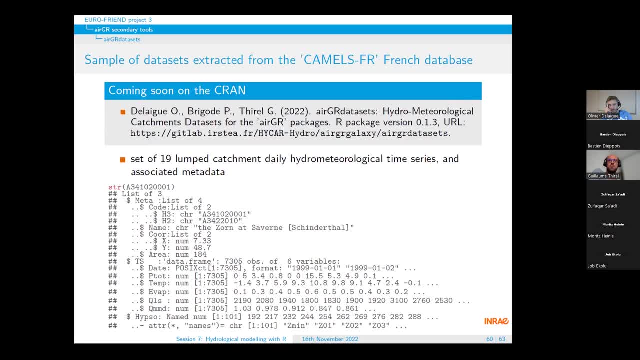 then we have a very, very new package- rgr- datasets, datasets, datasets, which is a package that, actually, which is a package that actually, which is a package that actually proposes a set of, proposes a set of, proposes a set of of data, of data, of data. so we, we proposed the 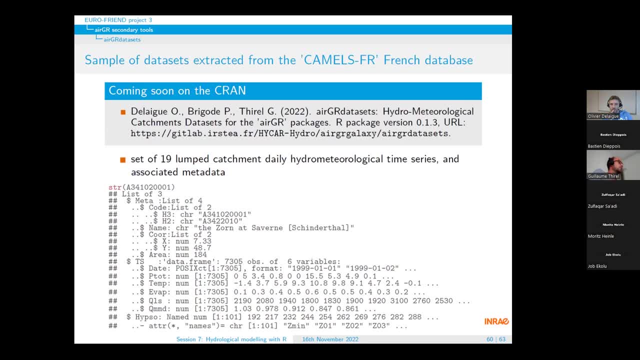 so we we proposed the. so we we proposed the. hydrometer meteorological data for 19. hydrometer meteorological data for 19. hydrometer meteorological data for 19. engagements in the loam in a lumped way. engagements in the loam in a lumped way. 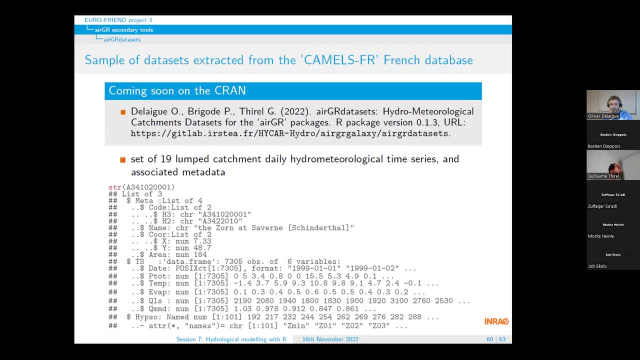 engagements in the loam in a lumped way, at a daily time step, and all the metadata at a daily time step and all the metadata at a daily time step and all the metadata, the metadata that you, you need to, the metadata that you, you need to. 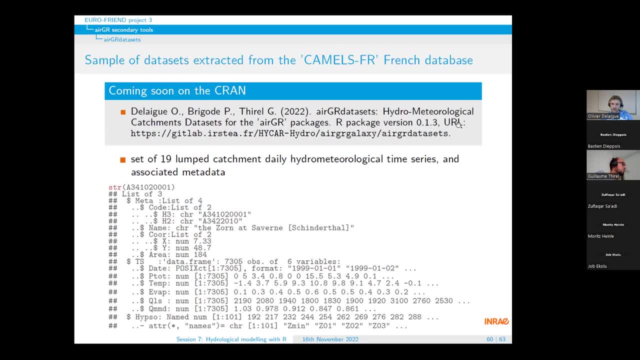 the metadata that you, you need to to make anything with that um, to make anything with that um, to make anything with that um. so you have precipitation temperature, so you have precipitation temperature, so you have precipitation temperature, potential depression and potential depression and potential depression and and discharge, mainly um. 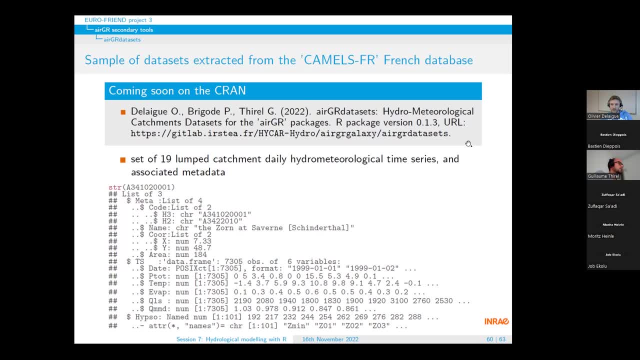 and discharge mainly um and discharge mainly um. so this is all available on the cron. so this is all available on the cron. so this is all available on the cron. actually, i think that it's not coming. actually, i think that it's not coming. actually, i think that it's not coming soon, but 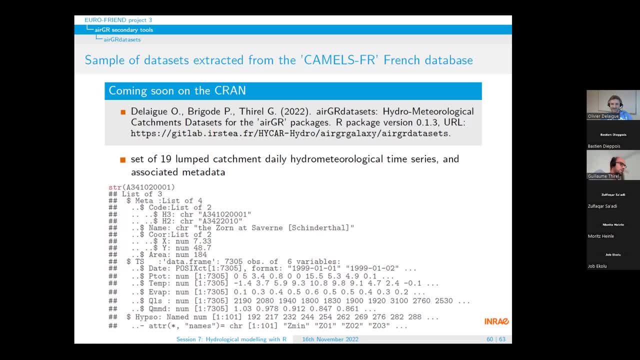 soon, but soon, but available for a couple of days now. available for a couple of days. now. available for a couple of days. now, we are very happy about that, we are very happy about that, we are very happy about that. and uh, yeah, if you want someone about the. 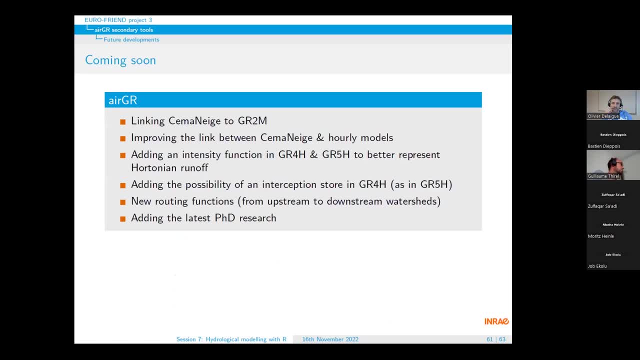 and uh yeah, if you want someone about the, and uh yeah, if you want someone about the future, future, future, development. we want to make with the development. we want to make with the development, we want to make with the different packages, different packages, different packages, things that we don't have yet, but almost 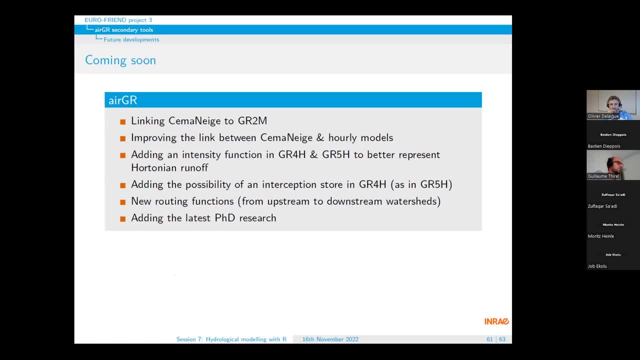 things that we don't have yet, but almost things that we don't have yet, but almost like, like, like. linking the snow model c-manage to the. linking the snow model c-manage to the. linking the snow model c-manage to the monthly gr2m model. 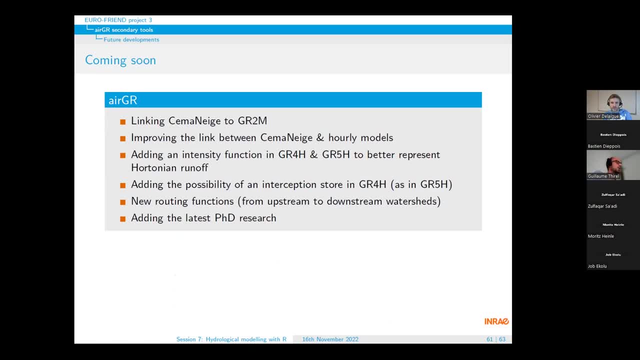 monthly gr2m model. monthly gr2m model. we also want to improve the link between. we also want to improve the link between: we also want to improve the link between the snow model and hourly models, because the snow model and hourly models, because the snow model and hourly models, because it's a very complex relationship. so we 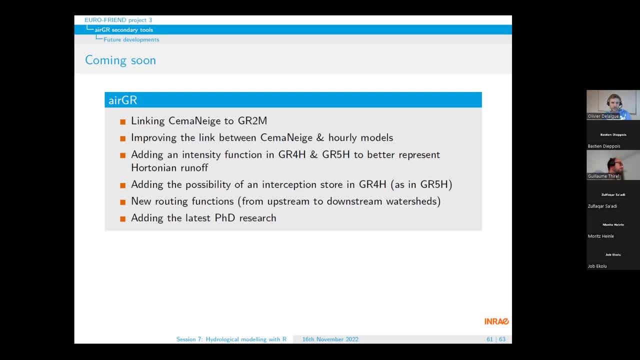 it's a very complex relationship, so we it's a very complex relationship, so we, we're working on that, we're working on that. we're working on that also for um, also for um, also for um flash floods, we flash floods, we flash floods. we have some phd works ongoing and almost 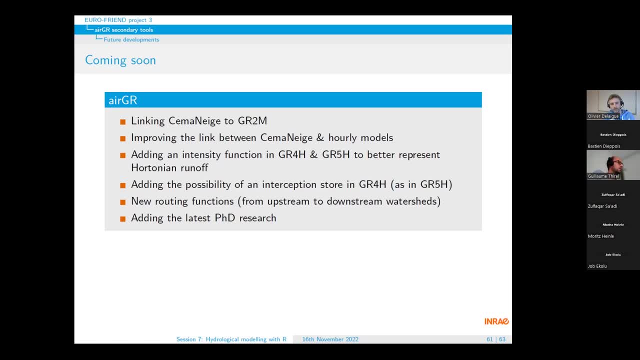 have some phd works ongoing and almost have some phd works ongoing and almost finished, finished, finished um to improve our hourly models uh in um to improve our hourly models uh in um to improve our hourly models uh in which they, which they, which they, the students, added some intensity. 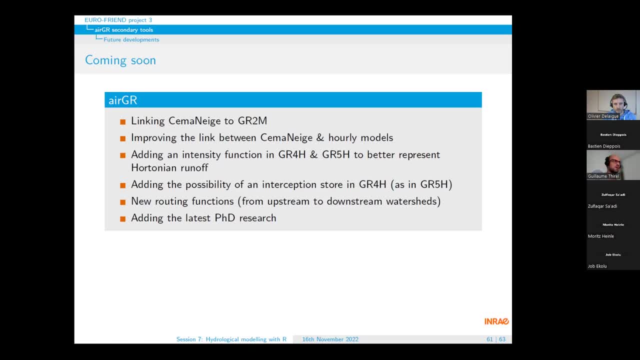 the students added some intensity. the students added some intensity, function to better represent a function. to better represent a function, to better represent a hartronian, hartronian, hartronian, runoff, runoff, runoff. we also have an intersection. turn gr5h. we also have an intersection, turn gr5h. 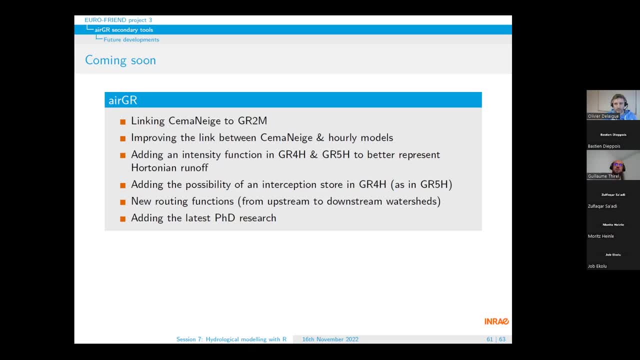 we also have an intersection turn gr5h. we want to add it in gr4h. we want to add it in gr4h. we want to add it in gr4h. very, very minor, very, very minor, very, very minor things, but things, but things. but that can be very useful. uh, regarding the 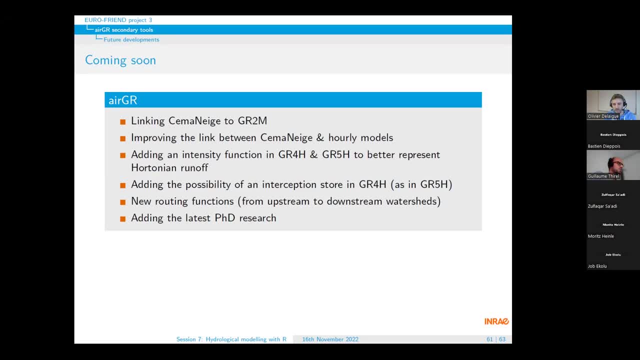 that can be very useful. uh, regarding the: that can be very useful. uh, regarding the routing, routing, routing functions. uh so the lag functions from functions. uh, so the lag functions from functions. uh, so the lag functions from upstream to dump stream. we want to. upstream to dump stream. we want to. 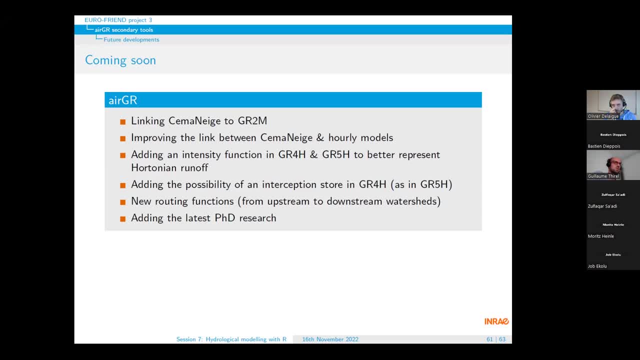 upstream to dump stream. we want to propose something else, propose something else. propose something else than the, than the simple lag that we, than the, than the simple lag that we, than the, than the simple lag that we have for the moment, have for the moment, have for the moment, uh and uh, yeah, we, we, it's ongoing- we, we. 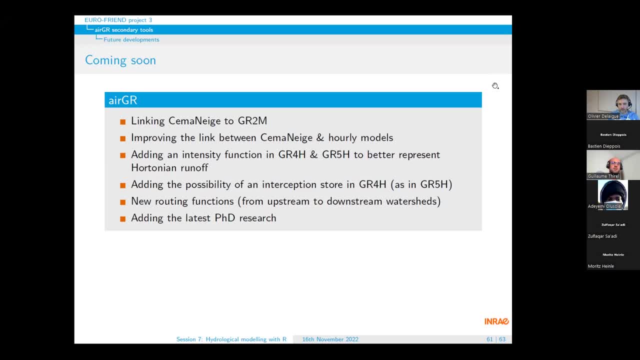 uh and uh. yeah, we, we, it's ongoing. we, we, uh and uh. yeah, we, we, it's ongoing, we, we want to continue to want to continue to want to continue to to, to add the phd research. so this was all in the rgr package. so this was all in the rgr package. 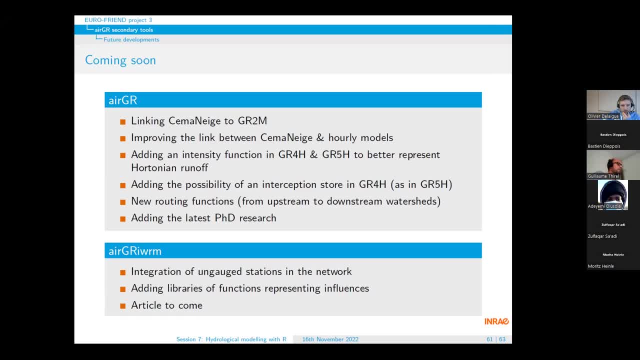 so this was all in the rgr package regarding rgrm. regarding rgrm, regarding rgrm, we recently integrated a. we recently integrated a. we recently integrated a way to way to way to: to use uh engaged stations in the net. to use uh engaged stations in the net. 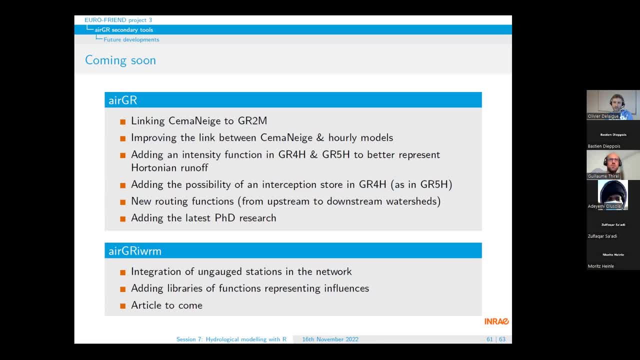 to use uh engaged stations in the net into the network, because uh the classical into the network, because uh the classical into the network, because uh the classical way to, way to way to to implement a semi-subject, to implement a semi-subject, to implement a semi-subject, semi-distributing models, is to 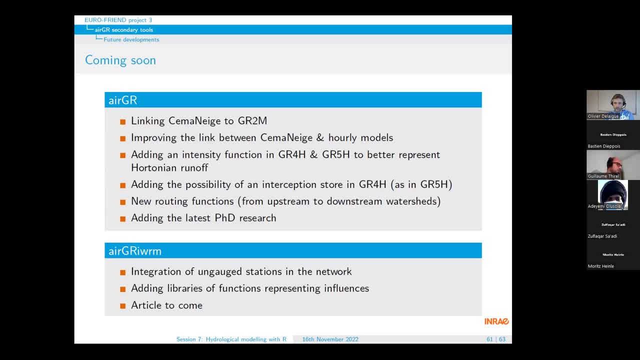 semi-distributing models is to. semi-distributing models is to to cut the basin on on points where you to cut the basin on on points where you to cut the basin on on points where you have have have observed discharge data, but sometimes you observed discharge data, but sometimes you 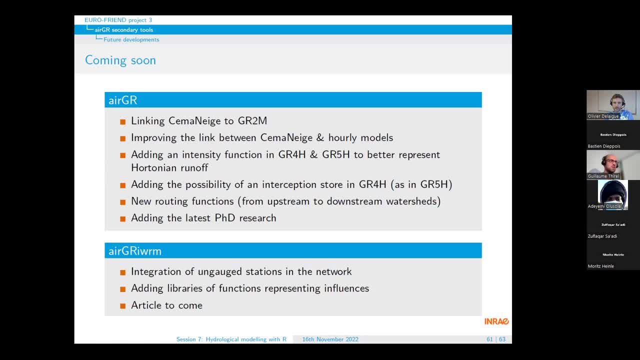 observed discharge data. but sometimes you have some interest, have some interest, have some interest within the catchments or sub catchments, within the catchments or sub catchments, within the catchments or sub catchments. so you want to do simulations, but for. so you want to do simulations, but for. 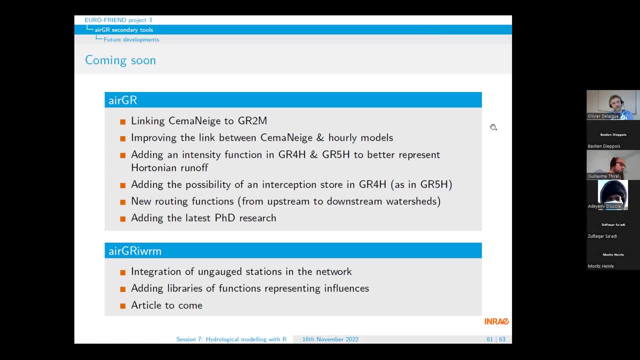 so you want to do simulations, but for this, you, you need a this, you, you need a this, you, you need a way to, to propose parameters to the way to, to propose parameters to the way to, to propose parameters to the model, model, model for, for this engage. 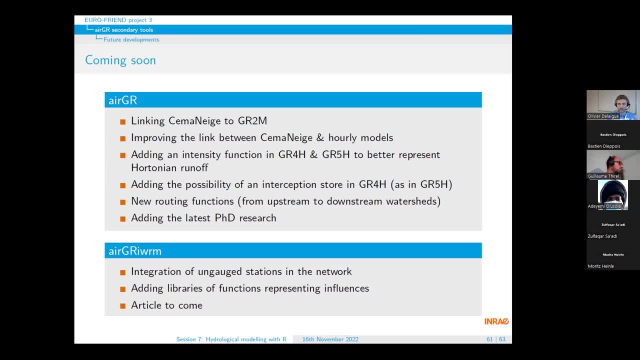 for for this, engage for for this: engage stations, sorry stations, sorry stations, sorry. we also want to provide libraries, or we also want to provide libraries, or we also want to provide libraries, or what we call vignettes, so this is a very. what we call vignettes, so this is a very. 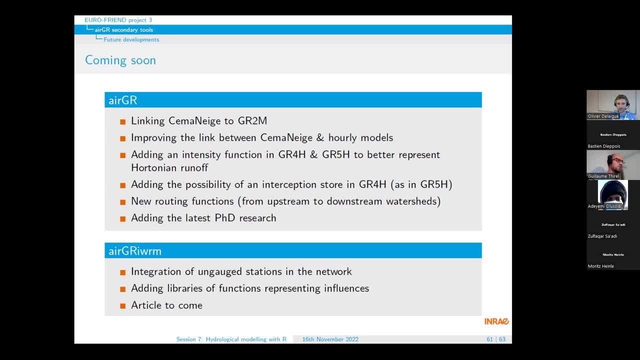 what we call vignettes. so this is a very complete description of functions, complete description of functions, complete description of functions to represent different type of, to represent different type of, to represent different type of influences. influences, influences, because when you, when you don't have the, because when you, when you don't have the, 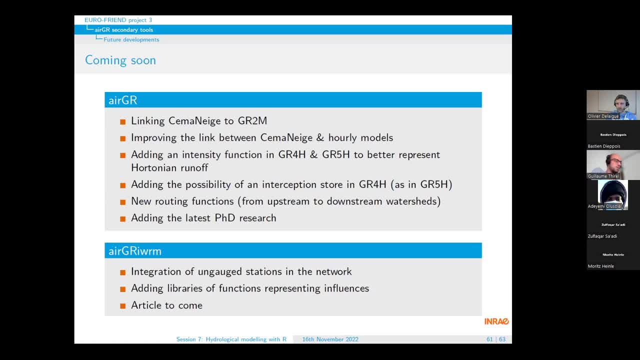 because when you, when you don't have the observed influence, observed influence, observed influence, data you, data, you, data you, you want to, you want to, you want to, to represent it, to represent it, to represent it, and also we, and also we, and also we. we are working on an article about this. 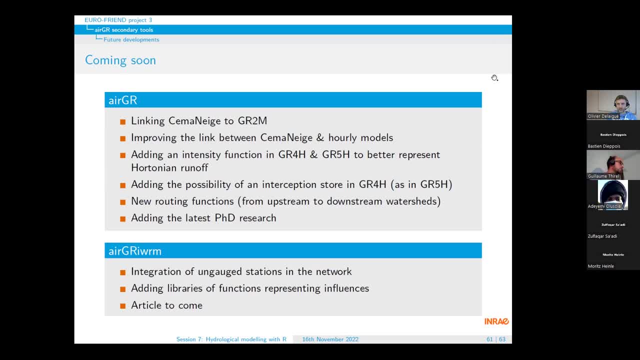 we are working on an article about this. we are working on an article about this package, package, package which will come soon may up, which will come soon, may up, which will come soon, may up, and and and, finally, as you're teaching, finally as you're teaching, finally, as you're teaching um. 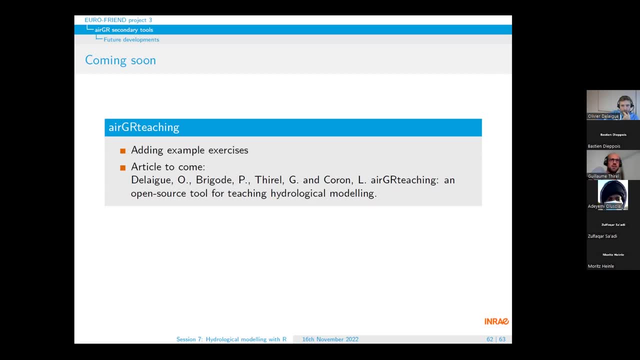 um, um, so, so. so, using the rgr data set, using the rgr data set, using the rgr data set, which proposes data for many catchments, which proposes data for many catchments, which proposes data for many catchments, we implemented, we implemented, we implemented in the, in the 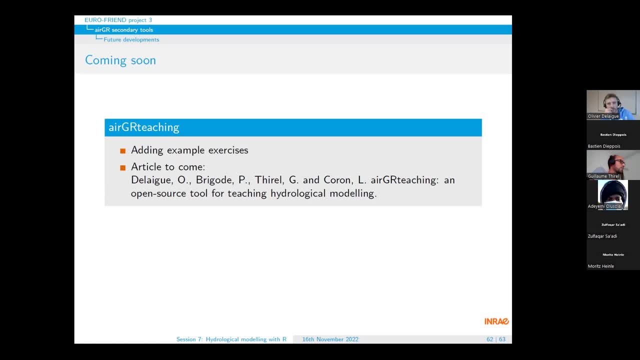 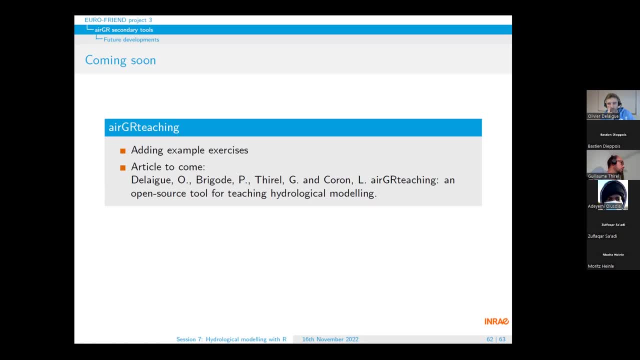 master project and so on, master project and so on. so this will come, so this will come. so this will come very, very, very soon and soon and soon. and what will come also very soon? i think it, what will come also very soon. i think it, what will come also very soon, i think it can be. 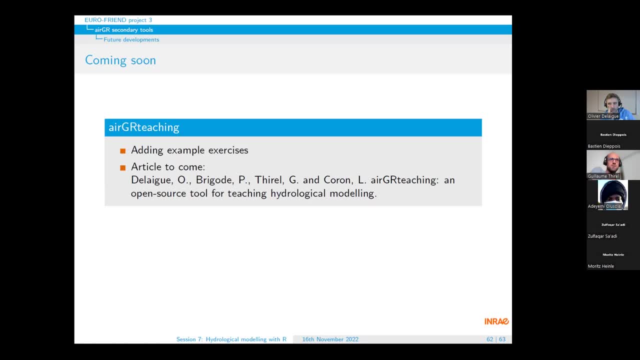 can be. can be submitted in the next uh before the. submitted in the next uh before the. submitted in the next uh before the before the end of the month. before the end of the month before the end of the month is an article describing both. is an article describing both. 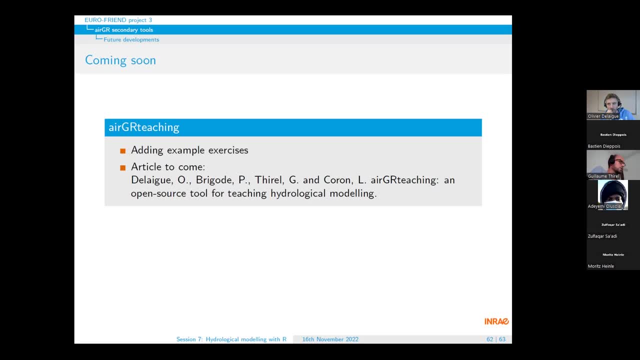 is an article describing both the use and the: the use and the. the use and the content of the rgr teaching package. but content of the rgr teaching package. but content of the rgr teaching package. but also also also describing some very general modeling. describing some very general modeling. 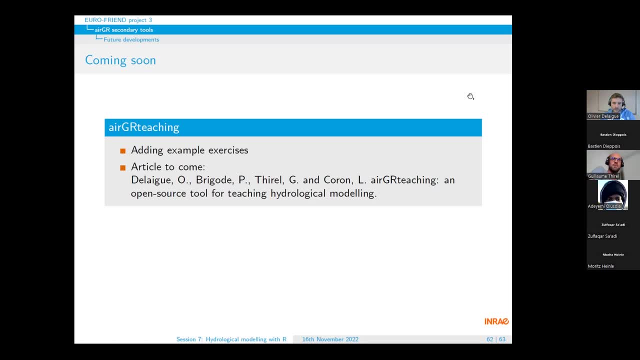 describing some very general modeling, hydrological modeling exercises, but also hydrological modeling exercises, but also hydrological modeling exercises, but also some very specific exercises that can be used for teaching, exercises that can be used for teaching exercises that can be used for teaching. and uh and uh.